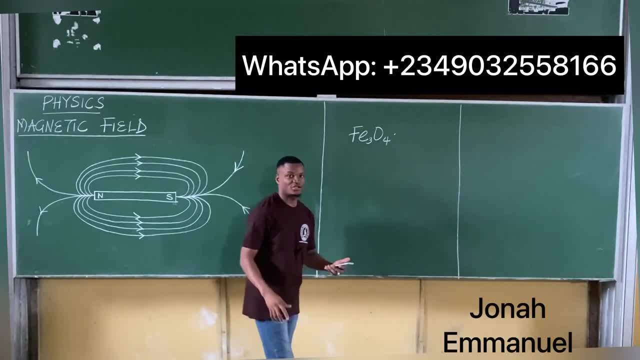 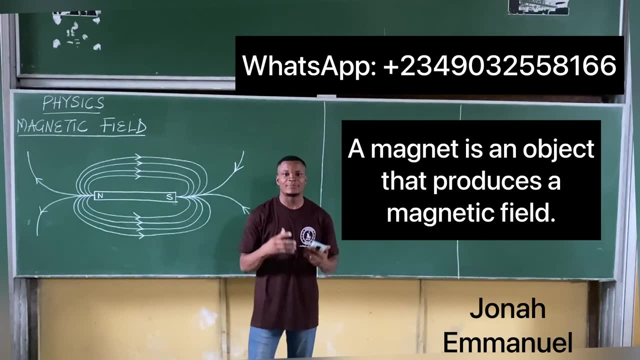 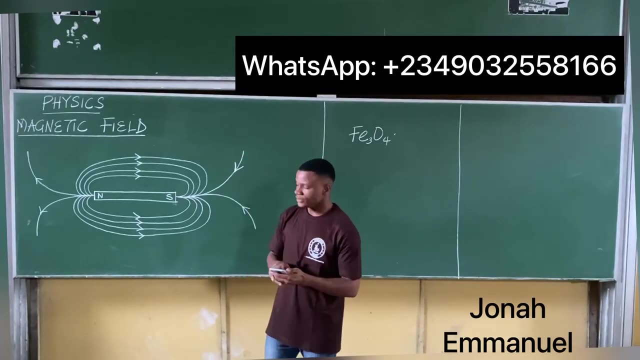 So you have three atoms of iron and four atoms of oxygen. that constitutes a magnet. Now, what's a magnet? By definition, a magnet is simply an object that produces a magnetic field. That's a magnet, All right. so, having said so, let's look at magnetic field properties. 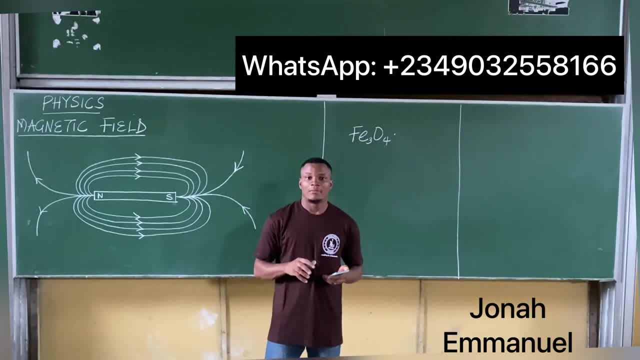 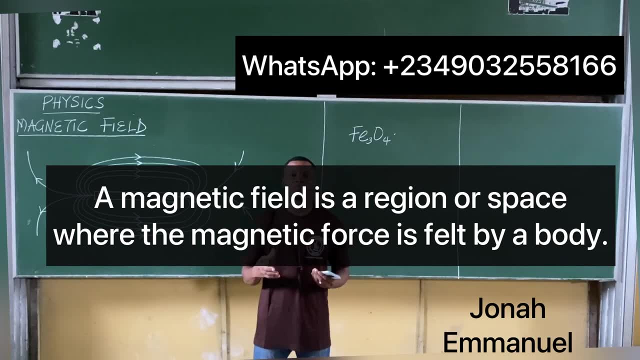 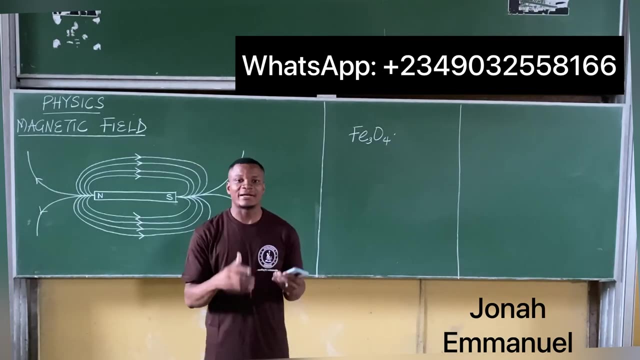 So, for example, magnetic field can be defined as a region or space where the magnetic force is felt by a body. That's the definition, all right. A magnetic field is simply a region or space where the magnetic force is being felt by a body. That's your definition for the magnetic field. 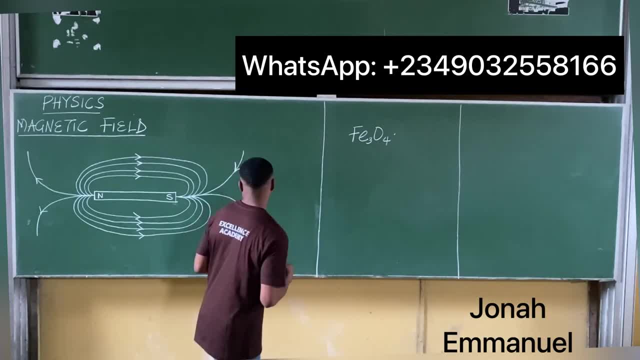 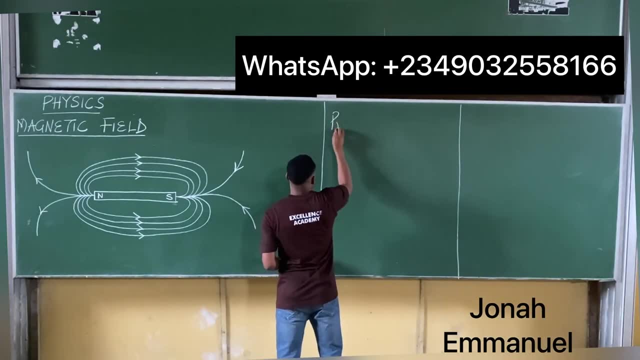 Now, when it comes to, let's look at how to produce a magnetic field. Let's look at how to produce a magnetic field. Let's look at how to produce a romantic field. Let's look at production of magnetic field. So, production of magnetic field. 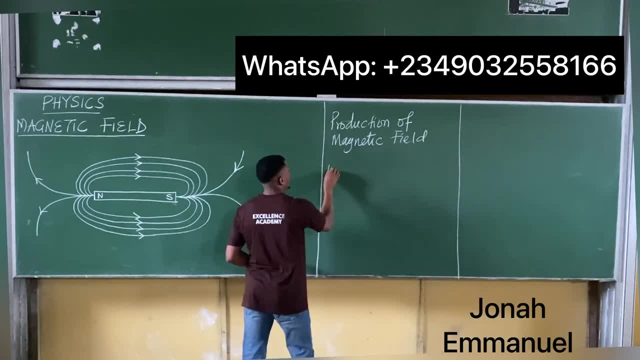 All right. So the first way of producing magnetic field is simply through the motion of electric charges. All right, This is through the motion of electrical charges. So when electrical charges move, they produce a magnetic field. That's the first one. 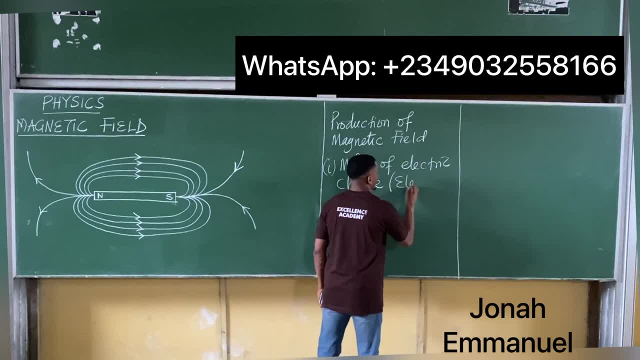 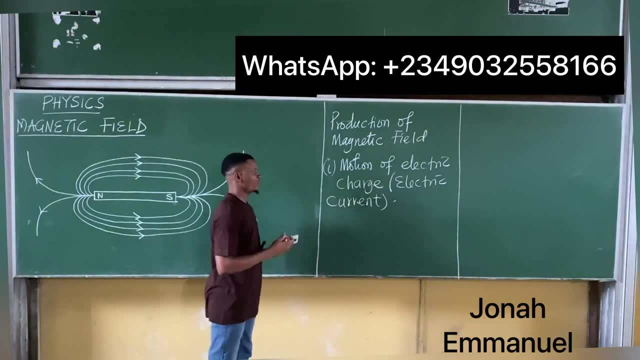 Or some would say They call it electrical currents. Some term this electric currents, Some term it electrical currents. So of course, electrical currents is simply the movement of electrical charges. So they are the same thing. The second way of producing magnetic field is through the use of a magnet. 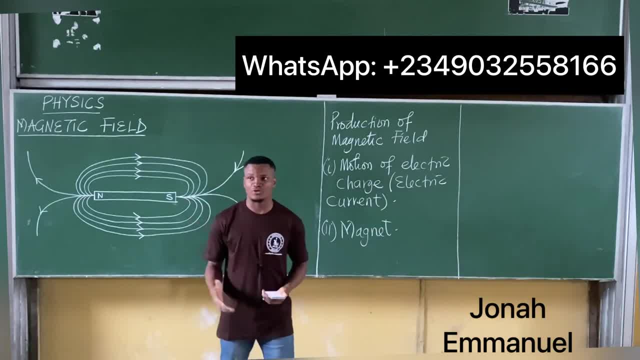 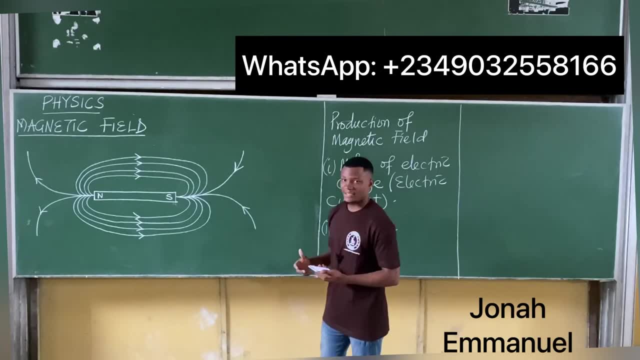 So the use of a magnet can be used. Or a magnet can be used to produce electrical field. All right, The electrical field produced by a barbed magnet is given here. So this is the diagram for the All right. So the magnetic field produced by a barbed magnet is given here. 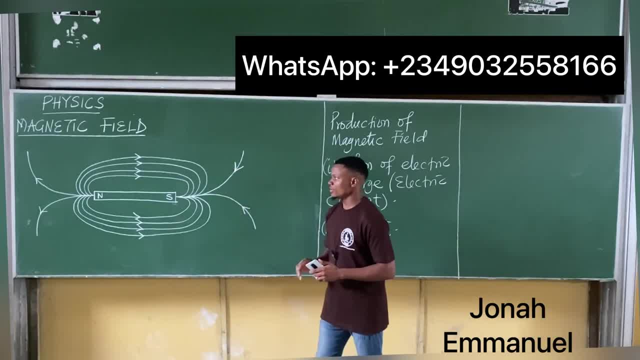 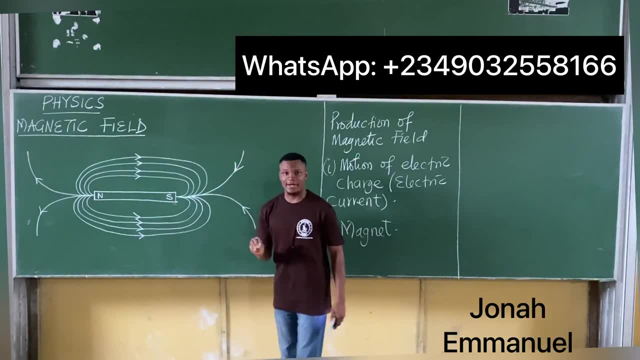 So this is a diagram that shows the magnetic field produced by a barbed magnet. So you can see the north pole, You can see the south pole. The key take here in this diagram is: The key take here in this diagram is: 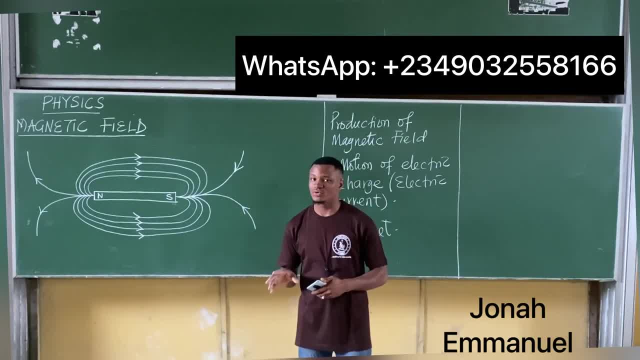 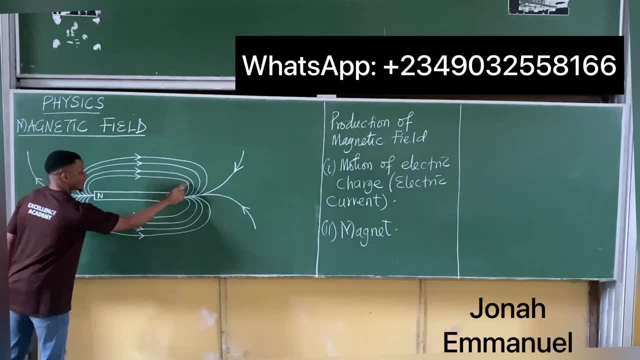 The magnetic field flows from the north pole to the south pole, Very important. So observe my diagram. Observe that the direction of motion is from north pole to south pole, From north pole to south pole, From north pole to south pole. 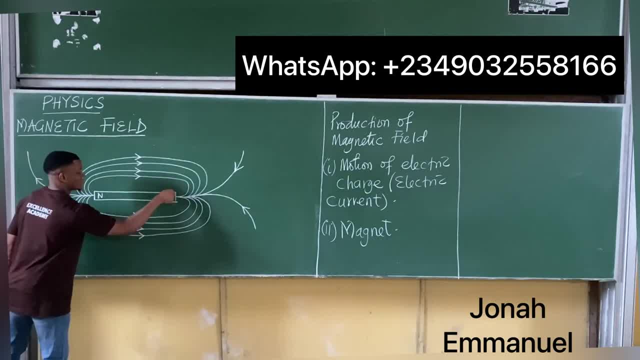 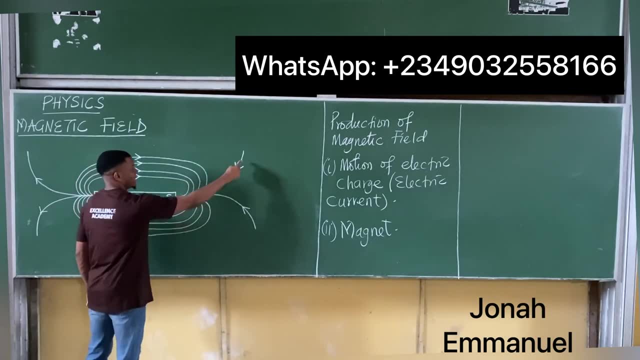 Same thing down here. Movement direction is from north pole to south, The north pole to south, The north pole to south And E to C. Even in this instance here, observe that for this one here it's flowing into the south pole. 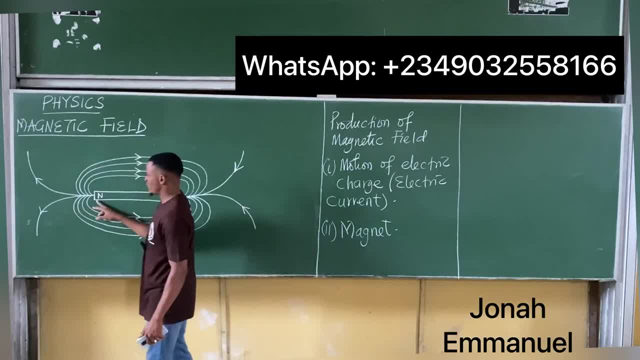 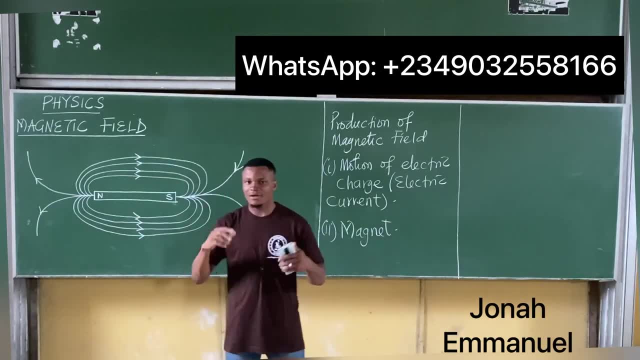 This direction too, Flowing into This direction too. the south pole for the north pole. now observe that it is leaving the north pole and also leaving the north pole. so, for your magnetic field, the direction of motion is that, if the magnetic field flows out, 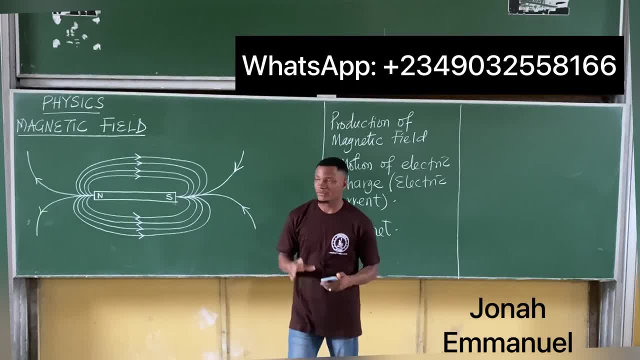 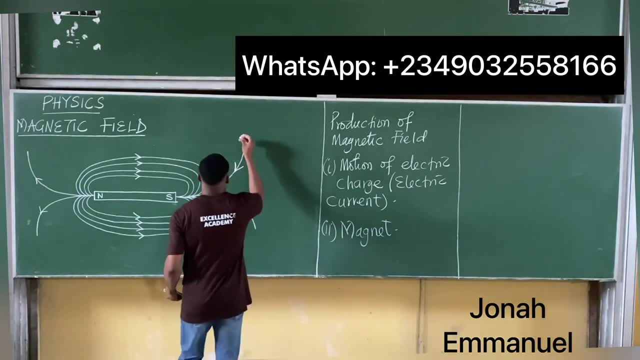 from the north pole and into the south pole, very important. now we talked about pole, pole, pole, pole, pole. what's a pole? if i have a bar magnet like this? so i have a magnet like this. a magnet has two poles. the two poles of a bar, of a bar magnet is simply, or are, the north pole and the south. 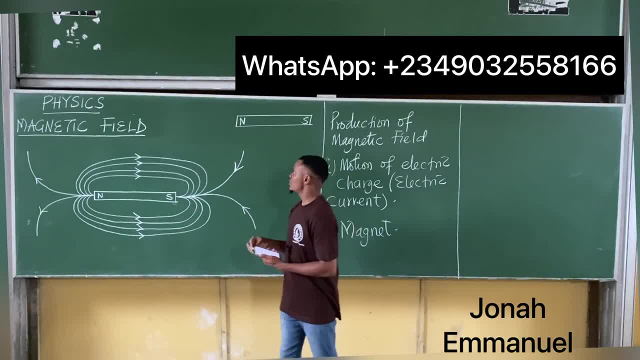 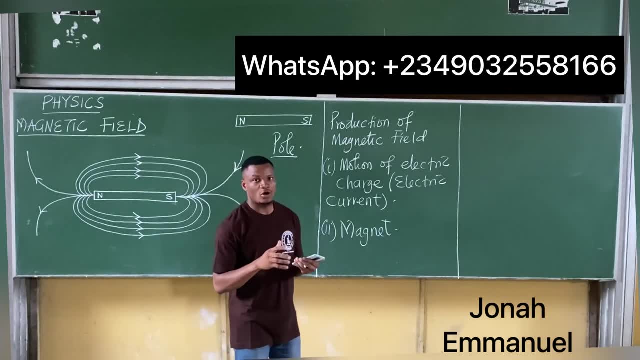 so these are the two poles of a magnet. what's a pole? that's the question. what's a pole? pole p-o-l-e is simply the region of a magnet where the magnetic field is being produced or the magnetic force is being produced. that's how we define a pole. so the pole of a magnet is simply. 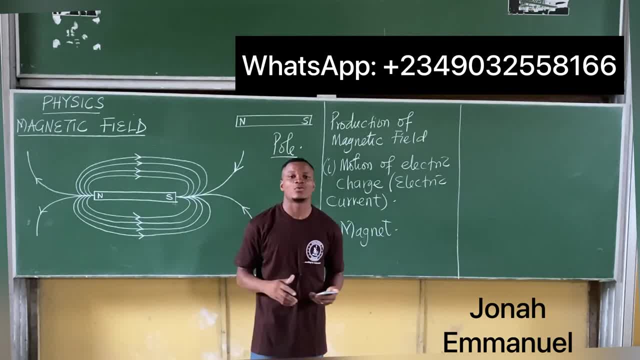 that direction region of a bar magnet or a magnet where the force of a magnetic field is being felt the most or being produced. this is how we define a magnetic pole. Now let's move on again. as earlier noted, we said, current flowing through a wire produces. 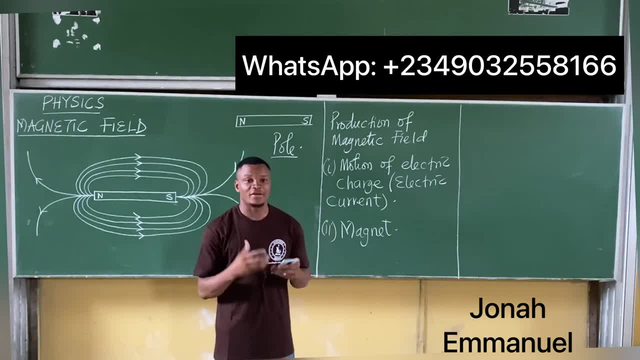 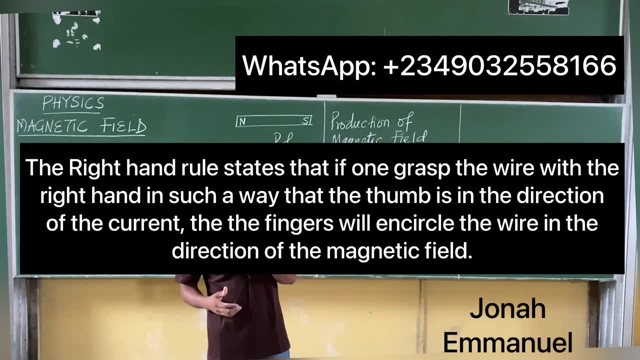 electric fields. the direction of this electric field can be remembered using the right hand rule. using the right hand rule. now, what's the right hand rule? The right hand rule states that if one grasps the wire with the right hand in such a way, 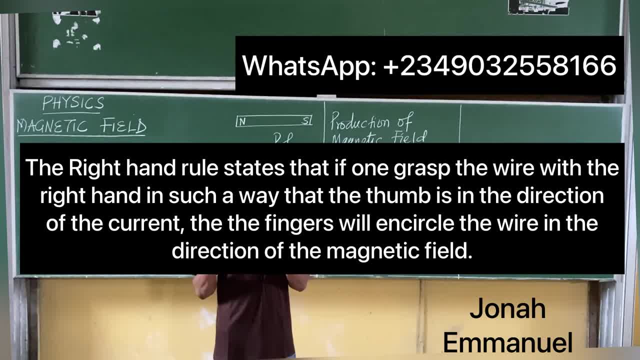 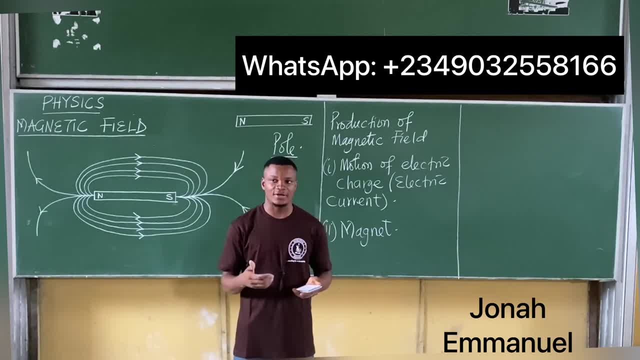 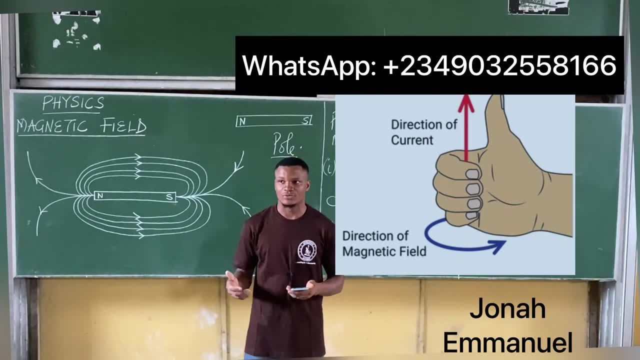 that the thumb is in the direction of the current, then the fingers will encircle the wire in the direction of the magnetic field, as you can see here. alright, so this is your diagram that explains, or that shows you your right hand rule. so that's it. alright, let's. 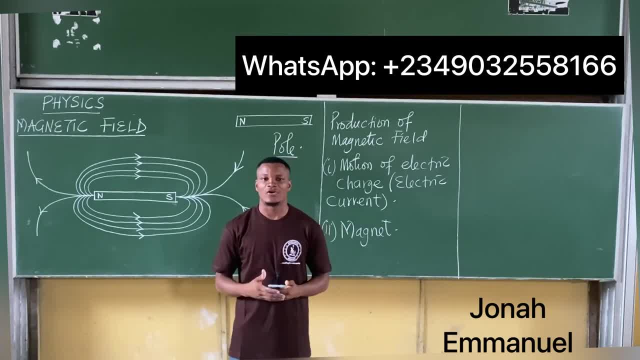 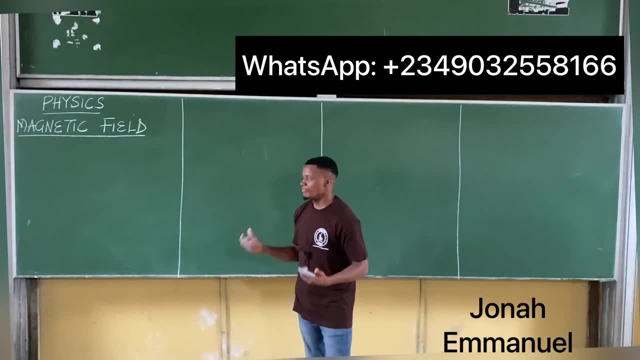 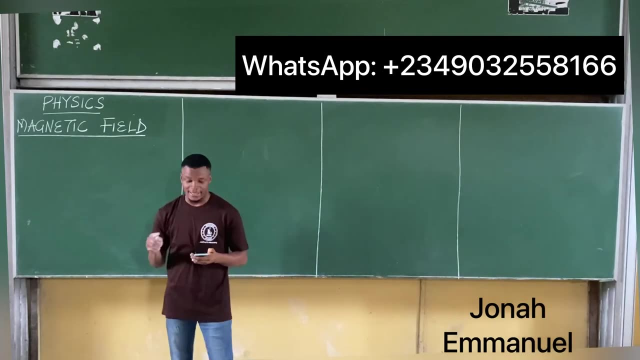 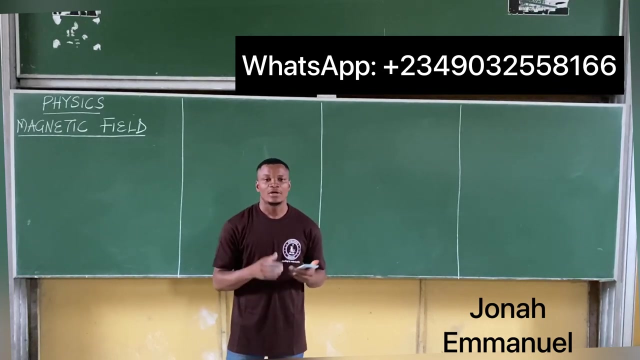 move on now. So let's now go to the calculative part of magnetic field. alright, so let's try some calculations involving magnetic field. now here are two things to note. number one: note that, given a conductor of length L carrying current I and inclined at an angle theta to 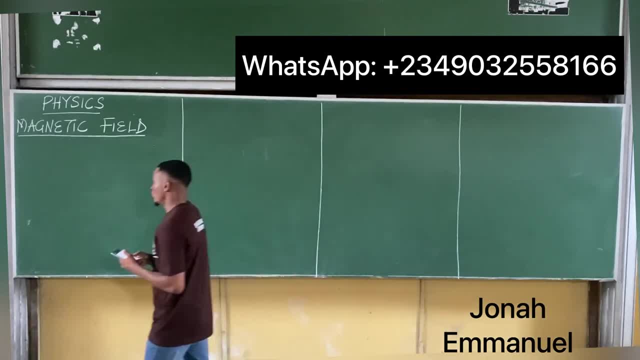 a magnetic field B, as shown below. So let's say I have a magnetic field B. So let's say I have a magnetic field like this, this, this, this 4 and 5, let's call this a magnetic field. so I'm showing the direction of motion as this. let's say I have 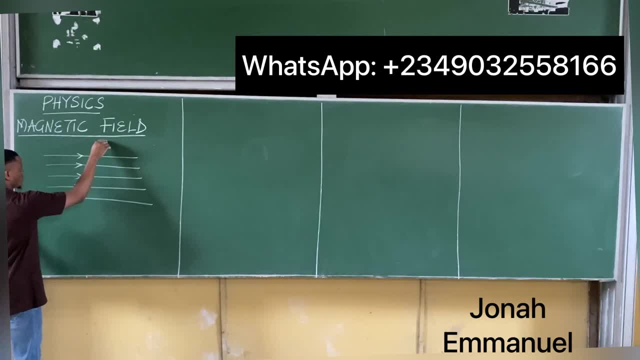 a conductor carrying current, let's say, a conductor like this, like this, so this is a conductor. alright, so I have a conductor in a magnetic field, such that this is a magnetic field, So this is a conductor. Now, this conductor is inclined to the magnetic field at an angle, this, let me call this angle. 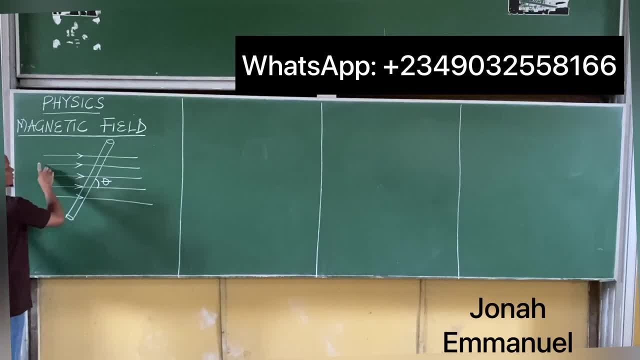 theta or theta here. let's call this magnetic field B, such that length of conductor, from this point up to this point, length of conductor is called L. okay, let me bring this down instead. so I'm bringing this length down instead. so, from this point to this point, let's call: 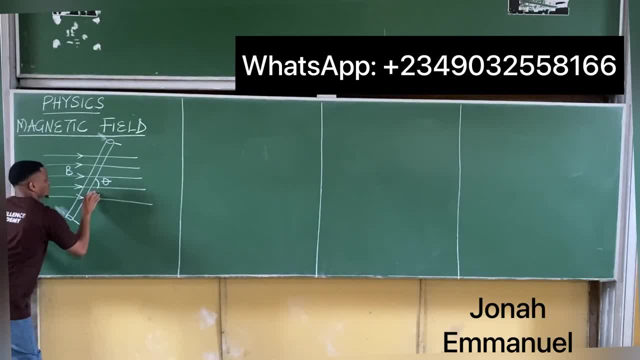 that length. So I'll call this L. Alright, so I have a conductor of length L carrying current, so this conductor has current I inside. so I'm saying that, given a conductor of length L carrying current I, inclined at an angle theta to a magnetic field B, then we have that, the force, the force. 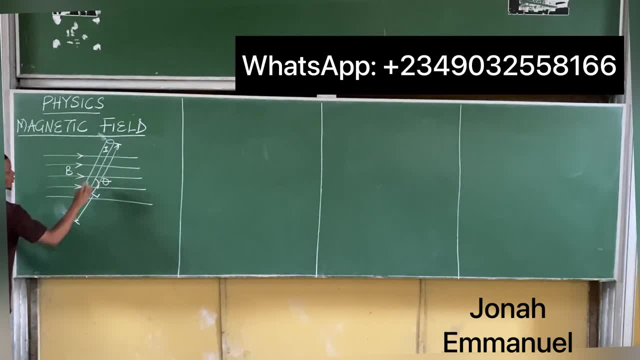 the force on the magnetic field is B. Okay, Okay, So the force on this conductor carrying this current is given by F, and F is equal to ILB, sine of theta, Please. this is a very important formula in magnetic field, that the force on the conductor 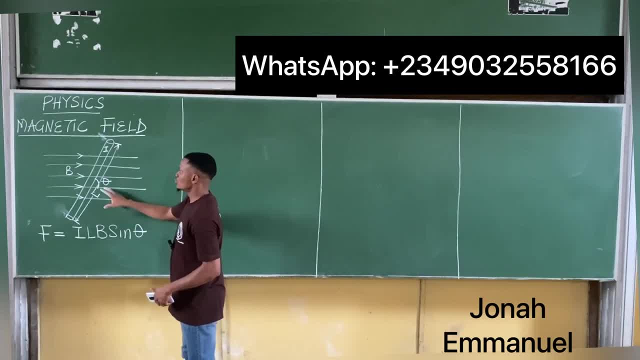 carrying current inclined at an angle theta to a magnetic field is given by F equal to ILB sine theta. Okay, So F is simply force on current. so F is equal to force on conductor conductor carrying current. carrying current I is equal to simply the current carried by the conductor, of course. 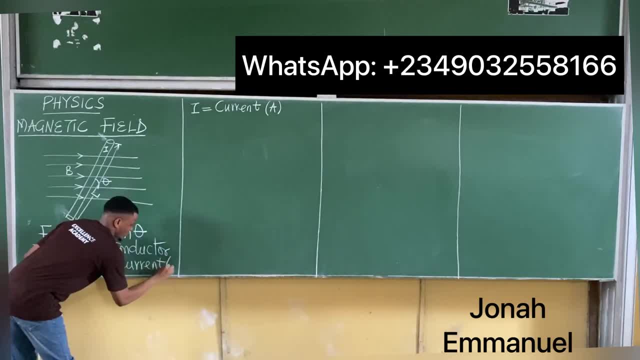 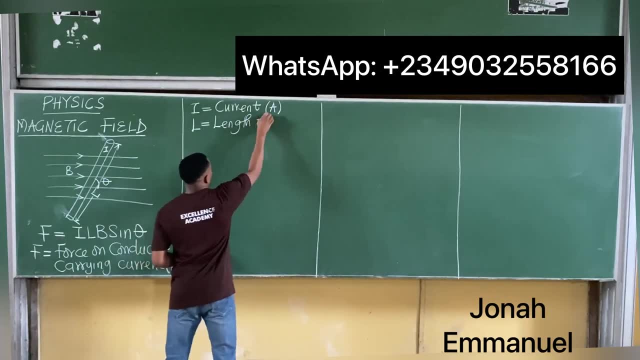 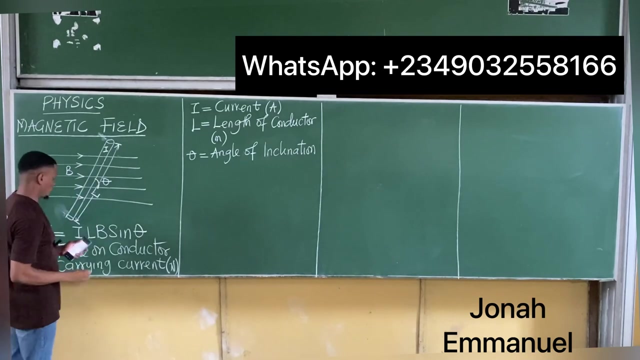 in amperes A, the force obviously is in Newton and L is the length of the conductor. so length of conductor, that's in meters. theta is the angle of inclination, angle of inclination of the conductor to the magnetic field and B is equal to magnetic field. 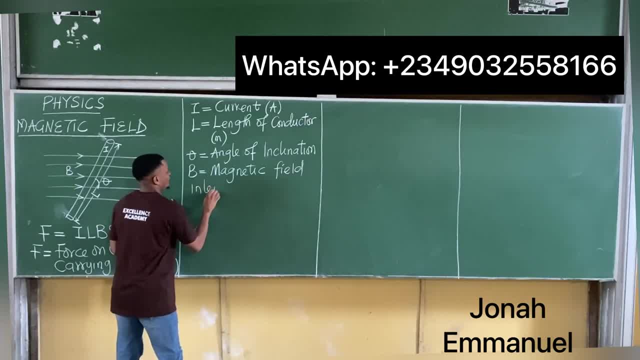 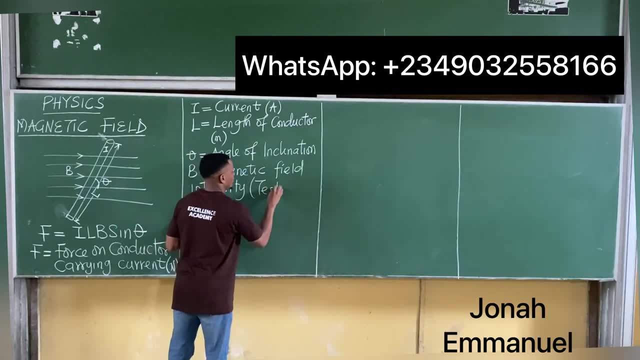 It's called the magnetic field intensity. Like I said, magnetic field or magnetic field intensity, and this man is measured in Tesla, So that's the SI unit, or magnetic field. So these are like what you have here, Okay, Okay. 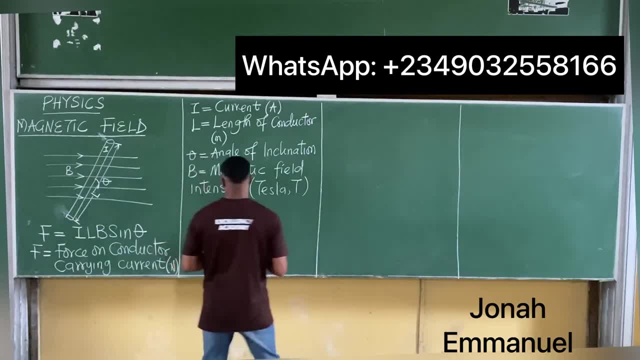 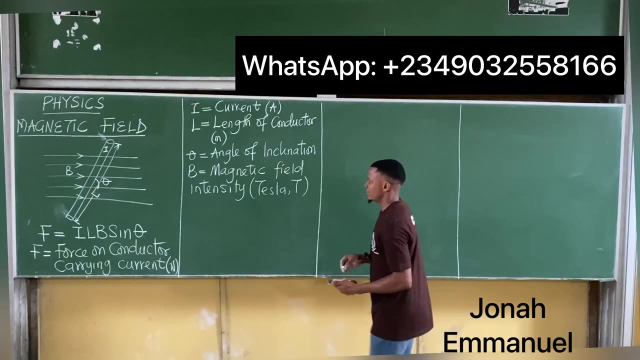 Okay, Okay. Now it is important to note that the maximum force that is expressed by the conductor in the magnetic field would occur when the conductor is perpendicular to the magnetic field. So we are saying that maximum force, we are saying this, we are saying that the maximum 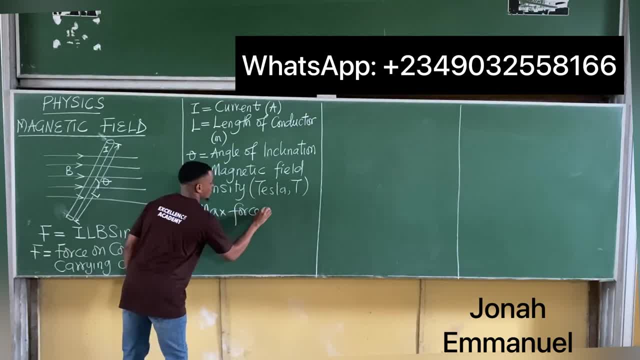 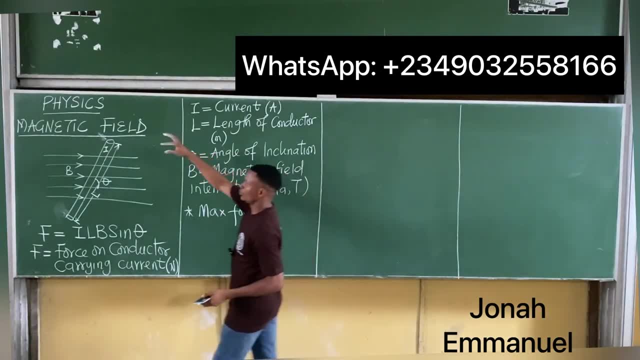 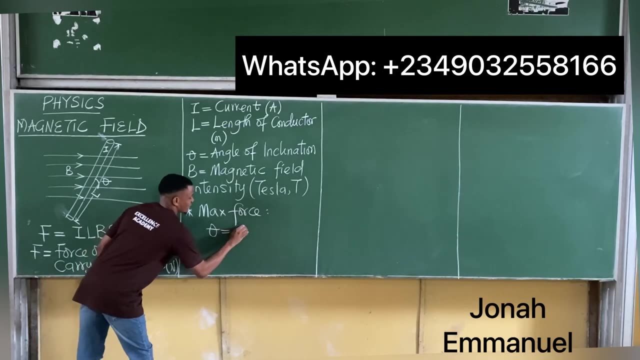 force, maximum force experienced by a conductor in a magnetic field occurs when the angle, theta, or when the conductor itself is far away. Okay, conductor is perpendicular to the magnetic field. that means theta will be equal to 90 degrees. all right, if that's so, i will substitute this condition into my formula. so i'll now have that. 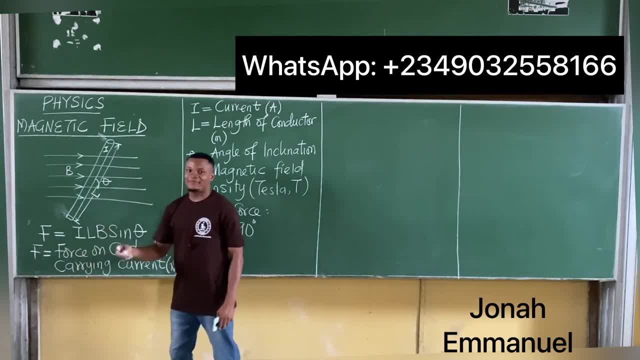 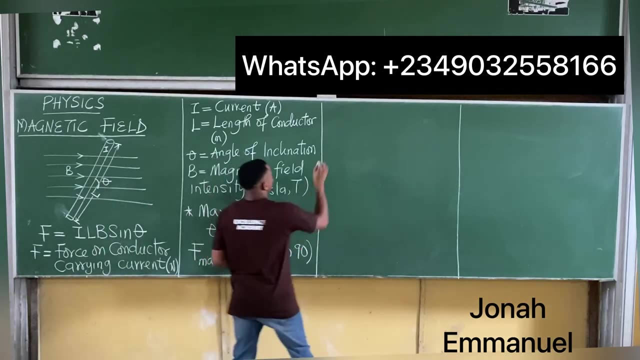 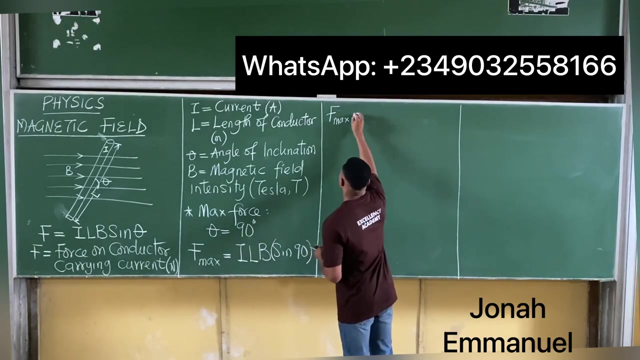 f, now no longer f but f maximum. so maximum force, f max, is equal to ilb sine 90. so i have this. so if this is true, i'll have that the maximum force experienced by a magnetic um but expressed by a conductor in a magnetic field is equal to ilb. 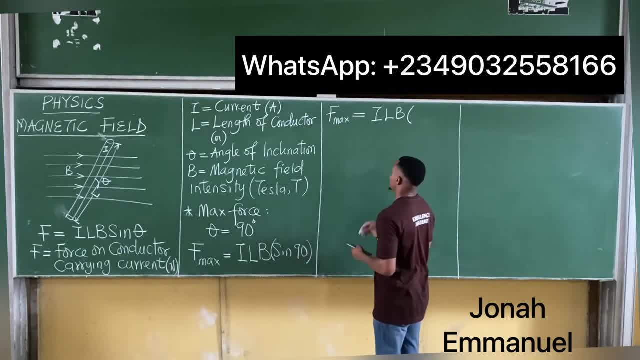 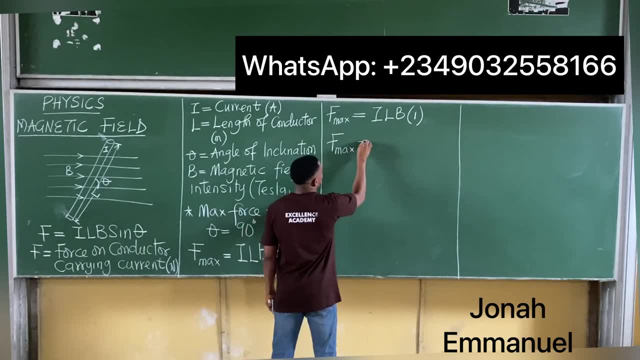 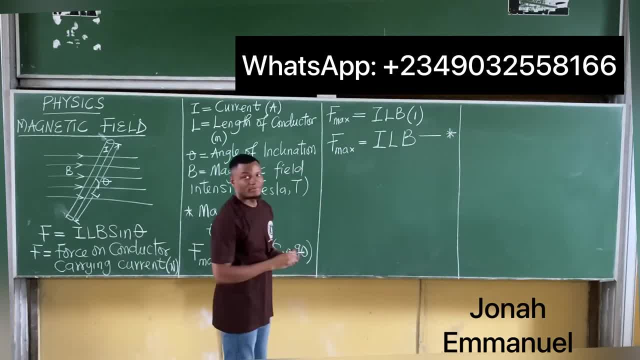 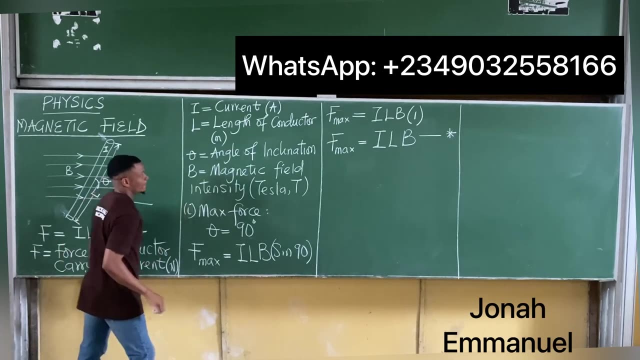 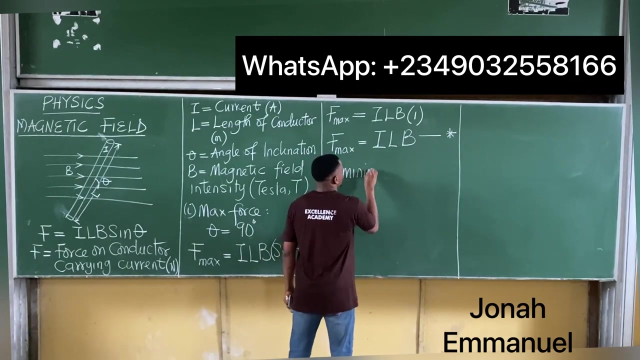 This is a very important formula in magnetism or magnetic field calculation. So if this is the maximum force, what about the least force, The minimum force? so let's call this one, let's call this I, let's call this II for II, the minimum force. if you look at maximum force, let's look at minimum force. 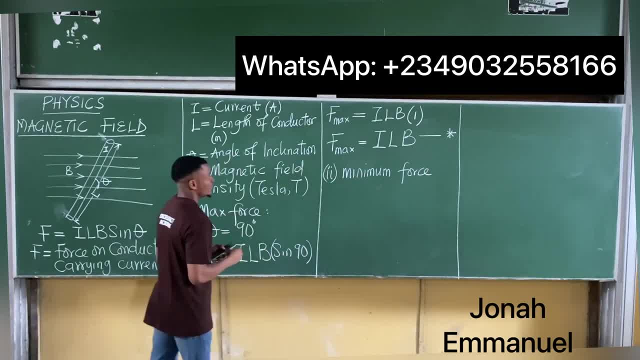 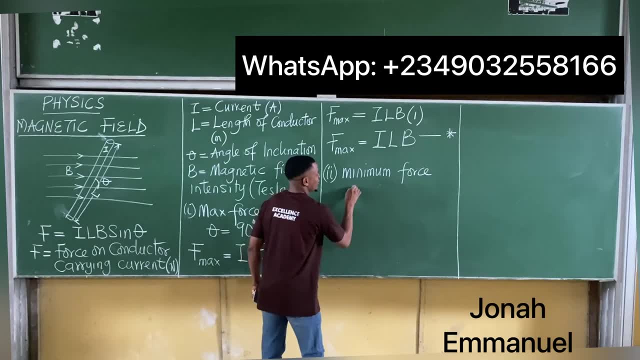 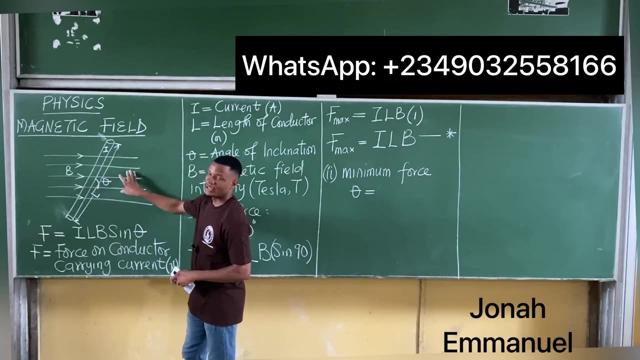 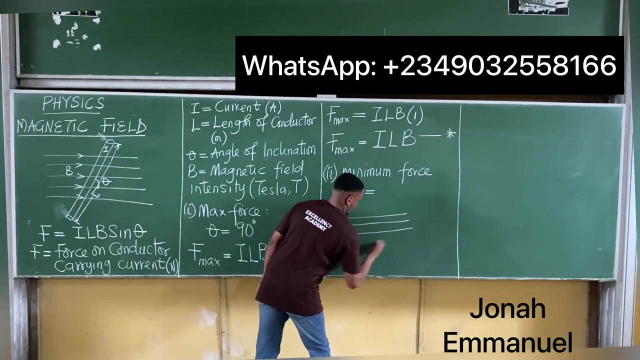 The minimum force that we experience by a conductor carrying current in a magnetic field Occurs when the conductor is parallel, when the conductor is parallel to the magnetic field, and by parallel will mean if I'm having the magnetic field as this, then by parallel will mean that the conductor will place this way, so we'll have a conductor this way at this point now, the conductor is now parallel to the magnetic field. 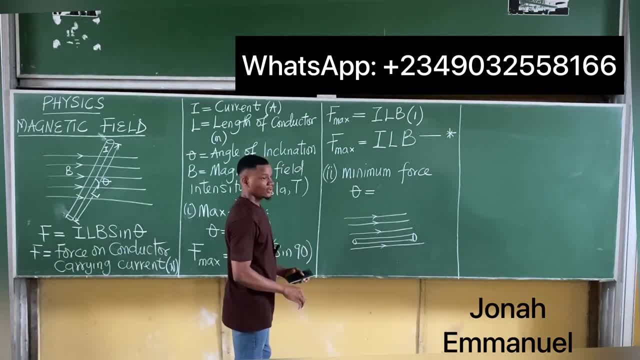 So here's my conductor, here's my field. It's now parallel to the field. If the conductor is parallel to the magnetic field, that means the angle between them is nothing, so hence the zero. So please take note that minimum force occurs when theta is zero. 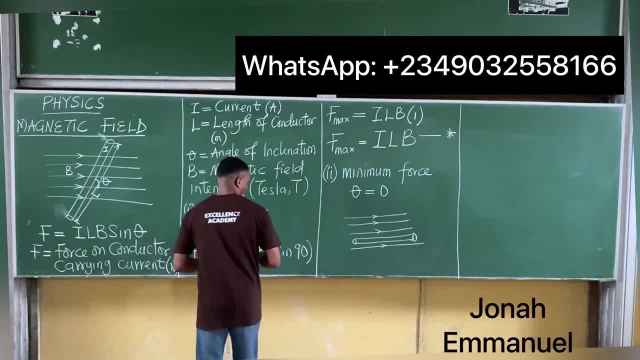 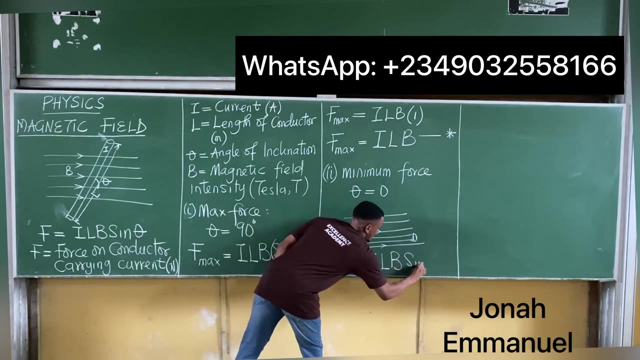 So if I substitute this condition into this formula, I'll have that F minimum, F no longer F, but F minimum. so minimum force is equal to ILB sine theta is zero. I'm having ILB sine Sine zero. 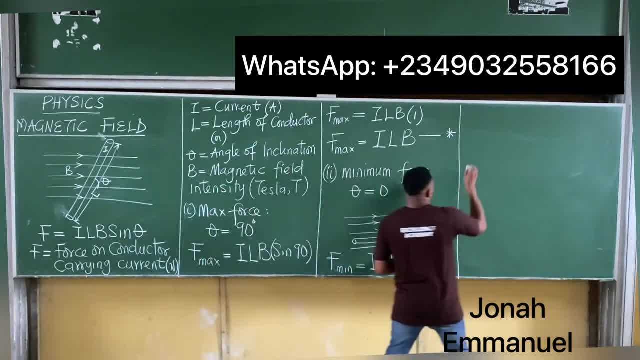 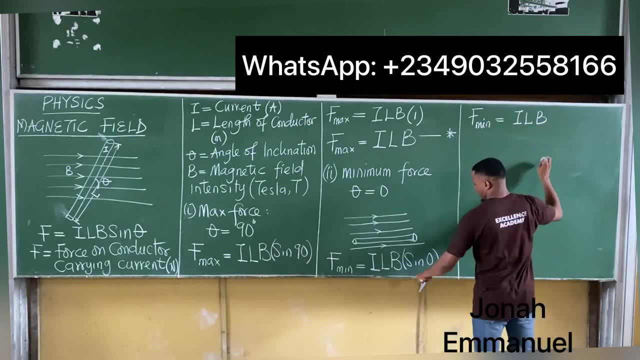 So I have this: If I work on this, I'll have that F minimum and the minimum force is equal to ILB. sine zero gives you zero. That means the minimum force, F minimum is equal to this time. zero is zero. 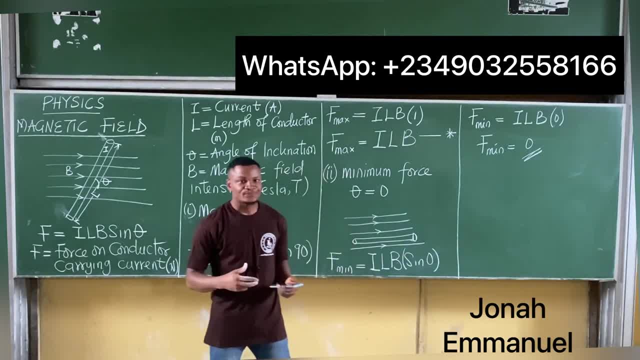 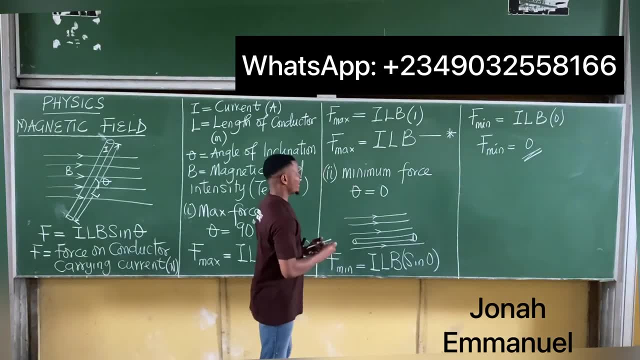 So the minimum force experienced by a conductor in a magnetic field is zero. Why? Because the minimum force is given by the formula ILB. Alright, so note that what you have here is actually: or. this formula here is actually the scalar form of this formula. 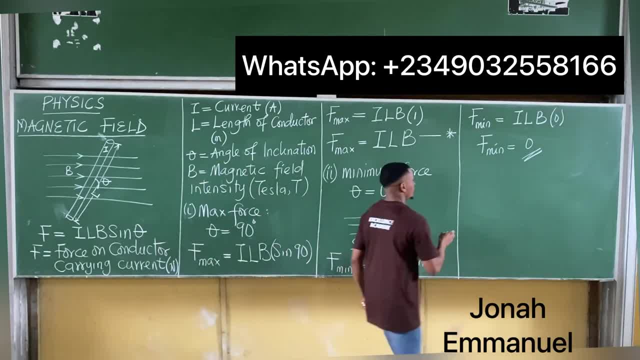 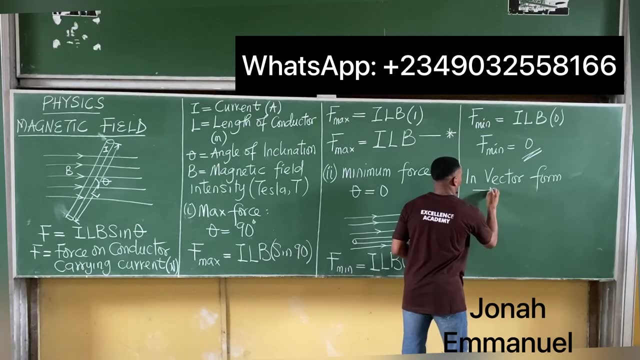 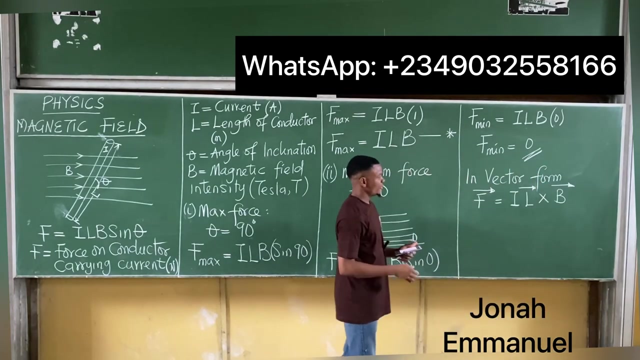 What you have here is the scalar form In vector form. in vector form this formula here can be rewritten as saying so. in vector form we'll have that F, It is equal to IL cross B. So here is a vector form representation of this formula. 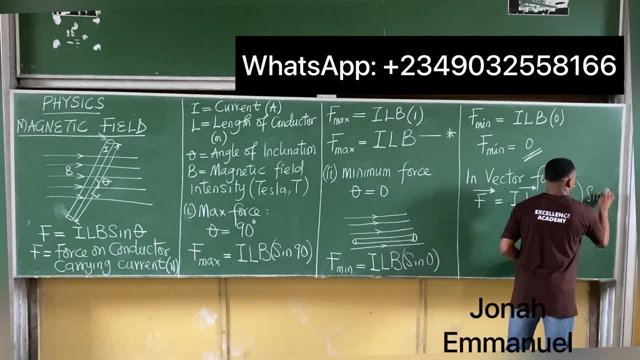 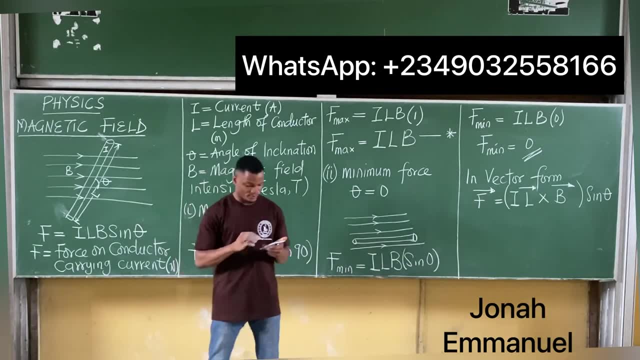 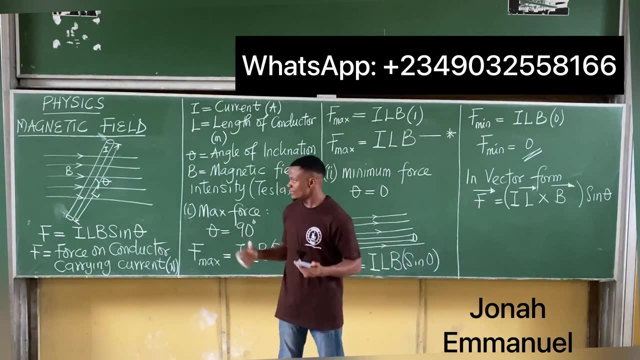 If you want, you can see: add sine theta, So this, sine theta, So this is a vector form representation of this formula. Alright, let's move on. Let's look at the second concept. So this is like the first idea or concept when it comes to making a calculation on magnetic. 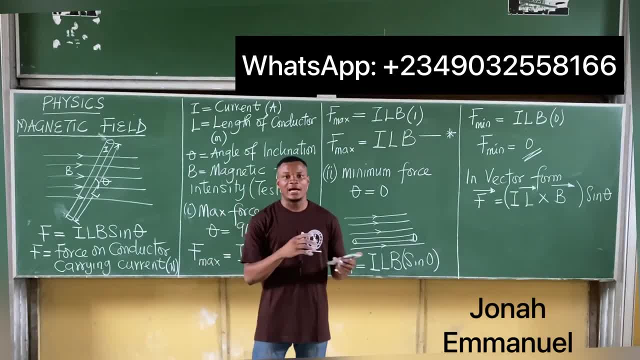 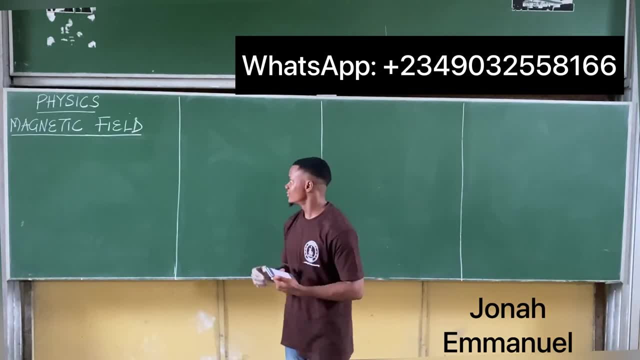 field. Let's look at the second concept, involving electrical charges placed in a magnetic field. So let's look at the second concept about magnetic fields or magnetic field calculation. So for this concept, we're looking at the magnetic force on an electrical charge placed. 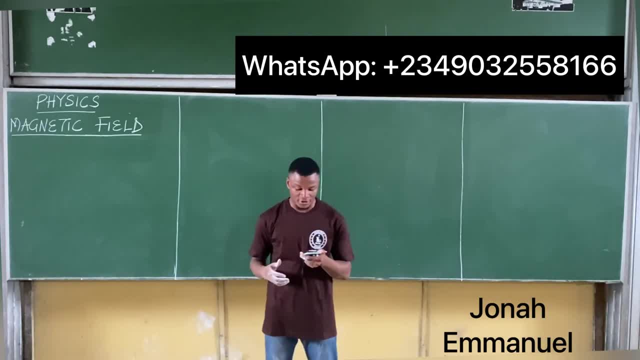 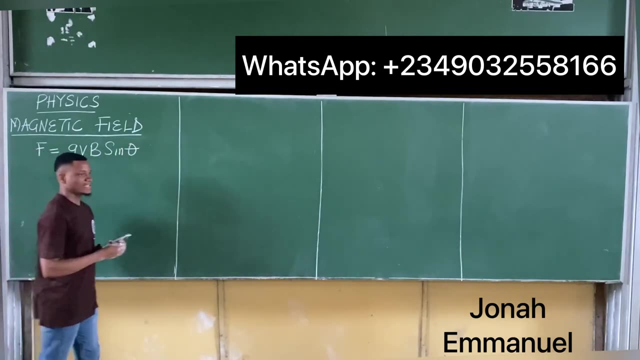 in a magnetic field. Now note that the force on a moving electrical charge in a magnetic field is given by the formula F, equal to QVB, sine theta. That's your formula there. In vector form this becomes F. F equal to QV, cross B, and then sine theta, if you want to. 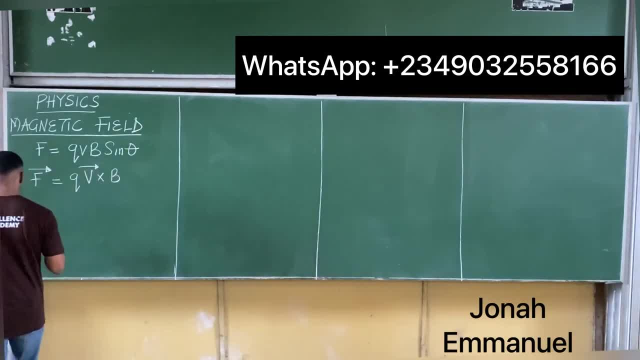 So I have this one here where F- let's define this- where F is equal to the force on moving electric charges, Electric charge, Singular charge, in Newton, That's F. Q is equal to the charge there, charge of an electron, because of course the 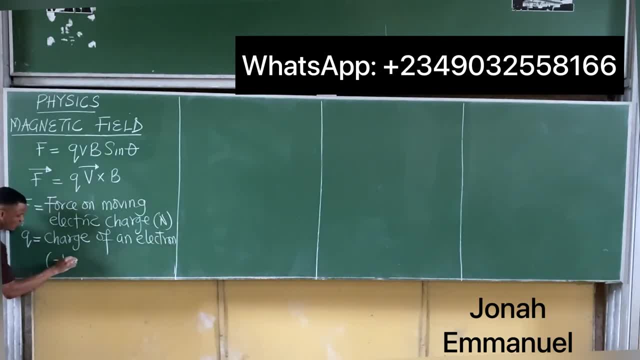 electron is negatively charged, The value is about minus 1.6 times 10 to the power, minus 19 coulomb and that's a constant. So that's the charge on an electron V is simply: we said the charge is moving. 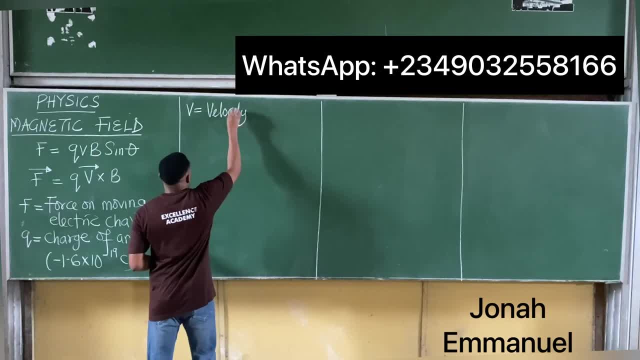 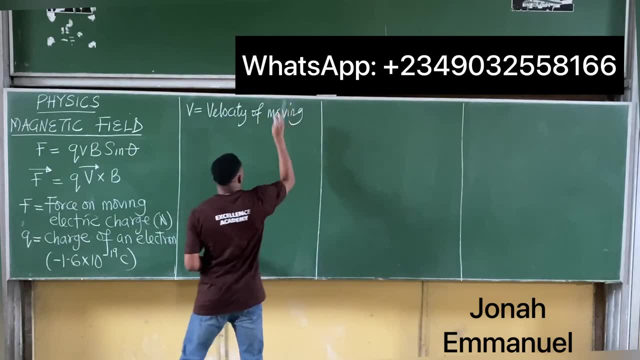 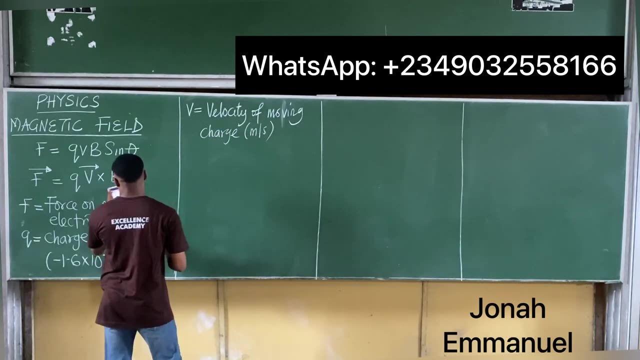 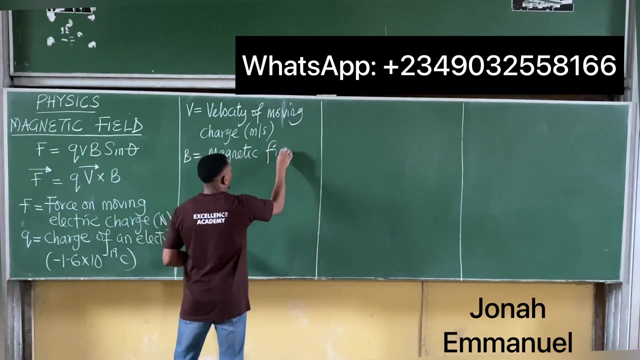 So V becomes the velocity of moving charge. velocity of moving charge, So moving charge, that's in meter per second, and of course V is the magnetic field. the magnetic field, We said it's in per second. We said it's in per second. 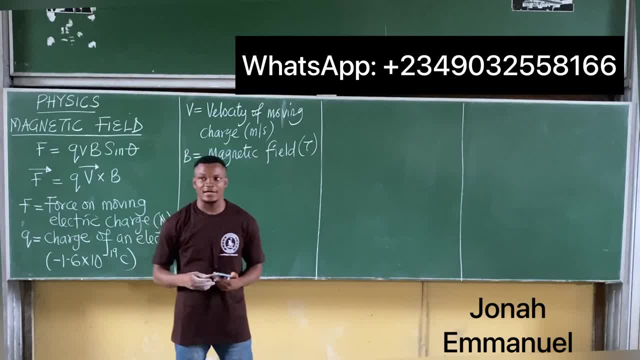 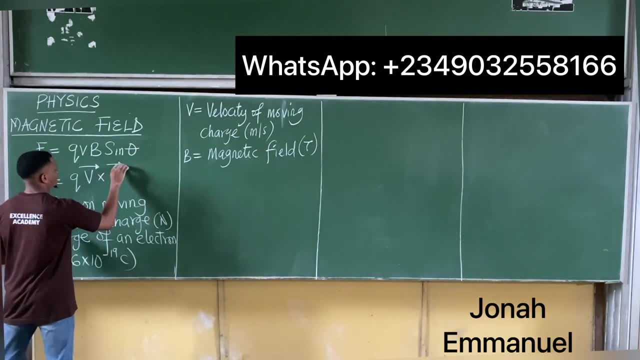 We said it's in Tesla, that's T T-E-S-L-A Tesla in T. So this is the okay in vector form. I have this All right. so I have this in vector form, All right. so here's your vector form representation. 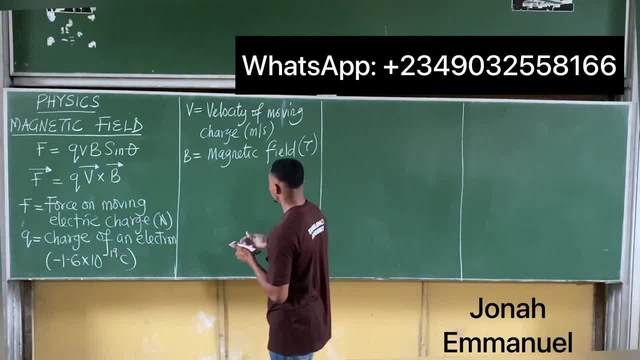 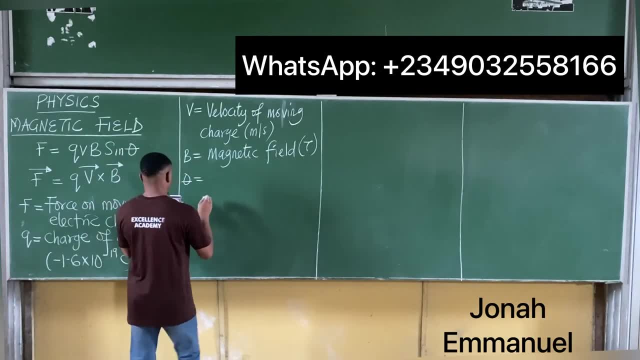 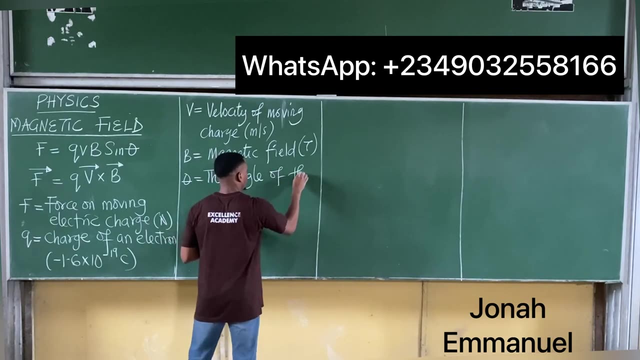 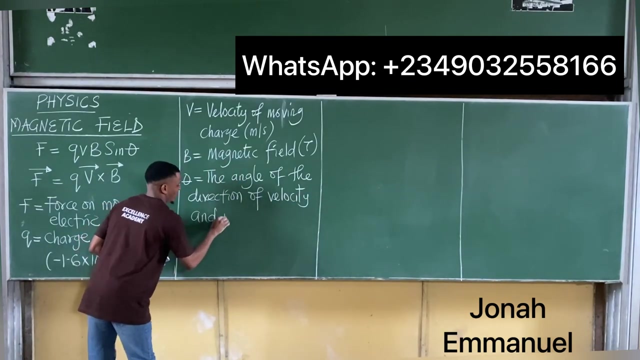 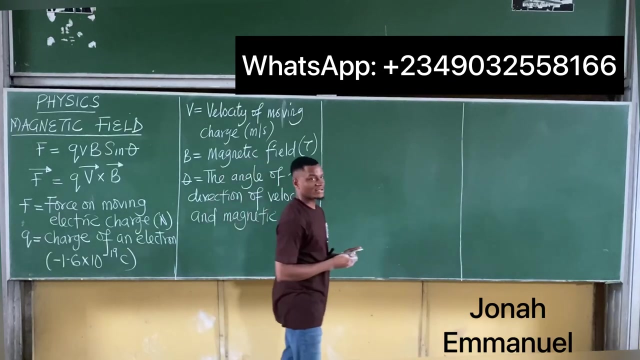 All right. so moving on, theta in this case, theta here is simply the angle of direction of velocity. Okay, So this is the angle of the direction, the angle of the direction of velocity, of velocity and magnetic field, Or simply say that theta is simply the angle right. 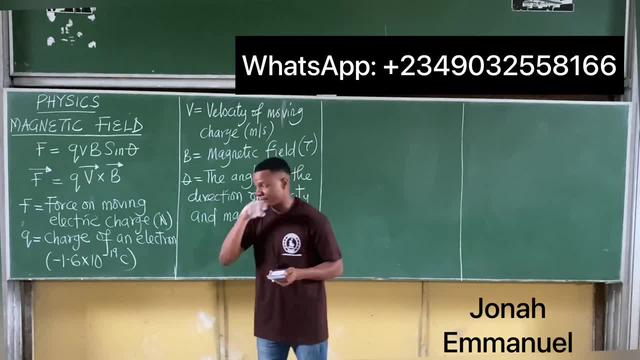 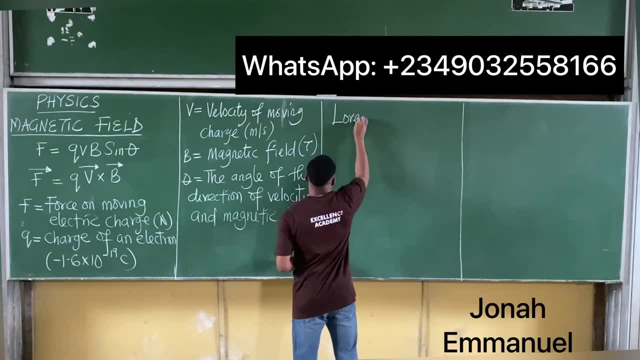 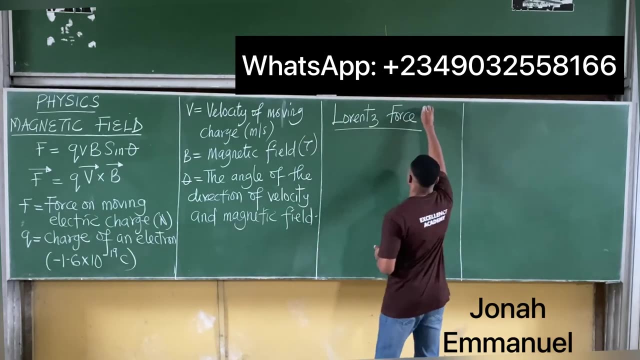 So I have this one here. Okay, So I have this one here. All right, There's something called Lorentz force, something called Lorentz Lorentz force, something called Lorentz force. Let's look at what's called Lorentz force. 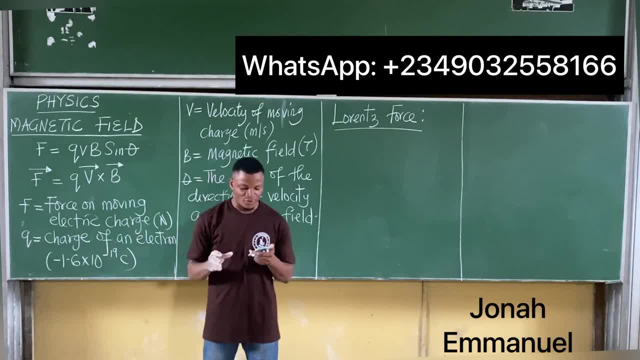 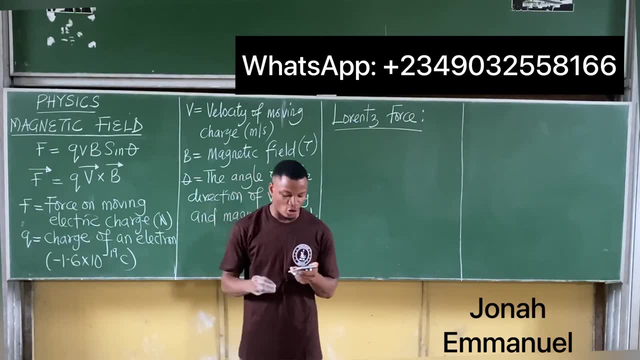 When a charged particle moves in a region of space where both electric and magnetic fields are present, both fields will exist. Okay, Both fields will exact on the particle- a total force called Lorentz force. Lorentz force is simply a summation of electrical force and magnetic force experienced by a particle. 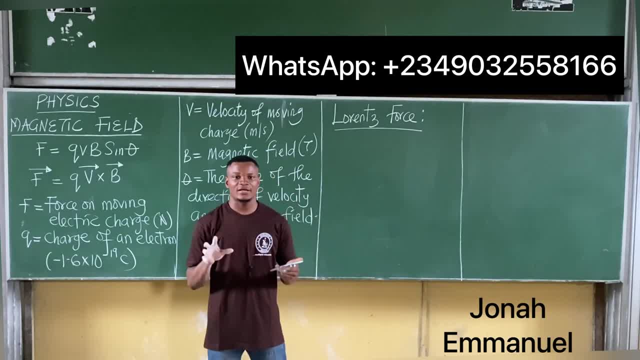 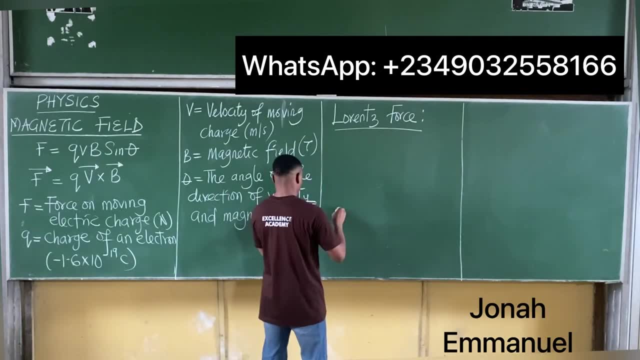 that is placed in an electromagnetic field. That's how you define a Lorentz force. All right, So we said Lorentz force, Let's call this F. Let's call this a total force. Lorentz force- Let's call this F. Let's call this Lorentz force, F L, that's showing Lorentz force. 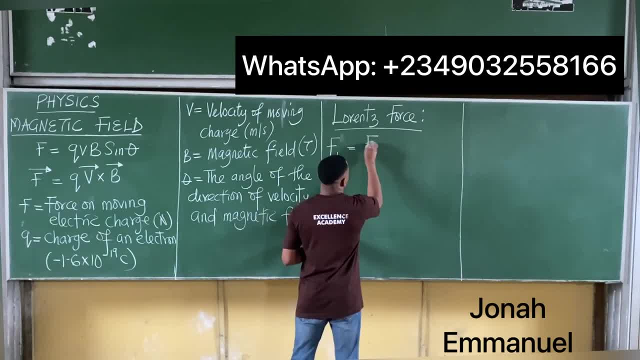 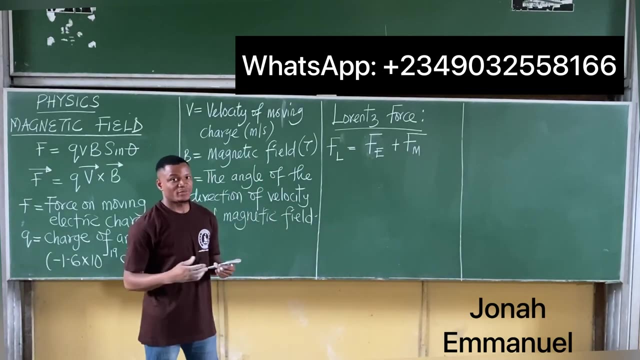 Lorentz, force is simply equal to the electrical force. let me call this F E. call this F E electrical force plus the magnetic force. let me call this F M experienced by a body placed in an electromagnetic force: electromagnetic field. 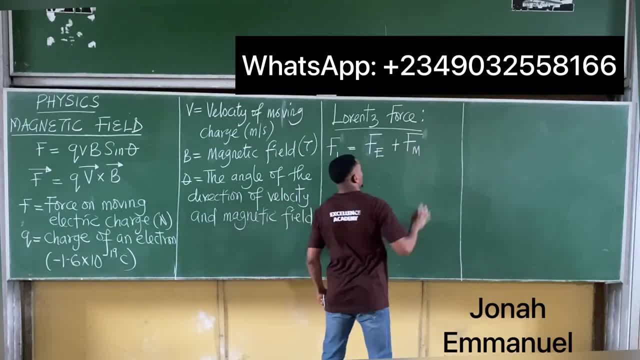 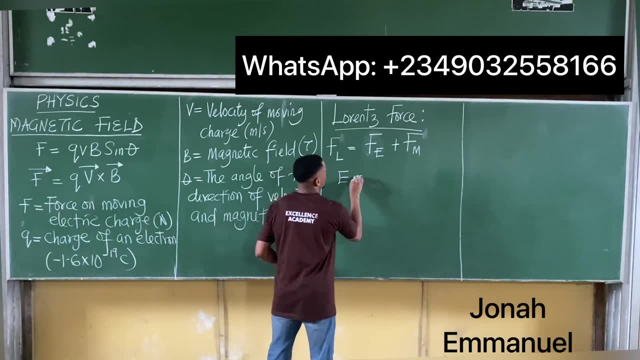 All right. So I have this: Let's get some things done For the electrical force. we said, if you can remember, we said electrical field E is equal to what there force all over charge. Just to be specific, I will call this electric force. 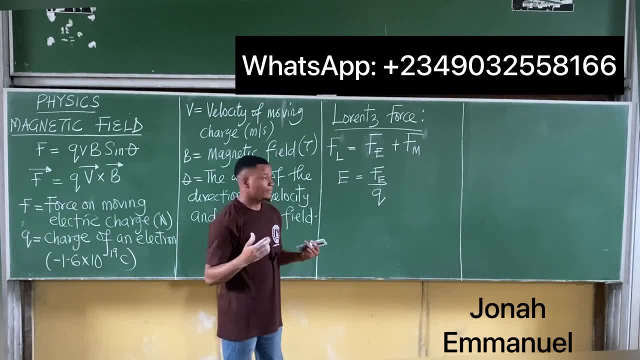 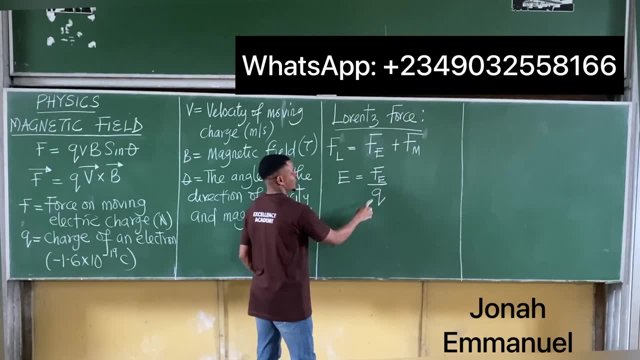 We did this in our previous class when we talked about electrical fields. All right, We said: electrical field E is equal to electrical force over charge. From here, If you cross, multiply this and this, we'll have that the electrical force F, E is equal. 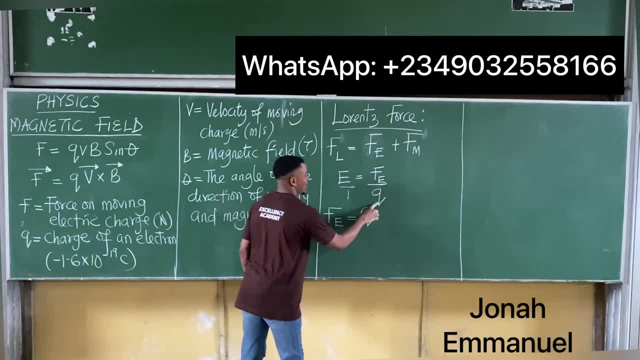 to the product of charge. this and electrical field, We have this. So call this your first equation. if you want to, Let's get for magnetic field, Magnetic field F. we already said this is equal to what there, Q, V, B. that's ignoring. 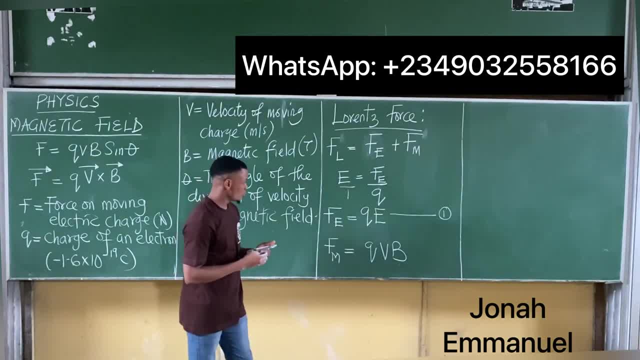 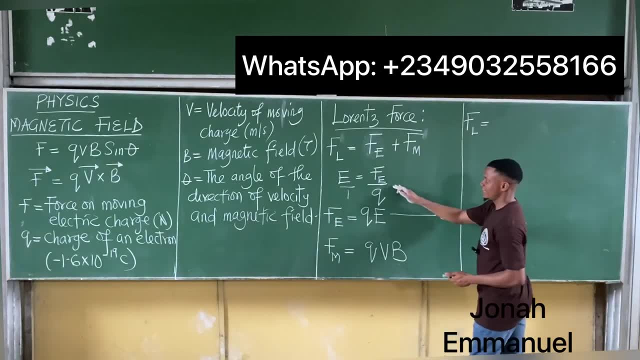 the angle We said F, M is equal to Q V, B. So if I combine these two, it means that Lorentz force, which is equal to the sum total of this and this. so I'll call this equation two. if you want to call this equation two, 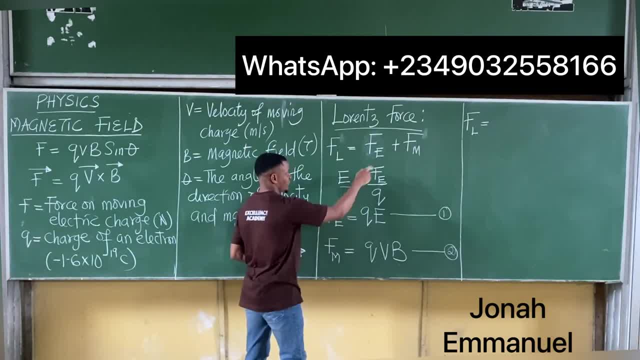 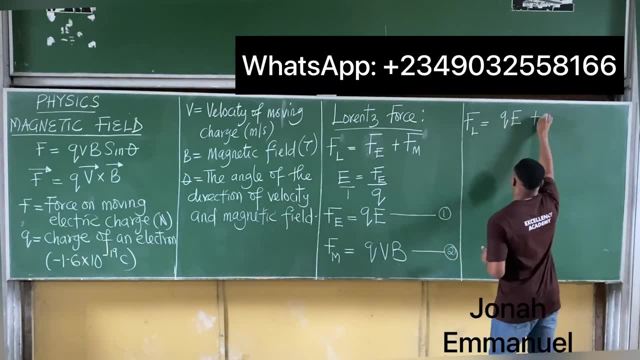 So we said Lorentz force, which is equal to the sum of this, and this becomes, for the first one, I have Q E. I have this. That's for electrical force, For magnetic, I have plus Q E, All right. 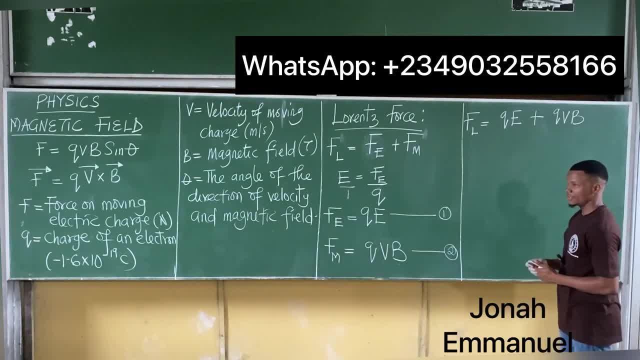 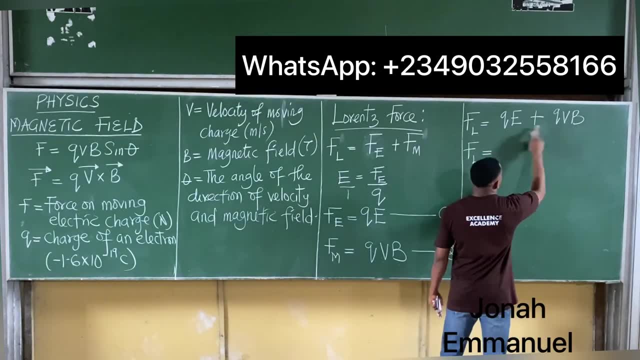 Q V B. So I have these two. So it means that from here that we can get that Lorentz force F, L is equal to. I can see Q on both sides, so I'm having Q here into, I'm left with E plus V B. 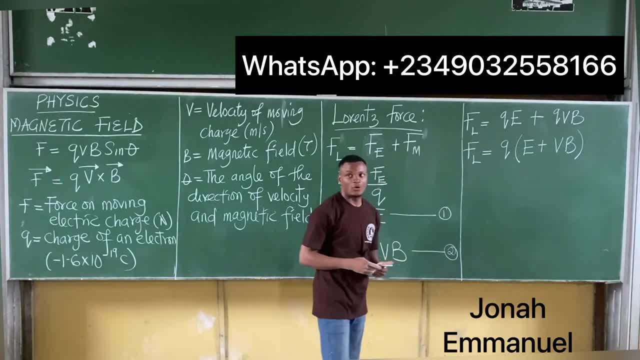 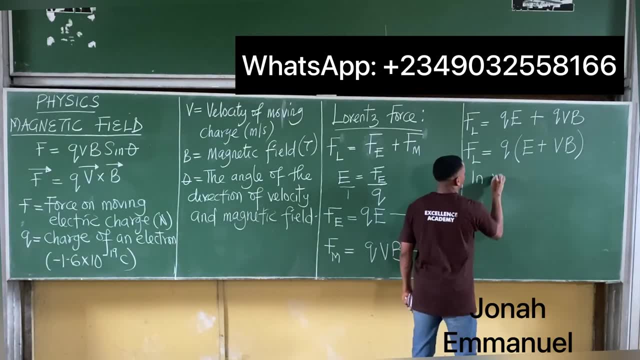 This is your formula for Lorentz force. I have this All right In vector form In vector form. In vector form, Lorentz force is given by this, That's F, L being equal to Q charged on an electron. 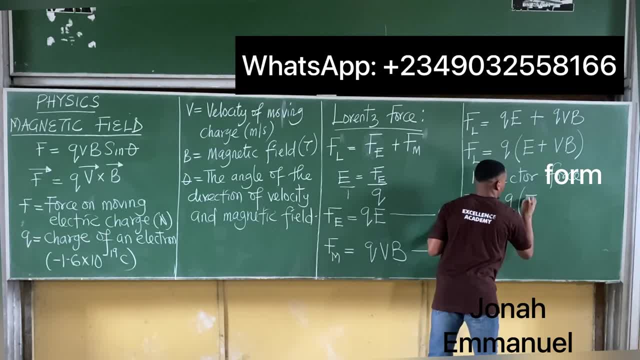 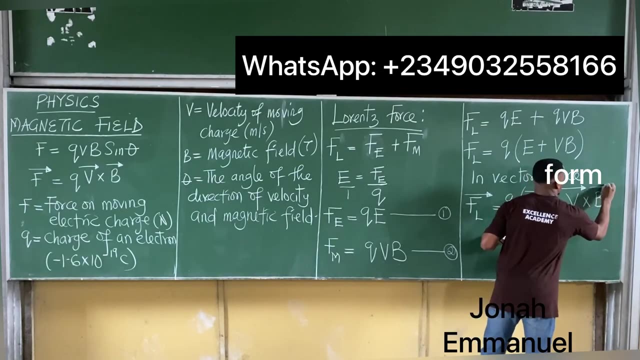 Q into electric field. in vector form is E having R on the head showing direction. plus, this product here becomes a cross product. It becomes V cross B. Now it's V cross B. Both are vectors. So I have this and I have this. 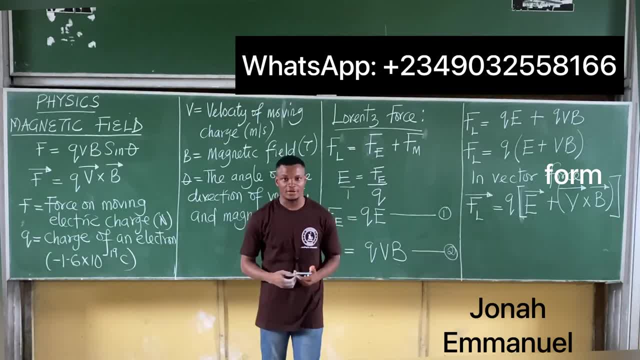 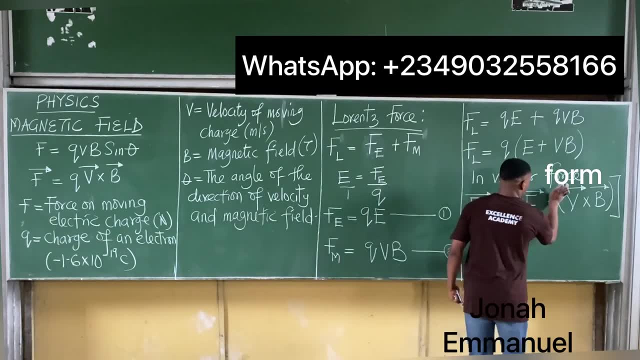 So this is Lorentz: force representation in vector form. All right, So let's move on. I will take some examples. I will solve on this. Let me call this a plus, please. Here's a plus. I'm having this as this, plus this: 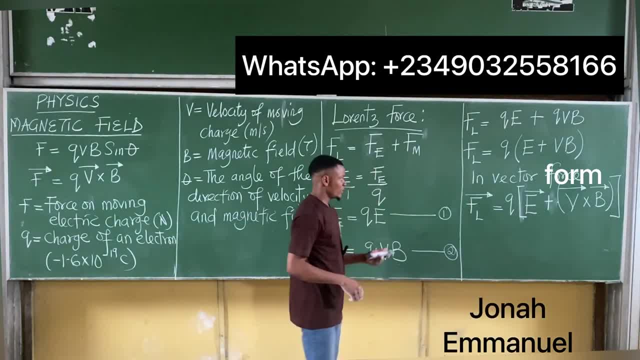 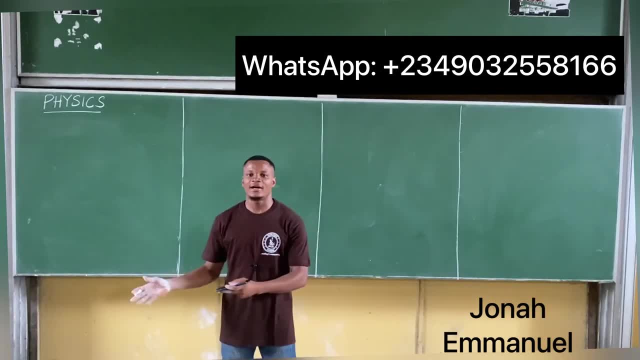 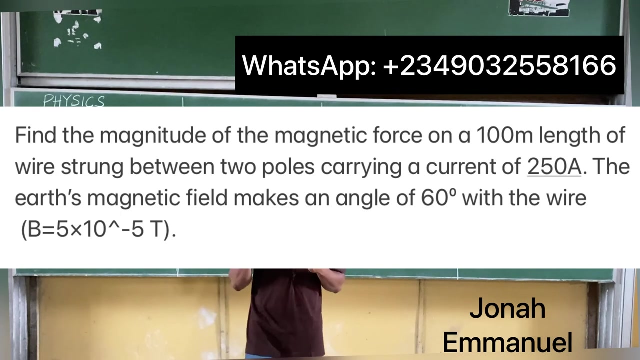 All right, So let's solve problems on this. All right, So we'll take an example on both the scalar and the vector problems on magnetic field. All right, Let's start with the first one there. The first one says: find the magnitude of the magnetic force on a 100 meter length of. 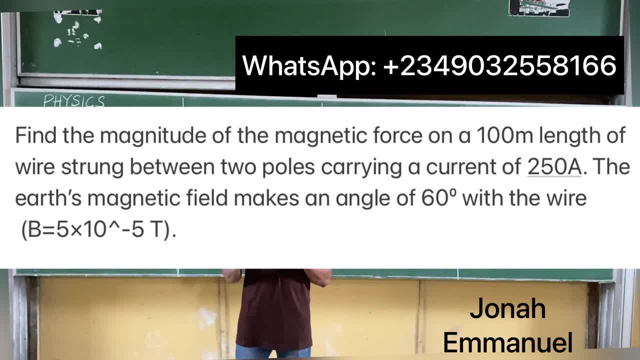 wire strong between two poles, Carrying a current of 250 amperes. Push, stop. The X magnetic field makes an angle of 60 degrees with the wire. It said: take the X magnetic field B as equal to 5 times 10, to the power minus 5 Tesla. 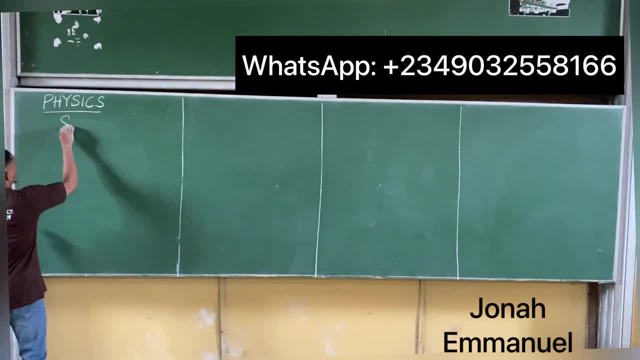 All right, Let's get this done. So solution there. As usual, Our first task is to list out given parameters. The first thing I'm given there they said a force on a 100 millimeters length, So the first thing I'm given there is length. 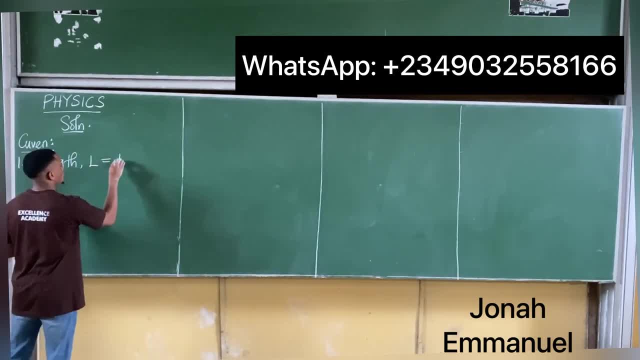 The length of conductor in full Length is equal to 100 meters. Moving to the third, Carrying a current about two, The current that's I is equal to, So 50 amperes, So I have 250 amperes. 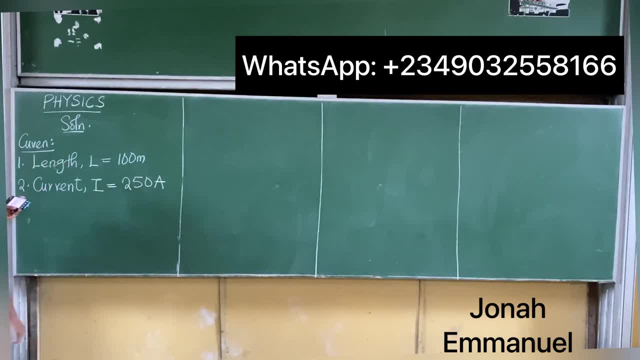 Also to give us the angle number three. I'm given angle there that theta has been equal to 60 degrees. I'm having 60 degrees here, All right, It said. finding number four: The X magnetic field does this Was giving us 5 times 10 to the power minus 5 Tesla. 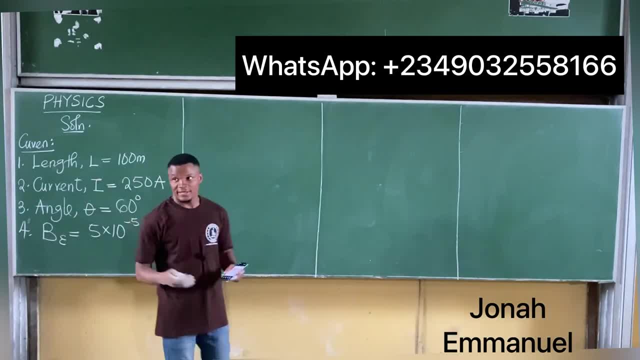 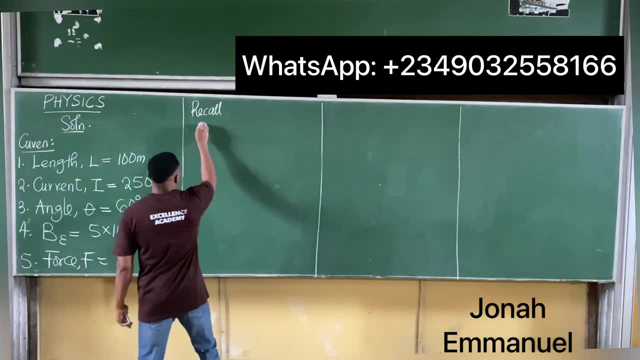 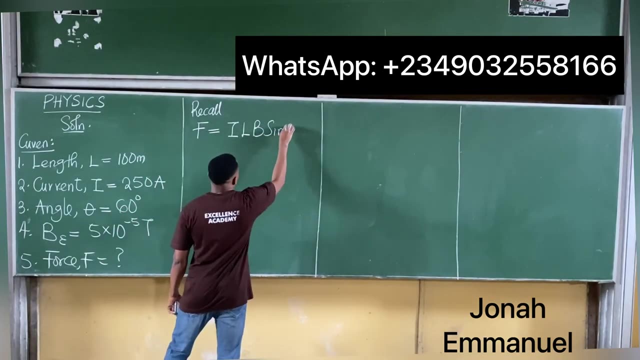 minus 5 tesla. all right, let's solve this question. let's recall formula record that F, from what we said, the force on the conductor, current F, is equal to I, L, B sine of theta. we have this. this question here is for scalar. now, how do 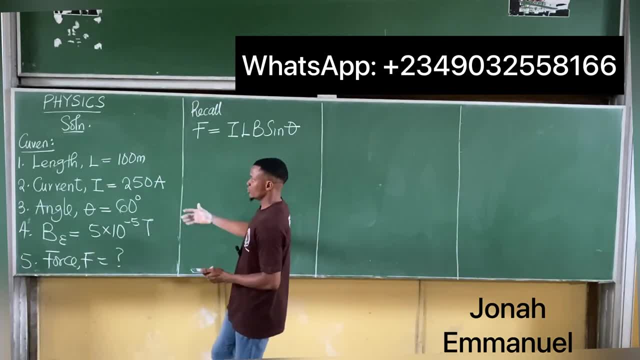 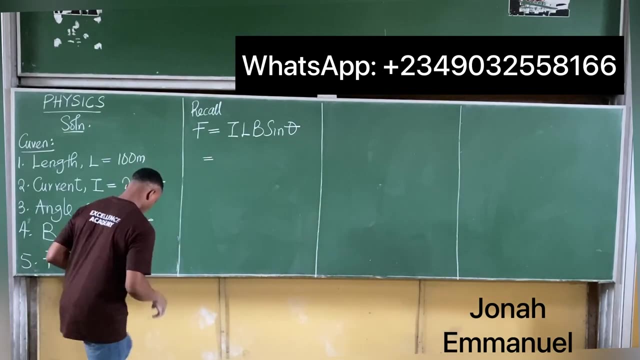 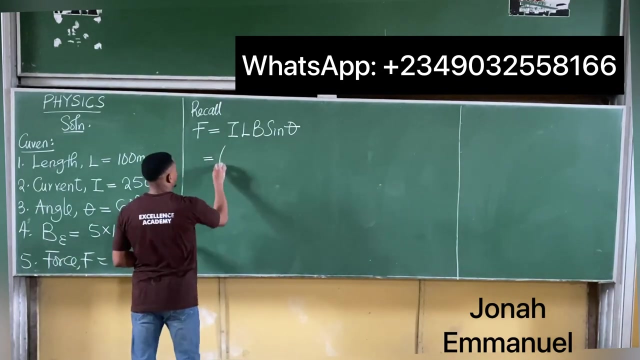 we know scalar because there is no I and J component. so whenever you are given a question on magnetic field when there is no I and J component, you know it's a scalar concept. so from here let's include values. this is equal to. so I'm having I current is 250. 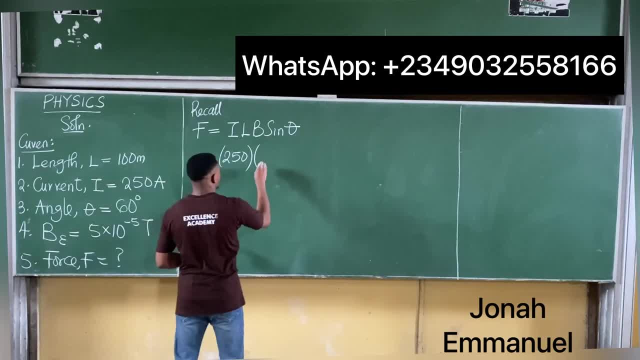 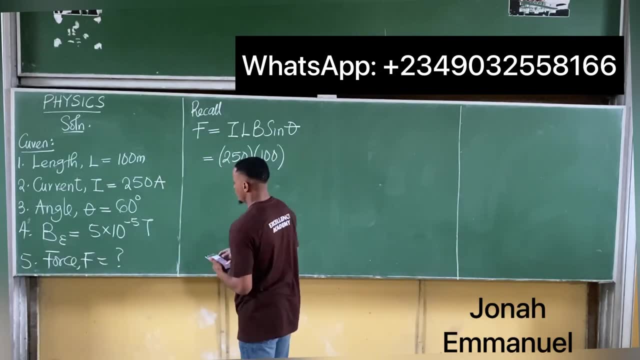 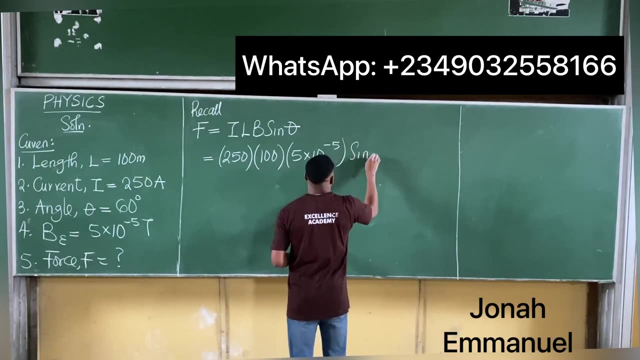 amperes, let's get L. the length is 100 meters, I don't have to convert again B, the, the round codes I have. Mexican field, magnetic field is 5 times 10 to power minus 5, and then sine of theta, theta. here is the. 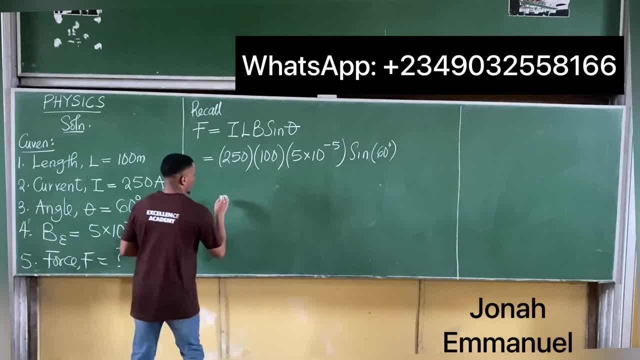 angular 60 degrees. I have 60 degrees. if I get this gun I'm having this is this. so 250 times 100 times five times 10 to power minus 5, I have 1.25. that gives me 1.25 w y. 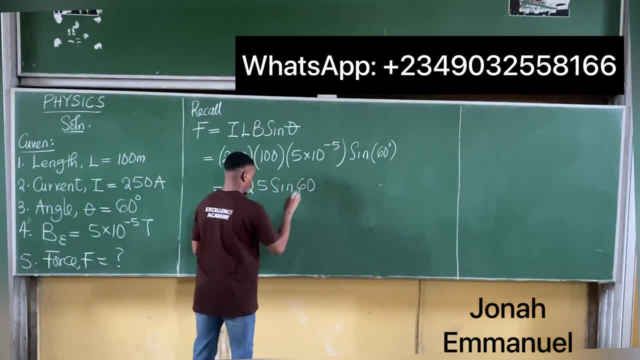 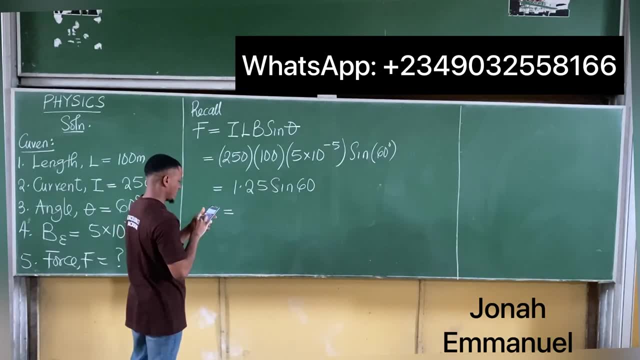 times sine 60. alright, so if I punch 1.25 sine 360 I'm having 1.25 sine 60. that's about 1.08 approximately. that means the force experienced by the conductor is about 1.08. of course, in Newton this is approximately 1.1. 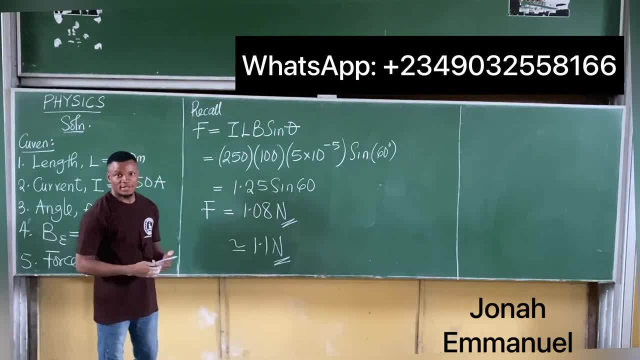 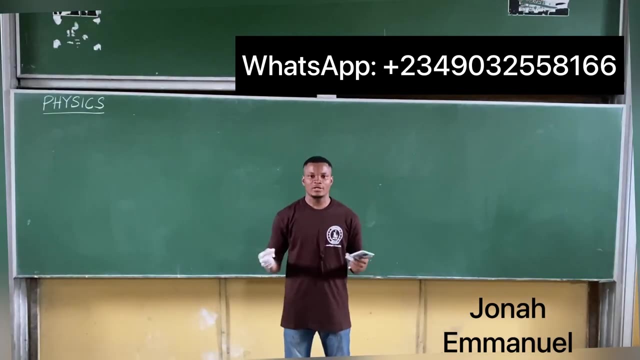 Newton, that's. if I want to use 1, this is my place. so this is how we get this done. let's look at a problem on this in vector form and we'll see how to solve problems on magnetic force in vector form. let's look at the second example, but this time. 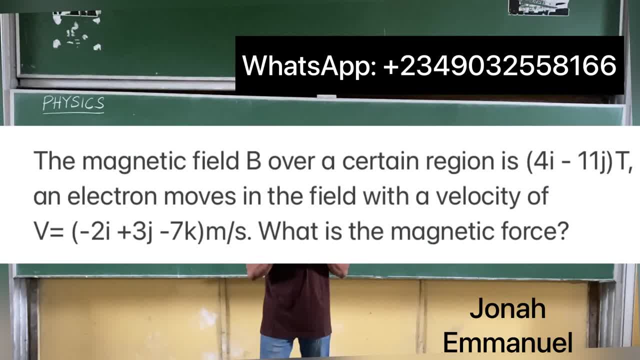 in vector form. this question says the magnetic field B over a certain region is 4I minus 11 J. Tesla, an electron moves in the field with a velocity of V being equal to minus 2I plus 3J minus 7K. what is the magnetic force? 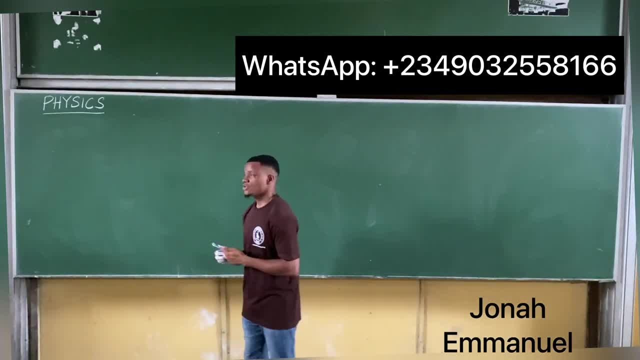 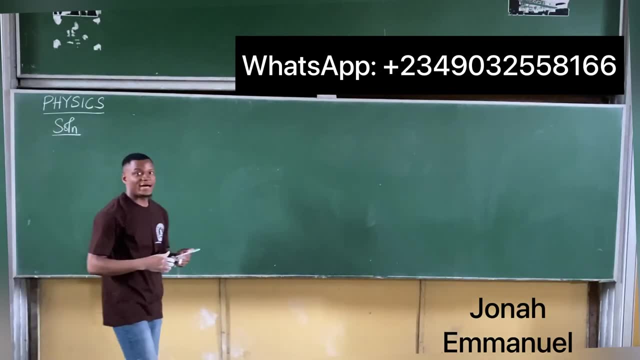 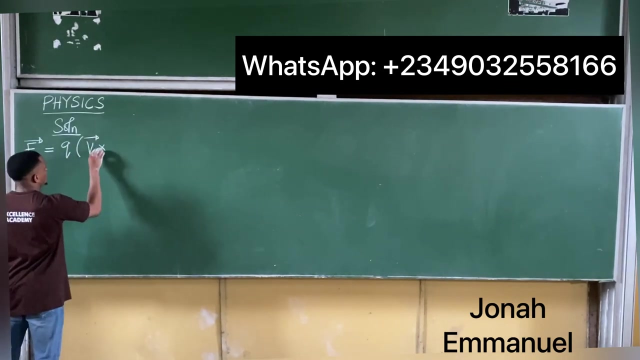 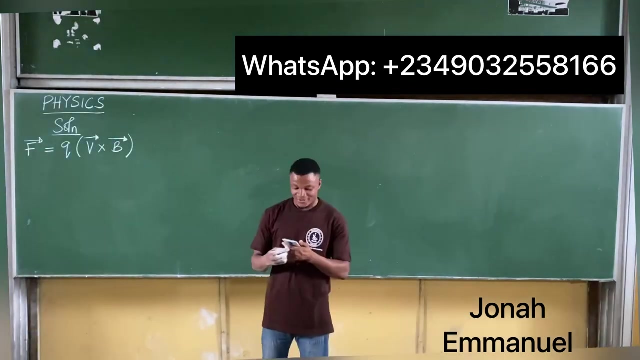 and that's your question. alright, let's get this done, please. so this one now involves a vector form because, as you can see, there there is an I and a J and obviously also a K. so this one now involves a vector form because, as you can see, there there is an I and also a K: Heart. 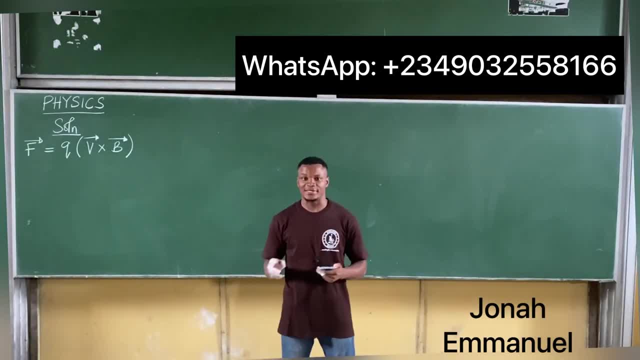 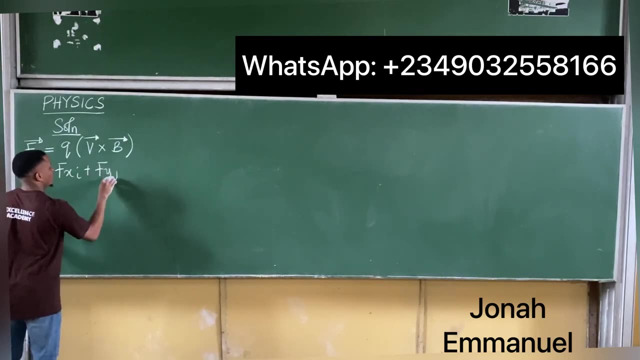 goes through each of these cages, total seed, so the average around an hour. RCции, boiler and the K component. that means F, F itself. F itself should be equal to F, X, I plus F, Y, J plus X, Z, K, also V, this one. here, of course, Q is a constant. the force of an electron. 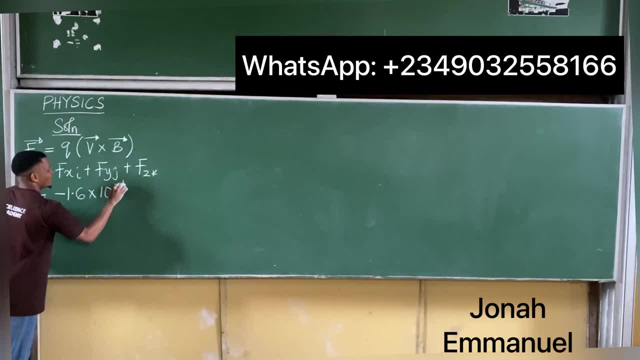 minus 1.6 times 10 to the power minus 19. volume V, also in vector form, is equal to V X I plus V Y J plus V Z K. and then finally we have B: electric field, also in vector form, is: 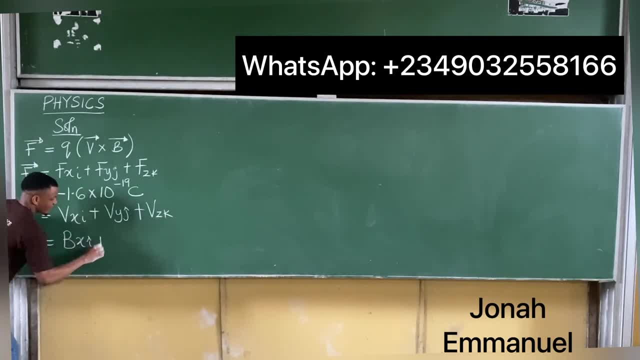 equal to V X, I plus V Y, J. Okay, so I have this one here, all right. so I have this next thing. so what I'm giving here? so what I'm giving here. if you have these two in vector form before, then let's. 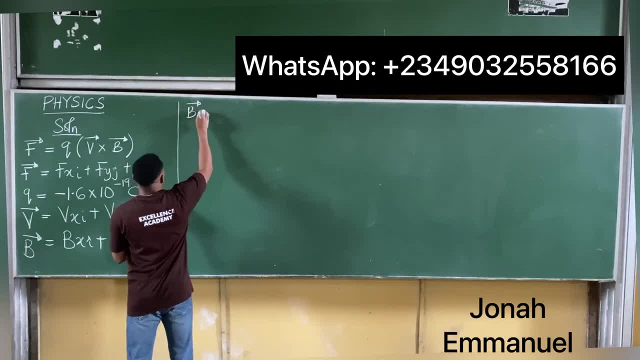 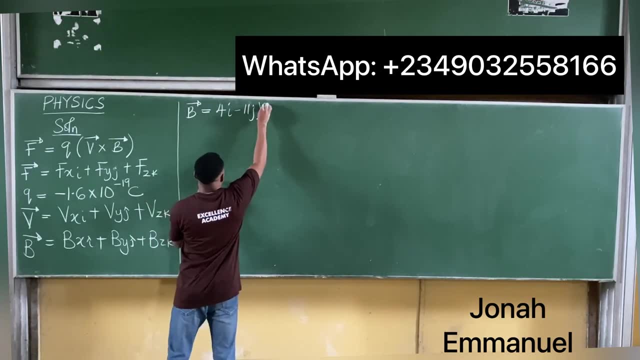 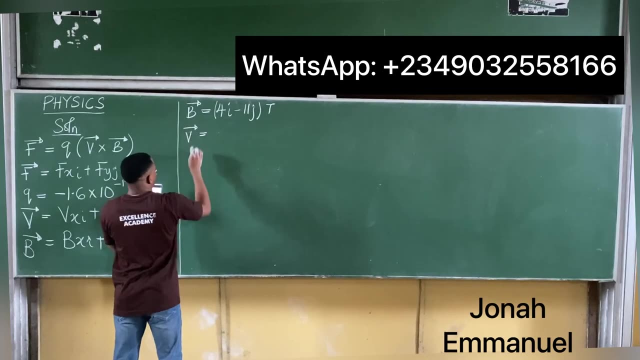 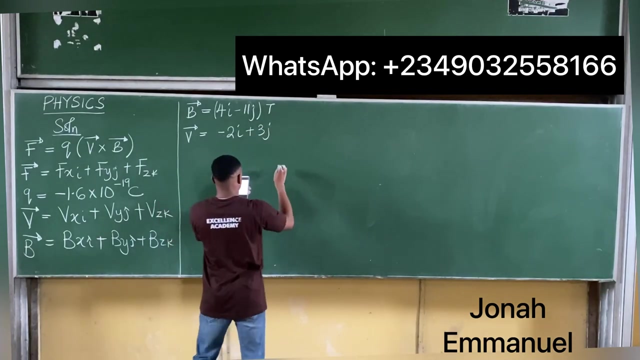 list out what I'm giving there. I'm giving the magnetic field D as being equal to 4 I minus 11 J Tesla, that's B. I'm also giving V, so V also is equal to. I'm giving this as minus 2 I plus 3 J minus. 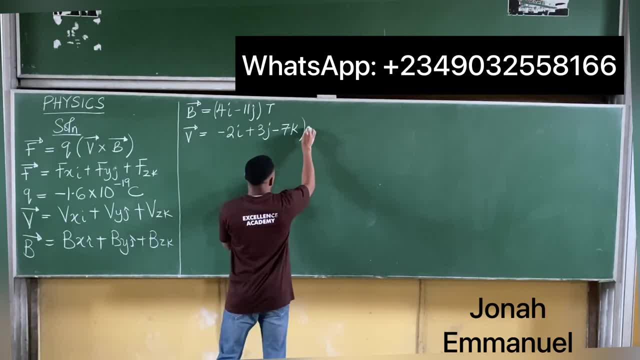 7 K, this in meters per second. so I have this all right. so I have these two here. observe: here it's in Tesla, so I'm not converting. so if there was a milli Tesla, becomes times 10 to the power there minus 3.. 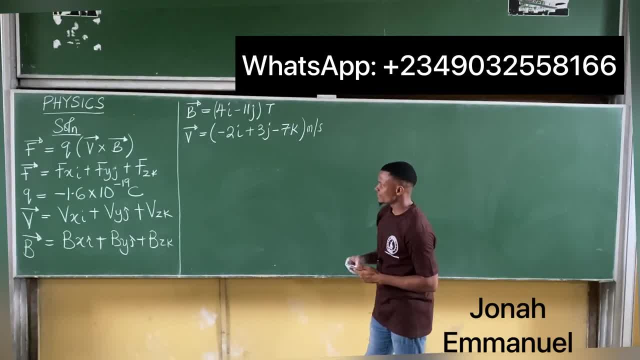 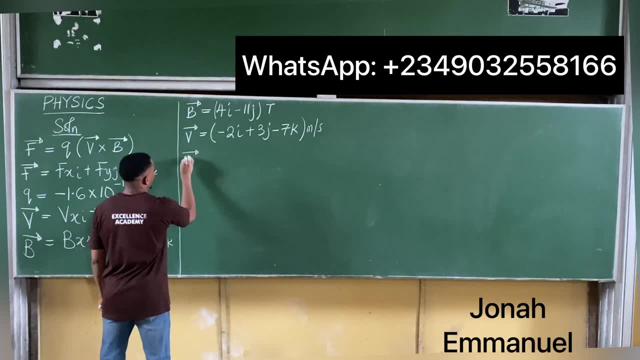 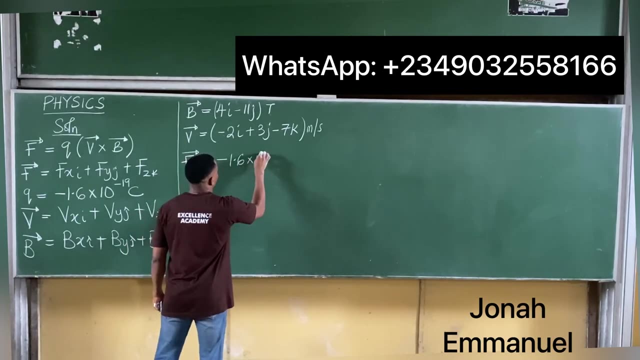 So what I'm doing here, I won't stress, I'm not converting. so how do I solve this? This is as easy as this. so from here I'll have that. the force on this, the F force on this, is equal to Q. Q is minus 1.6 times 10 to the power minus 19,. so this is Q into. 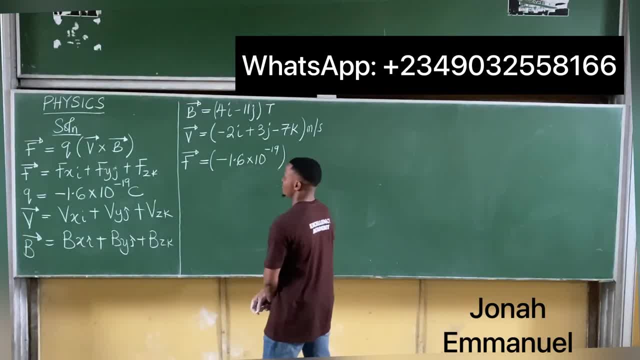 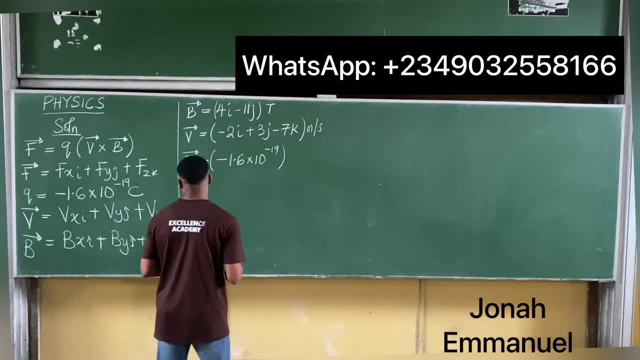 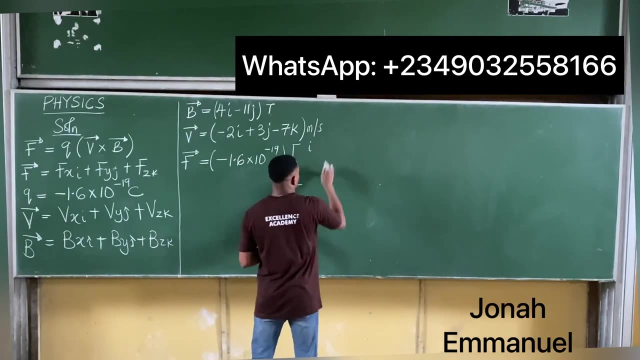 let's get V cross B. for V cross B now, remember what we did in our previous class. we did cross product of vectors. Okay, To get V cross B. what we'll do is this our first task. we'll get the I, J and K- yep. 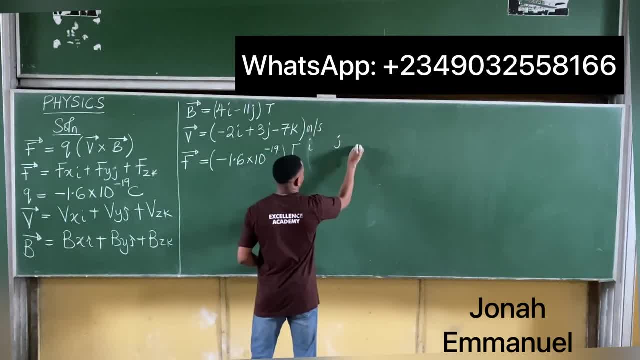 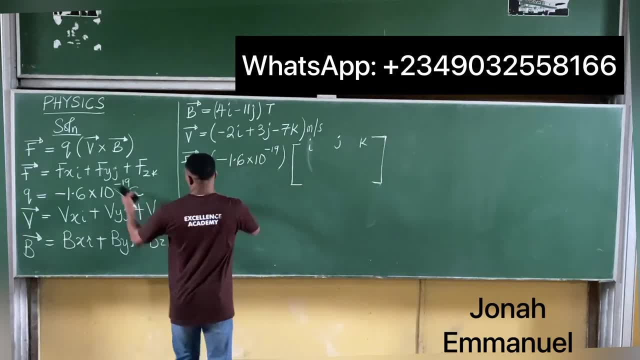 our first task is to get the I, J and K complete like this. so this is your first task Now, since this is V cross B, that means VX, VY, and then VZ comes first and then we get. 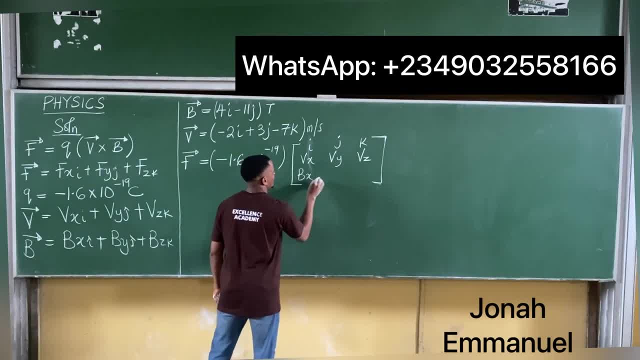 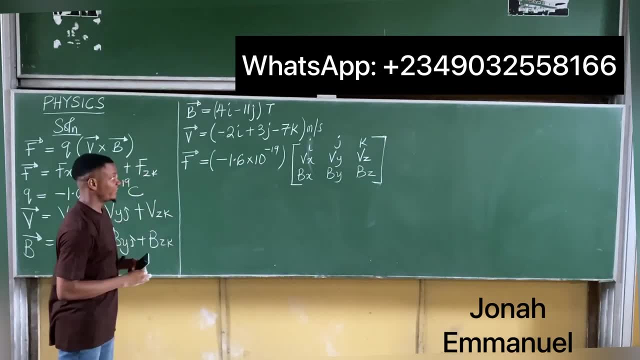 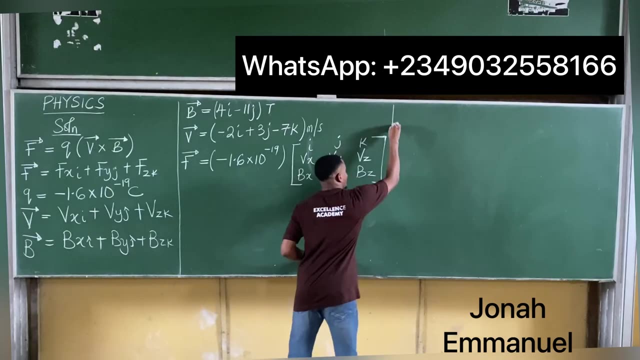 the I, J and K and then next up B, so we're having VX, VY and then VZ. so this is how you present this man here in vector form. I didn't use sine theta because the angle theta was not given, so we have this alright. 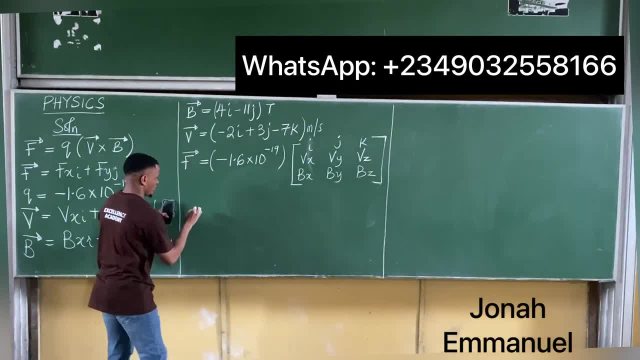 let's get this done, so let's impute values. This is equal to minus 1.6 times 10, to the power minus 19.. I have this Okay. So this is equal to minus 1.6 times 10, to the power minus 19.. 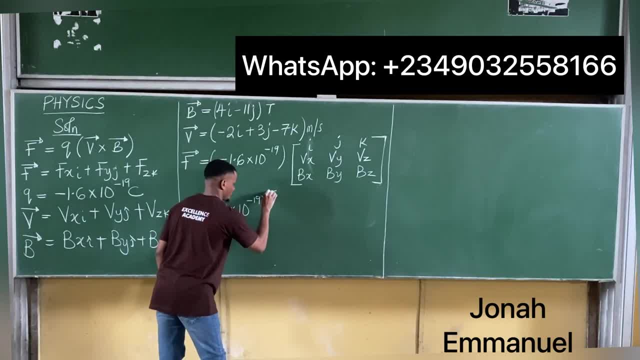 I have this. So plus minus 1 times, 10 times 13-12 to the power 14-13, plus 1 into for this one. here I have I J K VX. VX is, if I look at the value here, the VX is the I component or the coefficient of I. 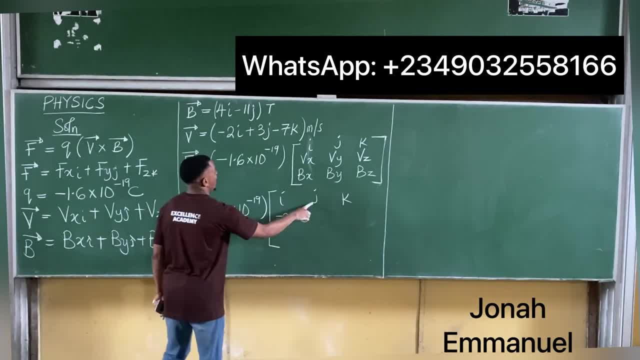 which is minus 2, so I have minus 2.. Y is the coefficient of J here, which is plus 3, so I have 3 or plus 3, same thing: K becomes the the K here. what you put here becomes the what you get here. 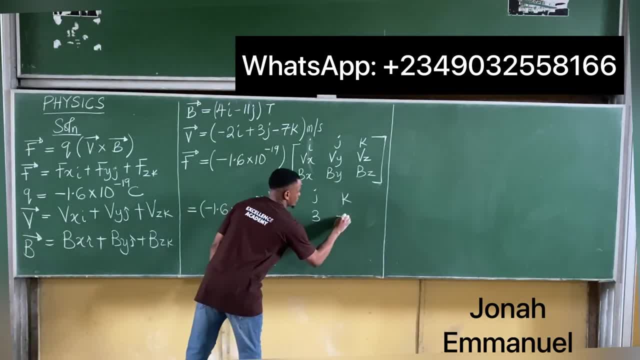 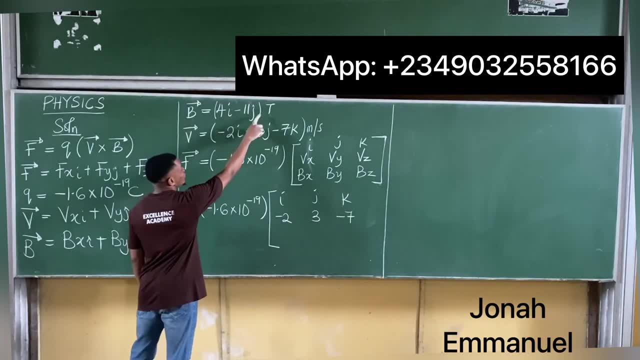 Thefunds, the equation of k here, which is minus 7 for v, so I have minus 7, so I have this into. let's get for b. b has just i and j. no k For i. there the coefficient there is 4, that's for b. 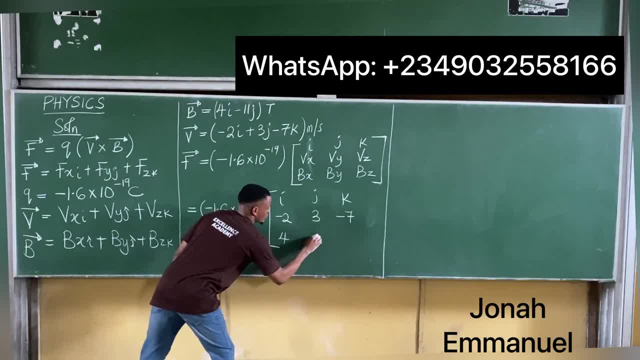 For j, the coefficient is minus 11, so I have this. Since b has no k component, the coefficient here becomes what there, 0.. I have this Alright, so you have this. This is my representation, So let's get this done. 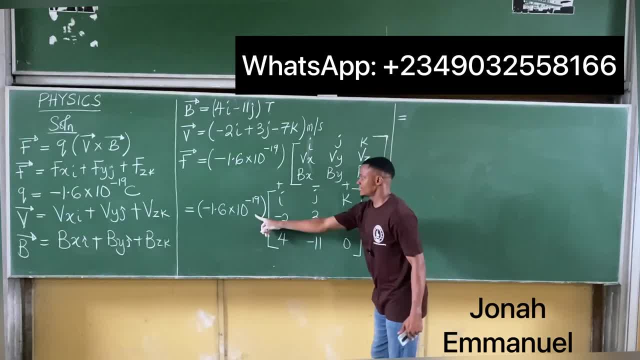 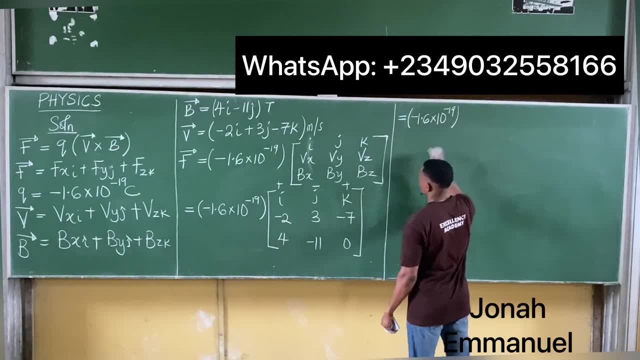 So that's now equal to. so this is equal to: I'm having this charge of an electron minus 1.6 times 10 to the power minus 19,. so this into this one here. So how do we solve a matrix of this form? 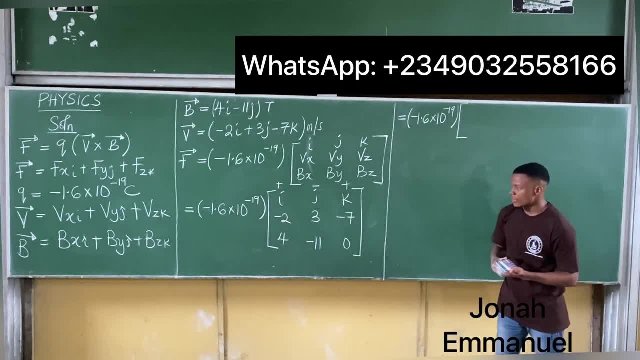 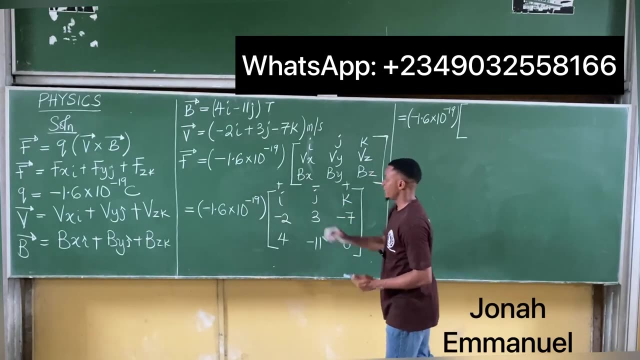 We've done this in our previous class when we did vectors, so I'll leave a link to the. okay, no links, no links, please, no links, Alright. so how do we solve this? This equals I'm having a plus. i. 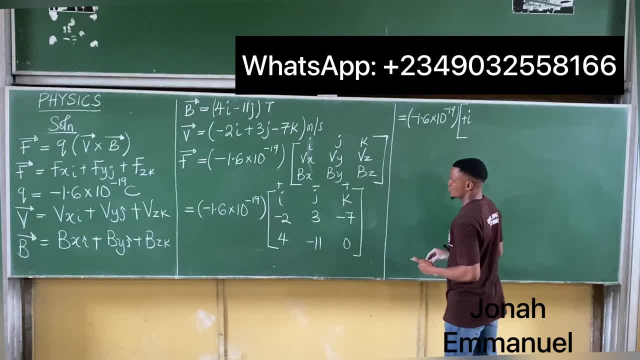 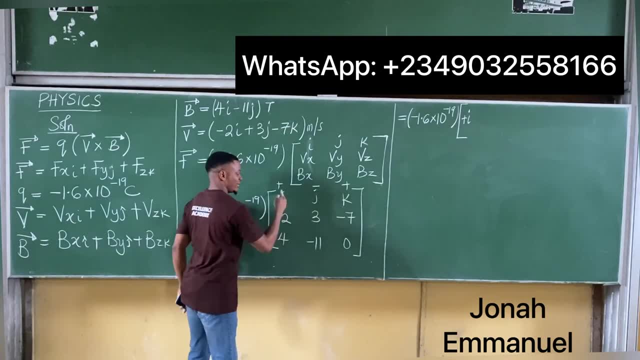 so I'm having plus i into, for i, here, I'll cover the role and the column like this. so i, here's your role, here's your column. Cover the role, cover the column. I have 3, minus 7, minus 11, 0.. 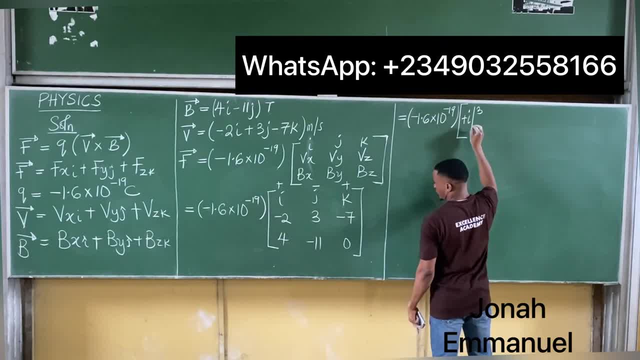 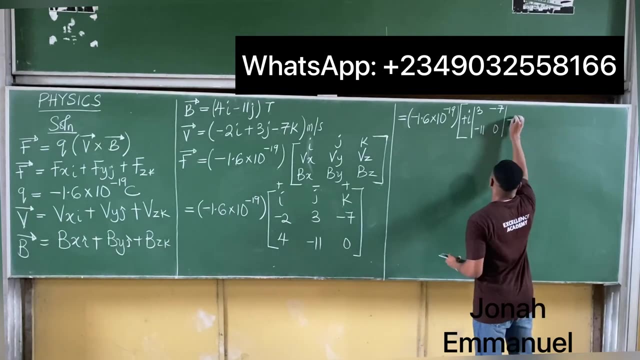 So I have this as 3,, 0.. Minus 7,, minus 11, and 0.. That's i. Let's now get j. So I'm having a minus j, So I'm having minus j, For j cover the role and cover the column. 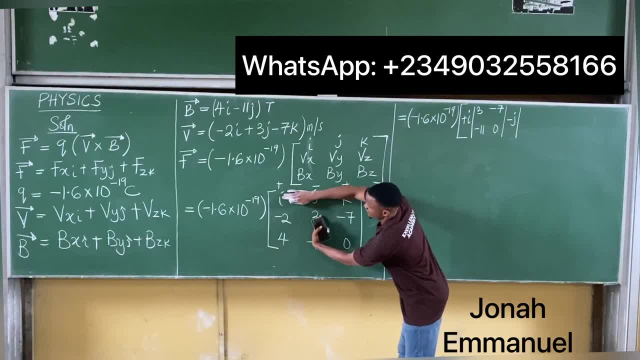 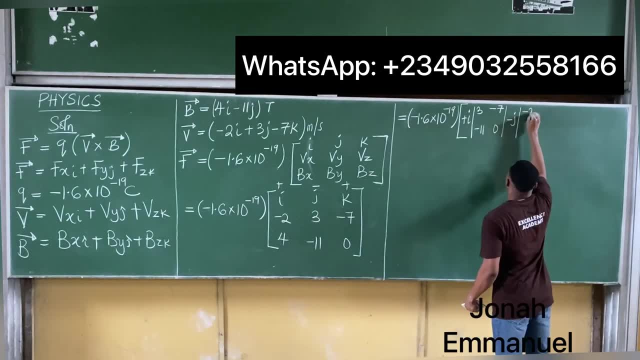 For j. my role is this, my column is this: So I'm left with minus 2, 4, minus 7, 0. So I have minus 2, 4, minus 7, 0. So I have this. finally, I now have a plus k. 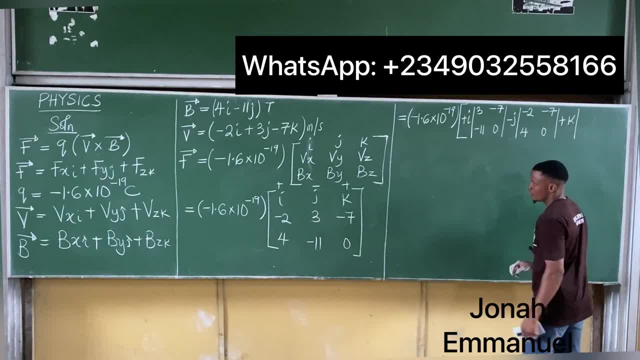 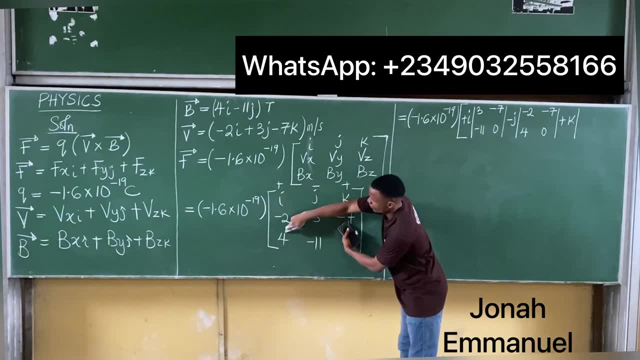 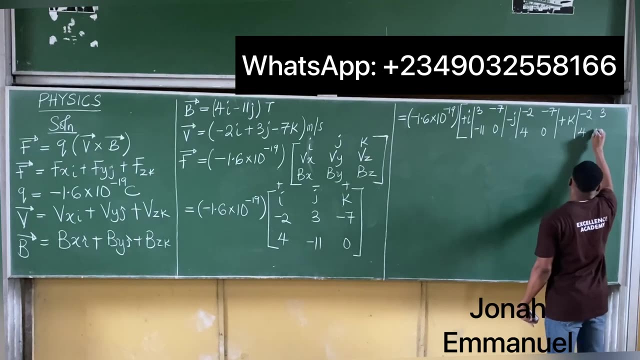 Finally, I have plus k into for k cover, the role cover, the column. I'm having minus 2,, 3, 4, minus 11.. So I have minus 2,, 3,, 4, minus 11.. 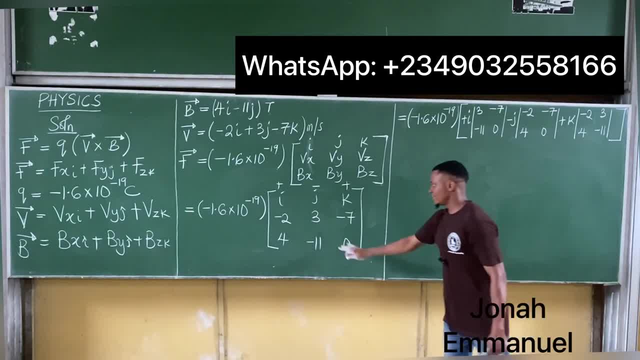 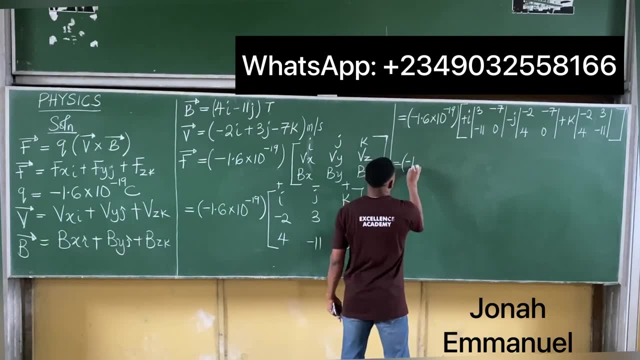 So I have this. so this is what I have. After simplifying this, I will now have this. Alright, let's solve for that. This is now equal to: I have minus 1.6 times 10, to the power minus 19,. 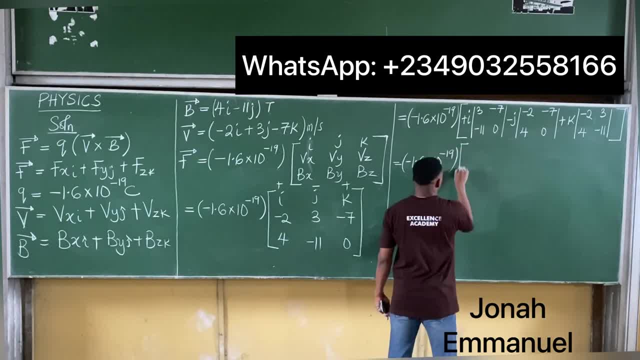 into. let's get this done. this gives you plus i. To simplify this, it's as easy as multiply this and this. this is called a principal diagonal. to multiply this two, 3 times 0,, 0, minus this times. this. 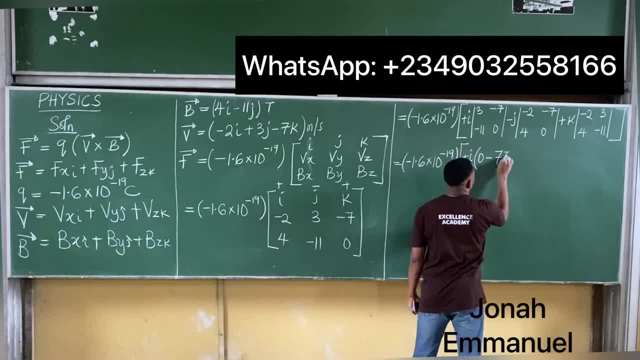 minus 7 times minus 11, is plus 77, so I have this. next up is minus j, so I'm having minus j into this times. this. minus 2 times 0 is 0, this times this, of course, minus first. so minus this times this. 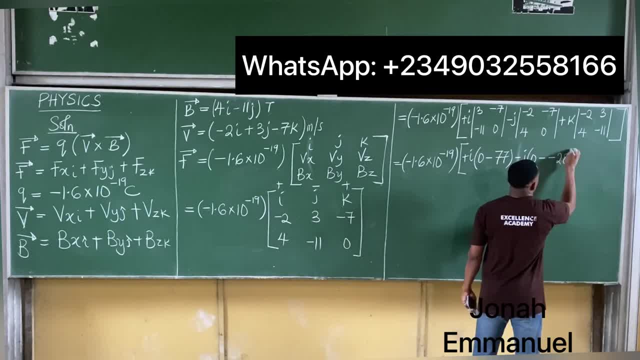 minus 7 times 4 is minus 28,. plus, and I have k, it becomes plus k, plus k into this times. this minus 2 times minus 11, is plus 22,. minus 3 times 4,. 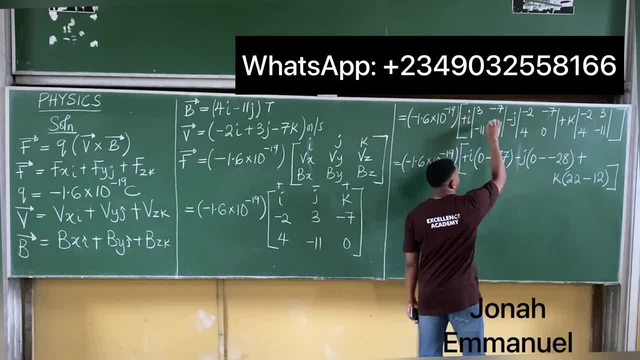 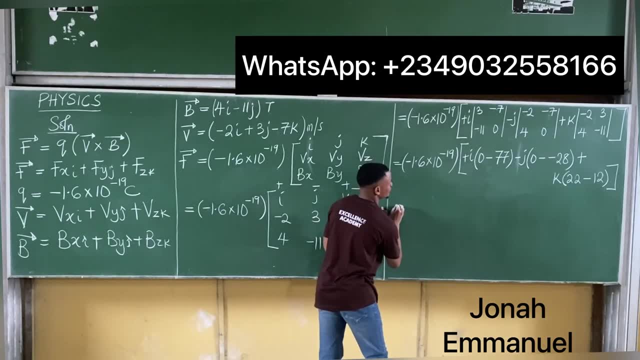 is 12, so I have this. so it's always equal to this times this minus, this times this for all of them. so I have this case here proceeding. this is equal to. this is equal to I'm having this as. 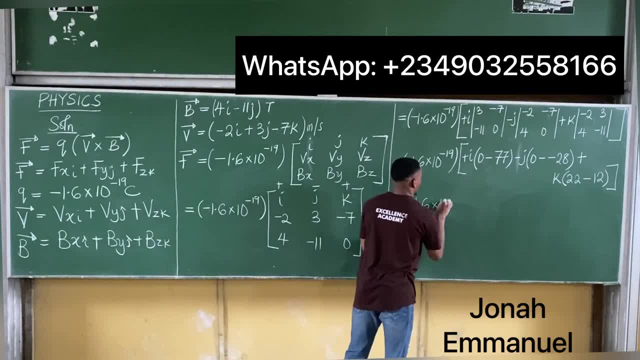 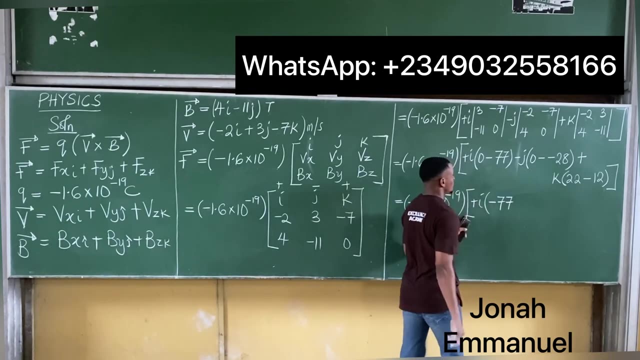 minus 1.6 times 10 to the power minus 19,. this into, if I work this out here, I'm having this as plus i. so plus i into 0 minus 77, is minus 77,. okay, next up. 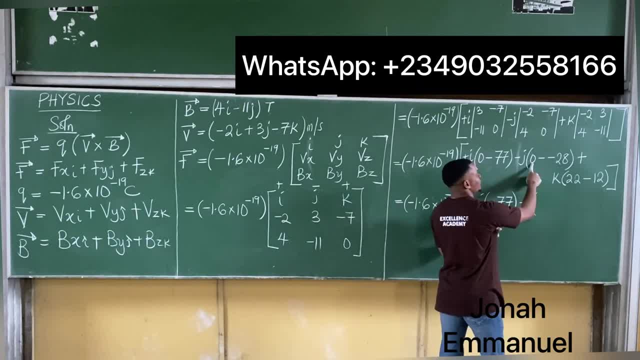 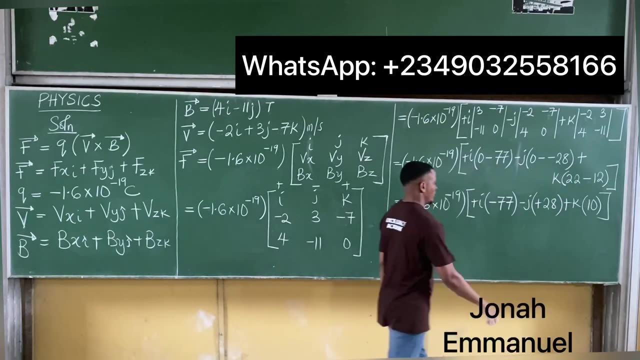 minus j, so minus j into 0,. minus minus gives you plus, so it becomes plus 28,. plus k, so plus k into 22. minus 12, gives you 10, so I have this one here. all right, let's simplify for that. 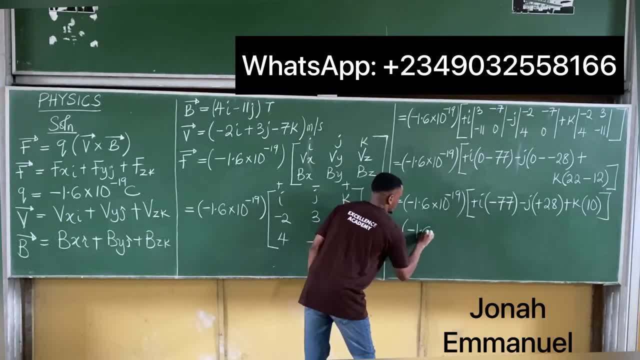 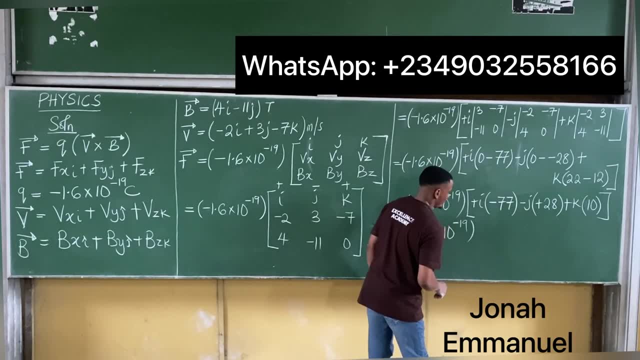 this is equal to minus 1.6 times 10, to the power minus 19,. into, let's get this done. what do you have here? this becomes minus 77 times. i gives you minus 77. i okay, minus times. 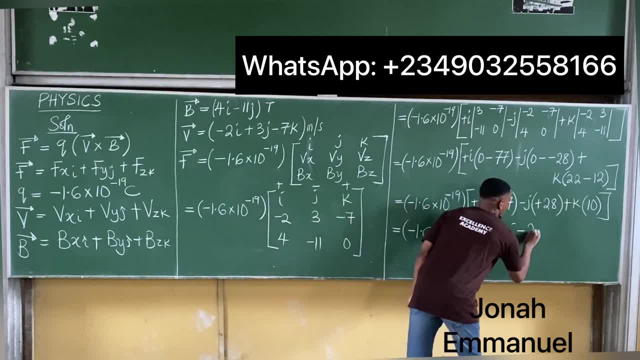 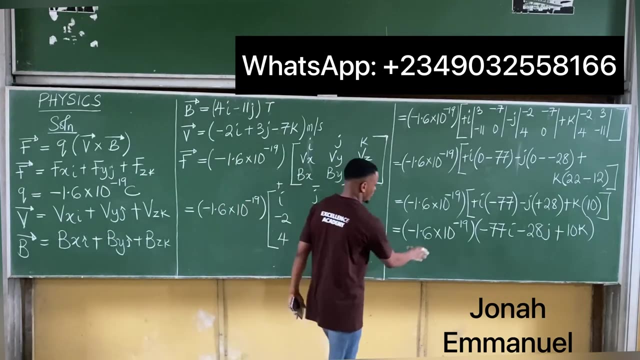 plus minus j times 28,, 28 j plus times plus plus k times 10, 10 k. so I have this all right. so I have this one here, my last tax number. use this to multiply it through if I use this one. 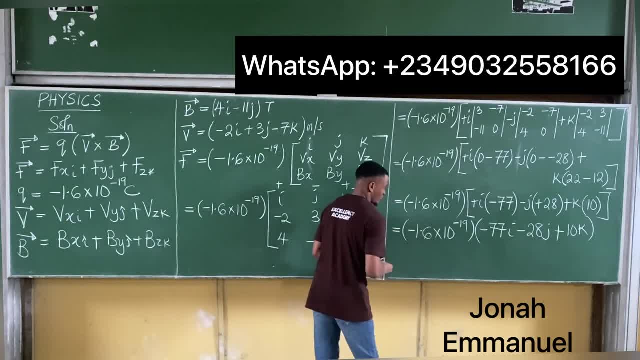 here to multiply it through. what do I get? so this is now equal to all right, so my simple idea will now be that f will be equal to. your simple idea will be this: use this one here to multiply the numbers. 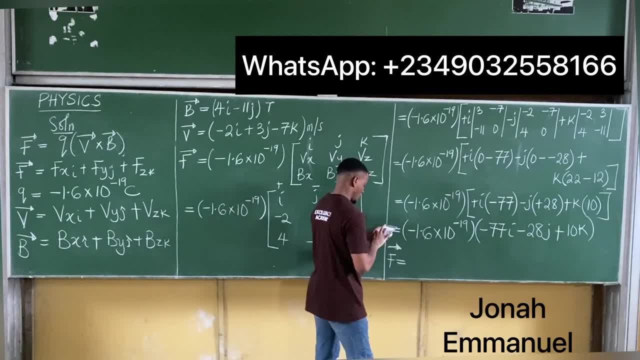 so the first thing here is minus 1.6, minus 1.6 times minus 77, that's about 123.2,, that's 123.2i. so I have this as my i, so this is this. i let me use normal i, so i, here next up, use this and this, so it becomes: 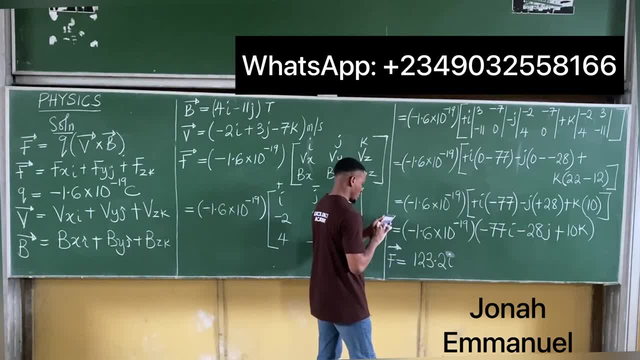 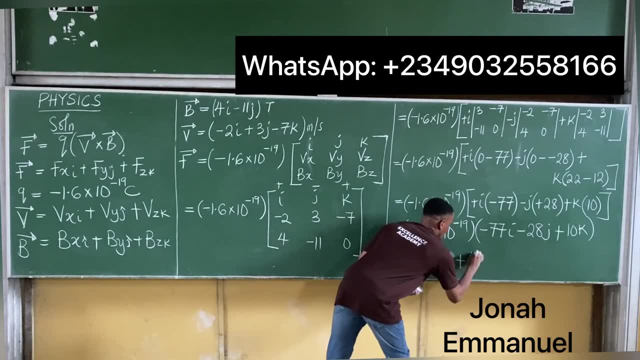 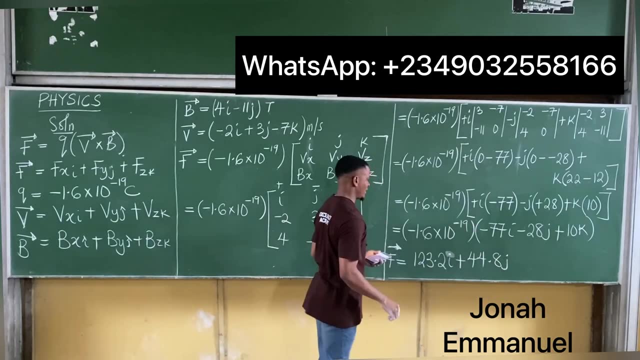 um minus 1.6 times minus 28,. that's about plus 44.8 j. and then I now have use this to multiply 10, minus 1.6 times plus 10, should give you um minus 16,, so minus 16 k. so after you're done with, 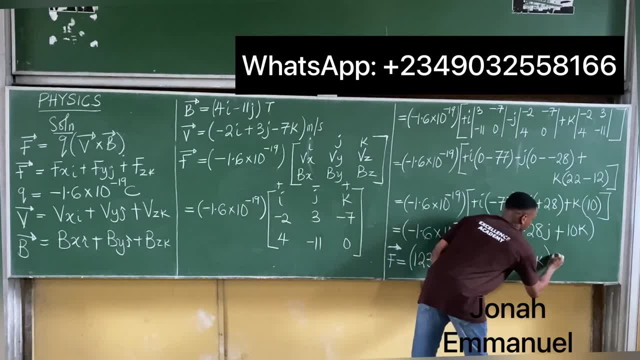 this one here. you can now bring this one here. that's times 10 to the power minus 19,. this is a force. the unit should be newton. all right, so I have this. so this is how I solve this. 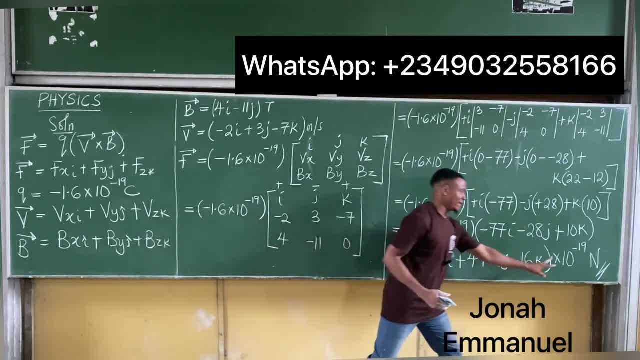 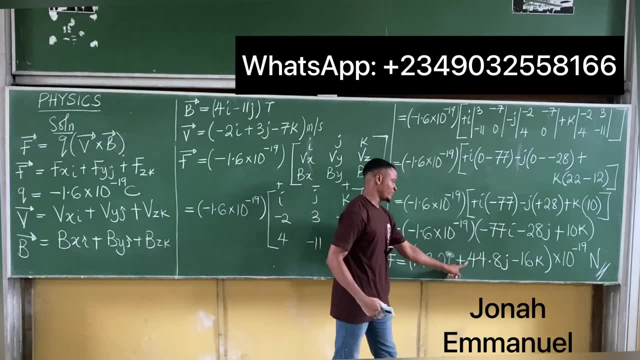 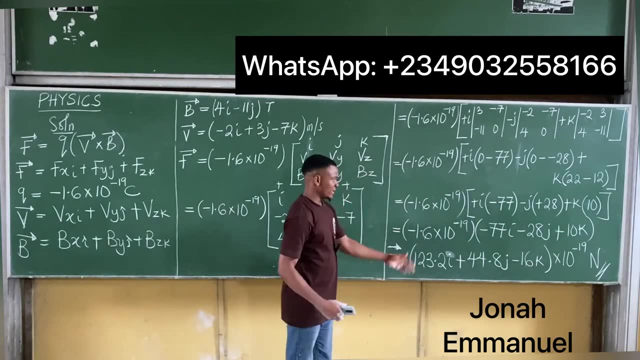 so that's the answer. so the simple idea is this: keep this one at the extreme. use this, multiply this. you have this. use this to multiply this: you have positive 44.8,. use this to multiply plus 10,. you have minus 16, and then bring this one to the extreme. the sd, the unit for force. 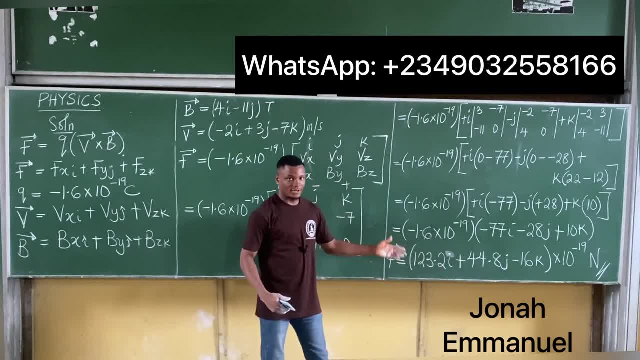 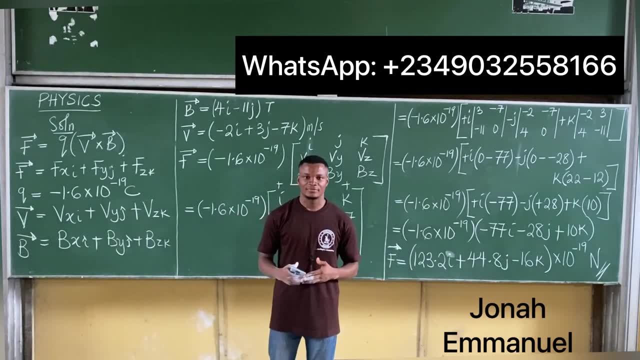 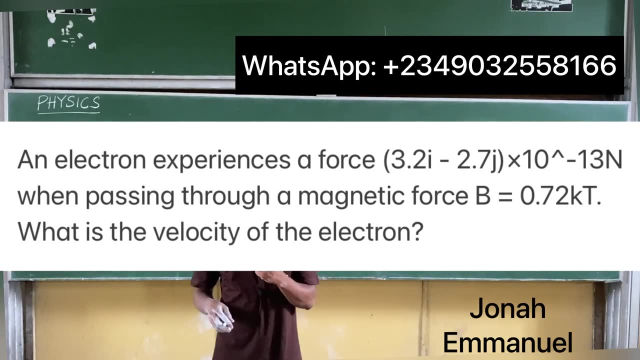 is newton, so this is my answer. so this is how I solve this question. let's try a final question. let's try another question. another question. this question says an electron experiencing force F being equal to 3.2 i minus 2.7 j. 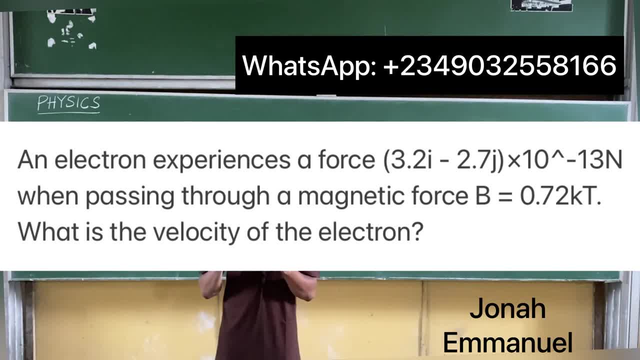 times 10 to the power minus 13 newton when passing through a magnetic field b equal to 0.72 k tesla. what is the velocity of the electron? that's the question. all right, let's get this done. 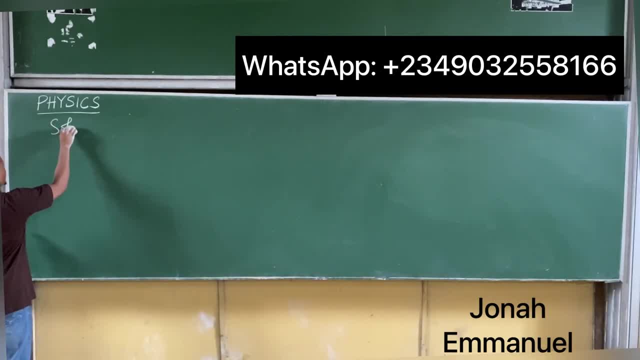 so, as usual, solution would be first of all list out given parameters. I'm giving about one there, the force in vector form. now, it's a vector force because you can see the i and j components, so I'm giving the vector. 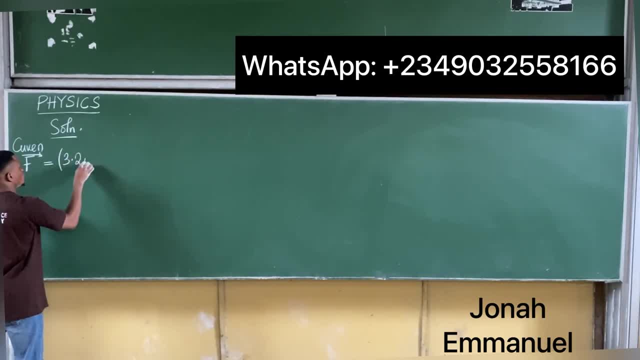 form of the force as 3.2 i minus 2.7 j. this is times 10 to the power minus 13 newton. also, I'm giving about two, the magnetic field b as equal to 0.72 k. so I have this. we're asked to find velocity. number three, I'm giving v. 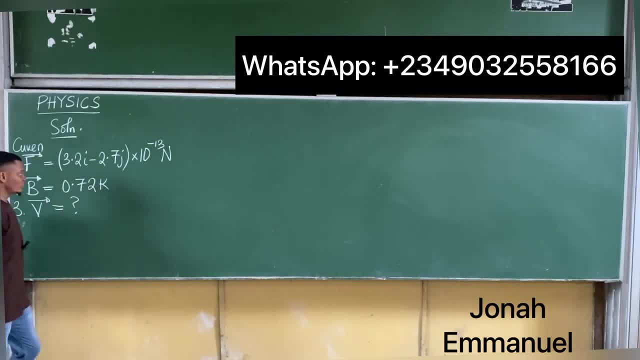 or v. I'm asked to find the value. that is unknown, so v is unknown. all right, let's get this done. and what do we know? recall formula, recall, recall our formula that's: F is equal to or in vector form, F in vector form is q into v in vector form plus b in vector form. 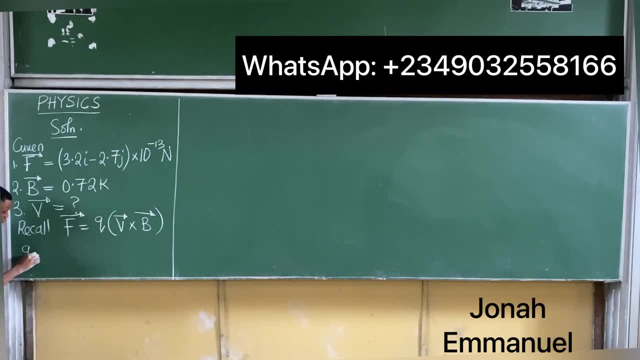 so I have this all right. what do we know? we need our q charge of an electron minus 1.6 times 10 to the power minus 19 coulomb. so I have this stuff here, all right. so what's next here? 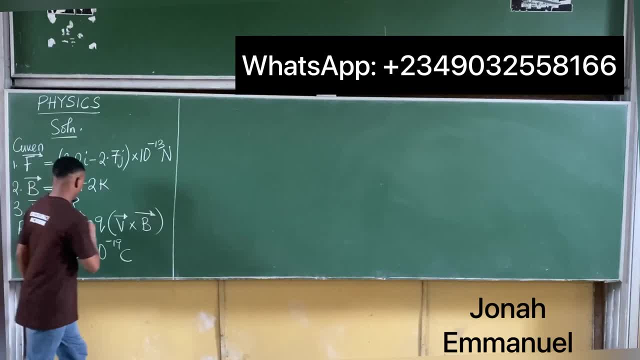 what's next here? so for v here, since we don't know the value of v, we take v as being equal to v x, i plus v y, j plus v z k. please, we are doing this because we were not giving the value of v. 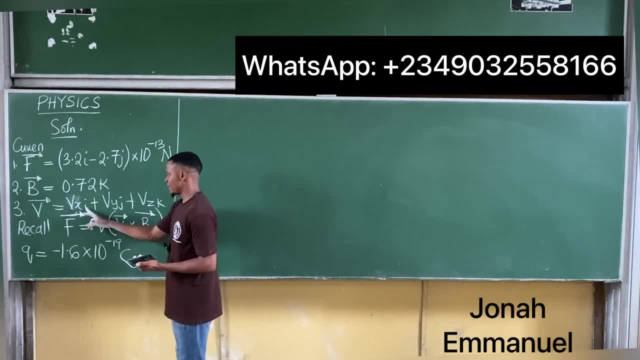 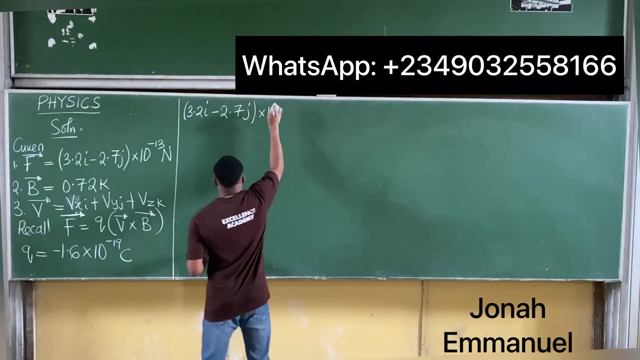 we are assuming that v will have three components. we have the i, j and k components. all right, let's get this done. so if that's true, as we did in our previous example, we have that F, this F value. that's about 3.2 i minus 2.7 j. all times 10 to the power. 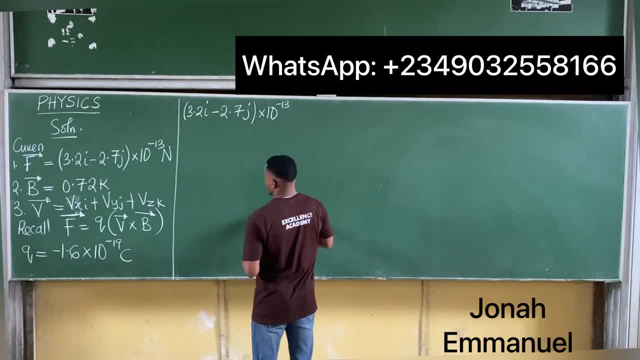 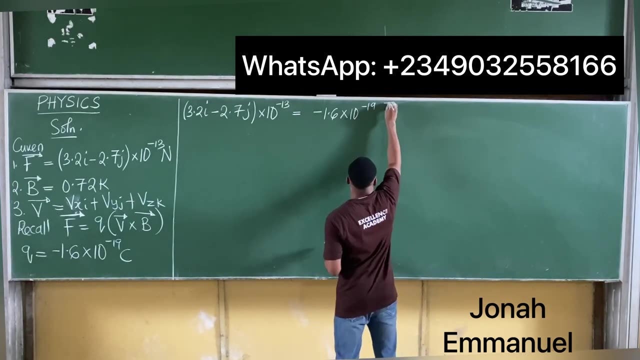 minus 13,. so that's F is being equal to q. q is minus 1.6 times 10 to the power, minus 19,. q into v cross v. let's get the vector form of v cross v my first time, so get my i. 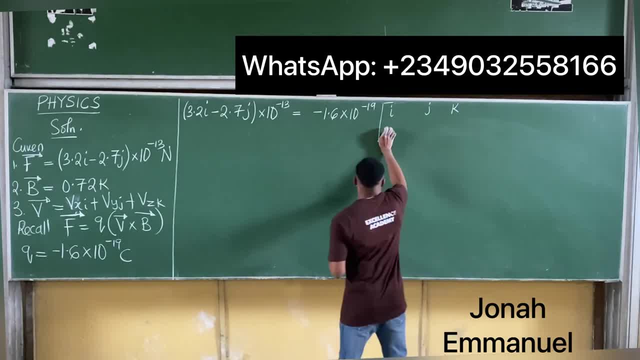 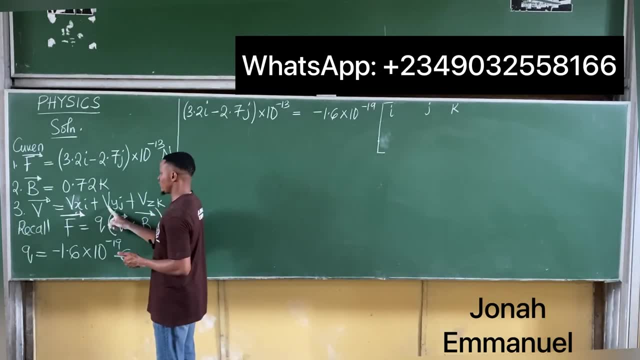 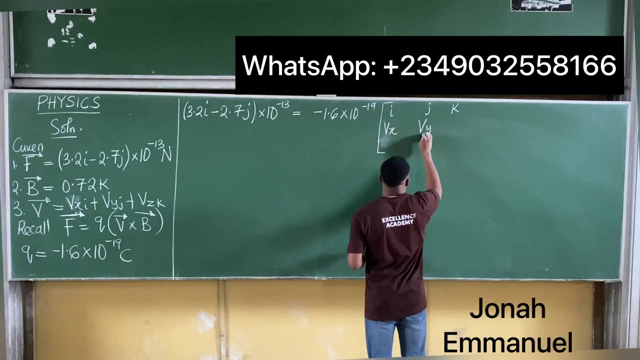 my j and my k components. so if that's true, let's look at v. for v. we don't know the value, so we'll assume it as v x, v y and v z. so for i, I have v x, for j, I have v y. for k, I have v z. 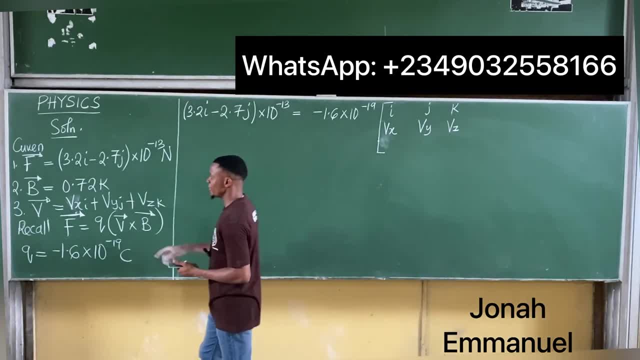 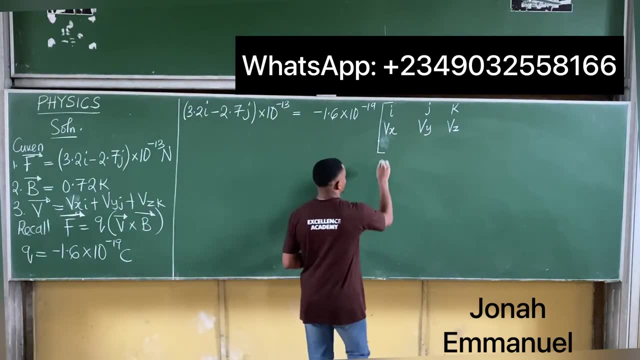 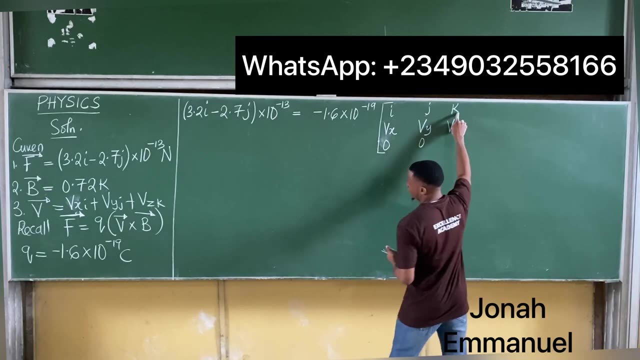 so that's your v components for b, observe that b only has a k component. there is no i, there is no j, so the. so that means: for i on that we'll have zero for okay, for j on that we'll have zero. for k, I'll now. 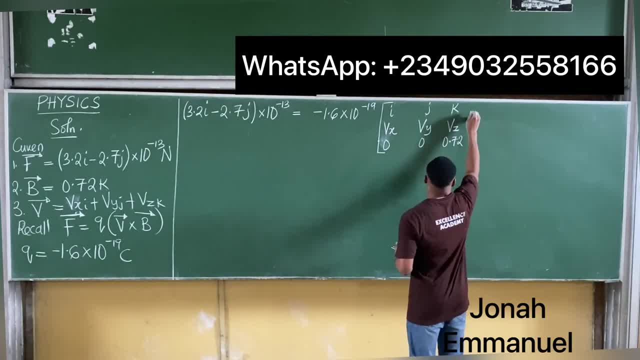 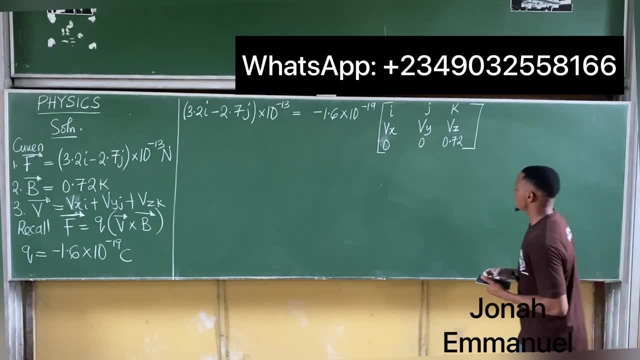 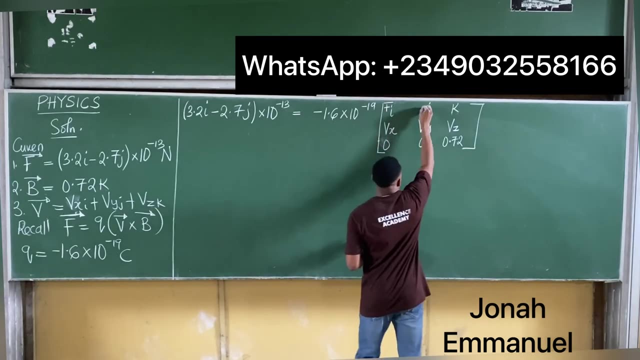 have 0.72, so I have this all right. so this is what I have. so let's solve this and see what we get. so if I solve this here, we said, in solving this one here, your first task is to add a plus, minus, plus. always this way, always that way. 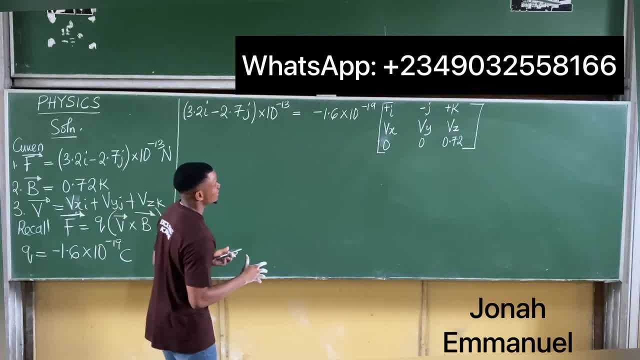 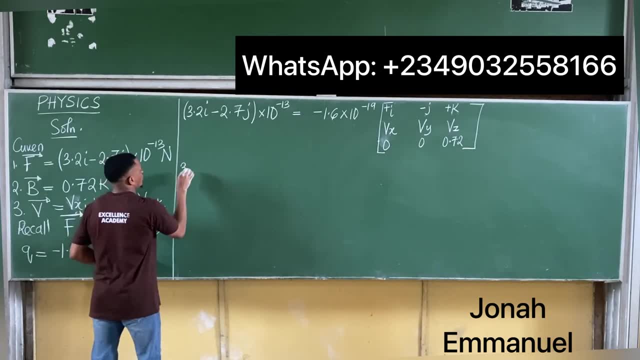 okay, if that's so, let's, let's try to expand this. if you expand this, what do you get? so this 10 comes inside. here I'm having 3.2,, 3.2 times 10 to the power, minus 13. i. 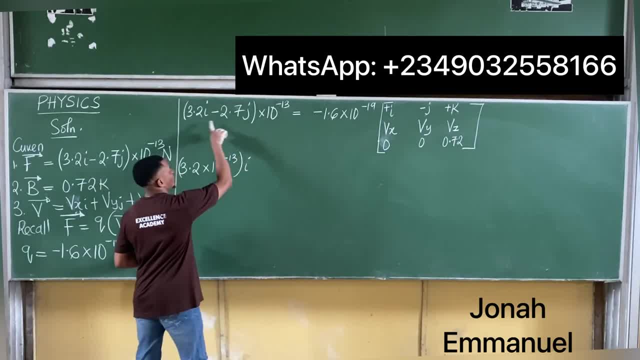 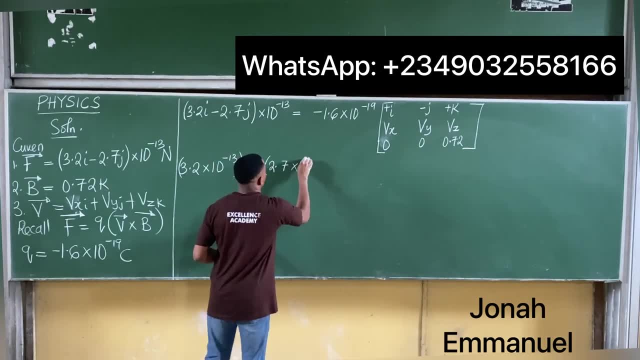 so that's the i value in full. so this one comes into here minus. so, minus this and this, I have 2.7 times 10 to the power minus 13. this j, if I have this is equal to what I have here, is minus. 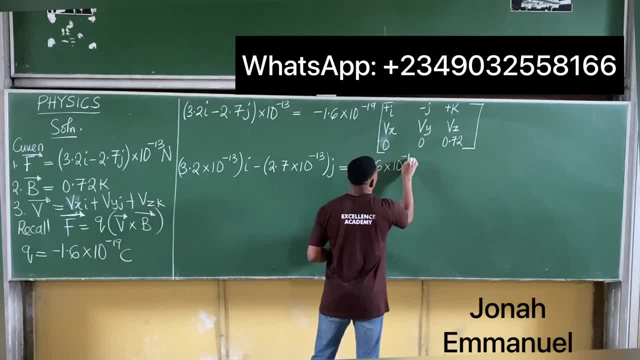 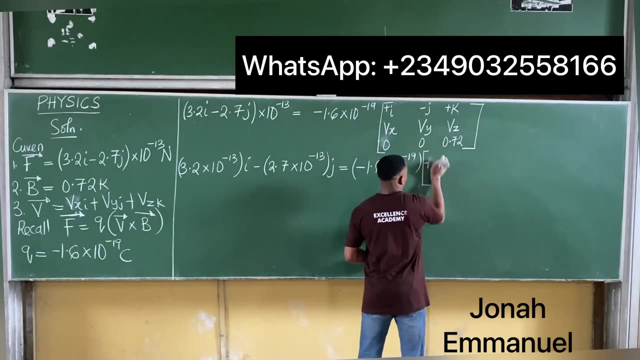 1.6 times 10 to the power minus 19,. this one here into let's get i j k, so for i becomes plus i I'm having okay, so let me use this so into into plus i. we said: get your 2 by 2 matrix, so plus i, my 2 by 2 matrix, for i here. 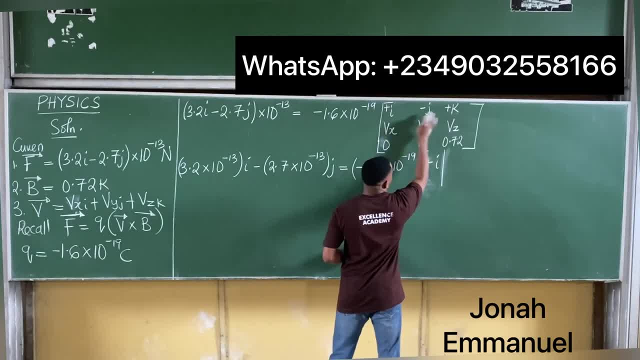 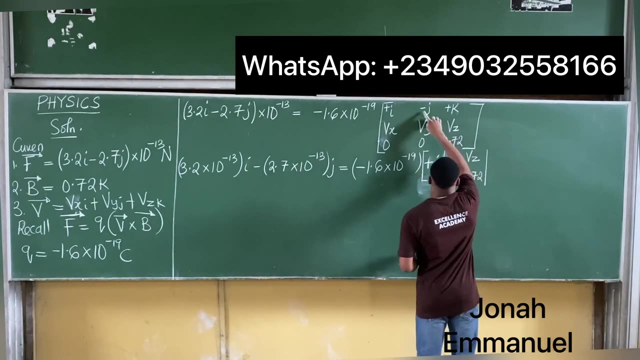 cover the row. cover the column. cover the row. cover the column. I have v y v z, so v y v z 0.72, 0.72, that's my i next one minus j, so minus j into for j. cover the row and the column. the row is of. this column is of. 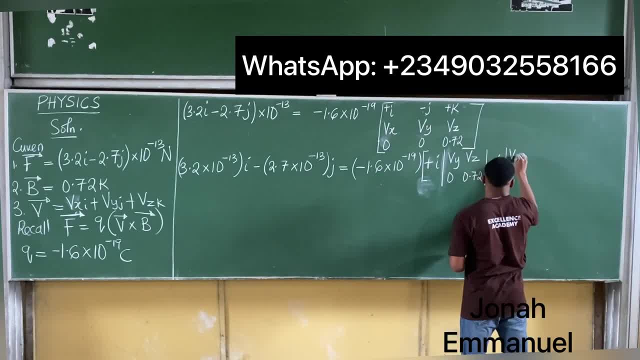 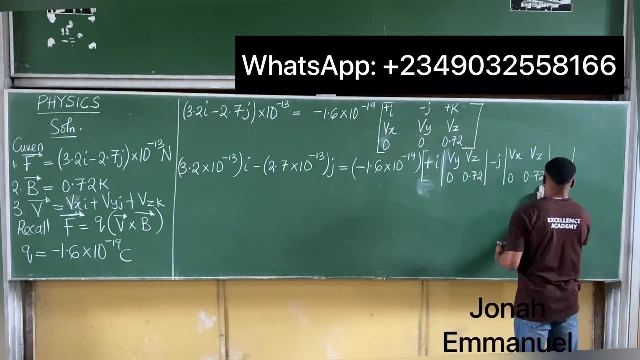 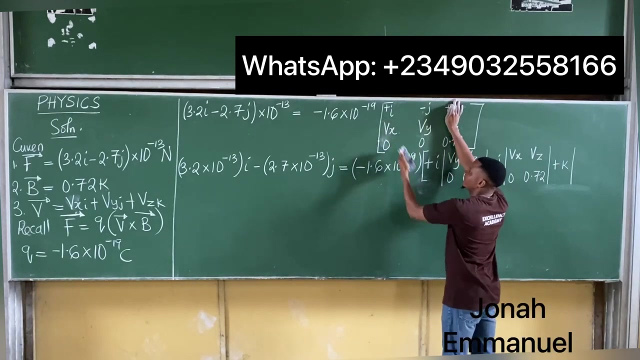 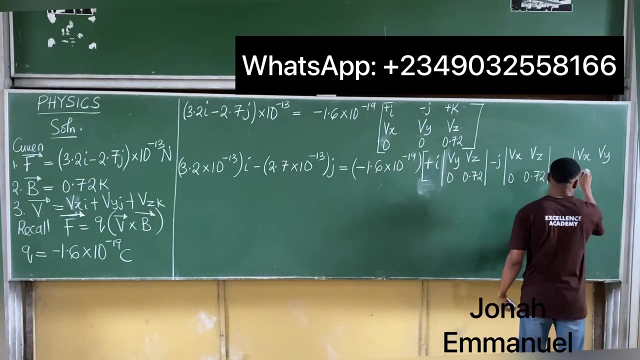 I have v x 0,, so v x 0,. v z 0.72,, v z 0.72,. finally, I have plus k. I have plus k into into plus k cover, the row and the column of k cover here and here. I have v x v y, so v x v y, 0, 0,. I have 0, 0,. 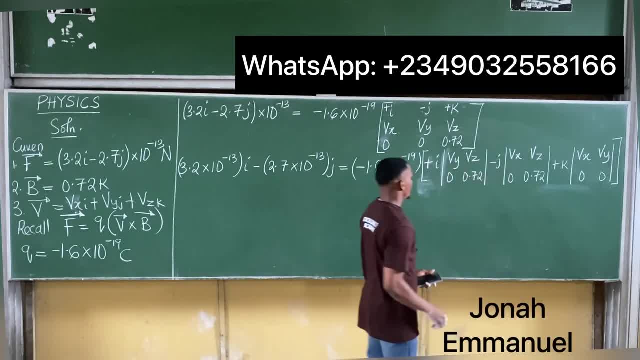 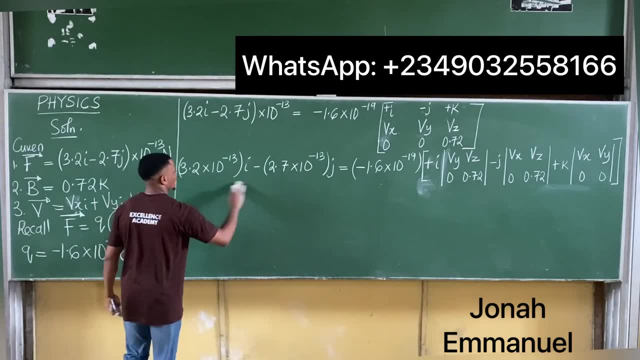 so I have this all right. so I have this case here. all right, let's expand further. what do I get? um expanding further, this one here becomes 3.2 times 10 to the power minus 15,. 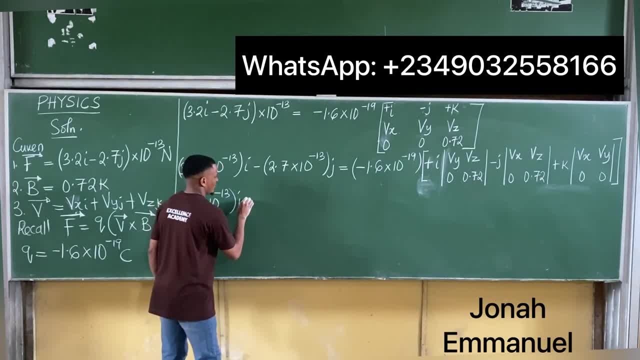 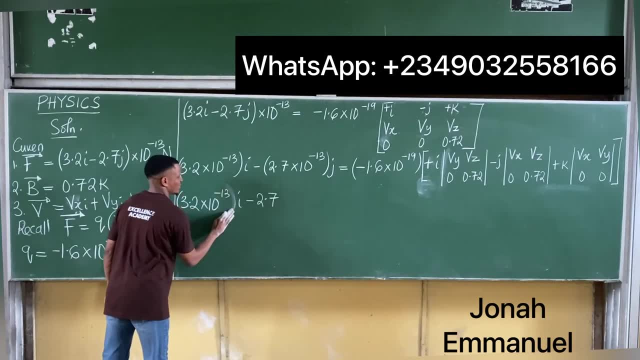 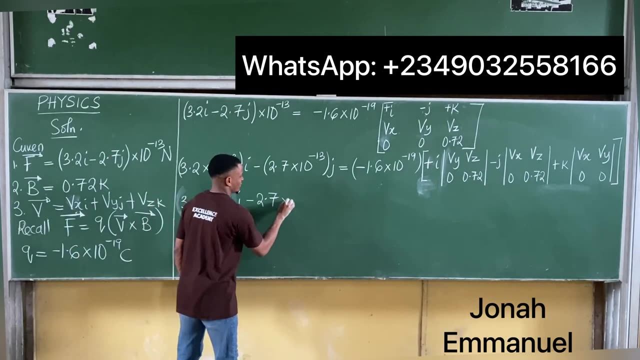 this is the i component minus into this minus 2.7, and perhaps at this point you can now take off the brackets. it's okay like this. so take off brackets now I have this. so this i minus 2.7. 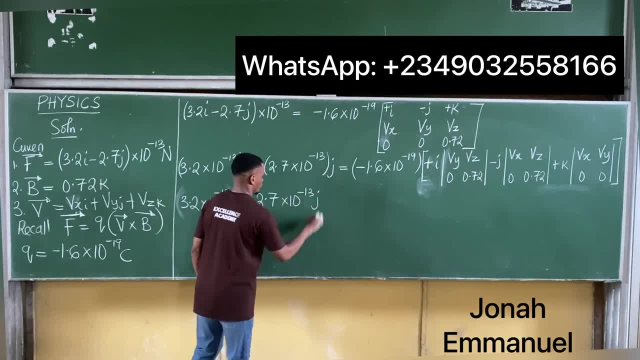 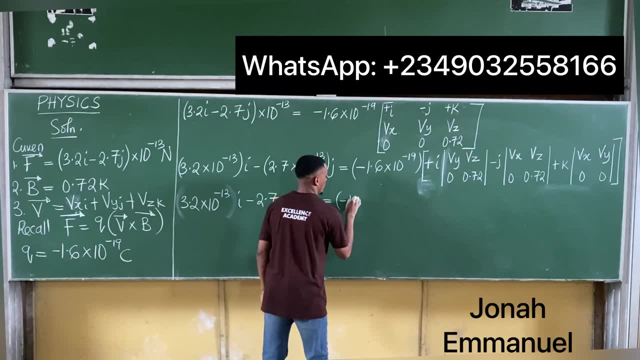 times 10 to the power, minus 13 g, if you want to, and that's equal to. I have this as minus 1.6 times 10 to the power, minus 13 g, and that's equal to: I have this as minus 1.6 times 10 to the power. 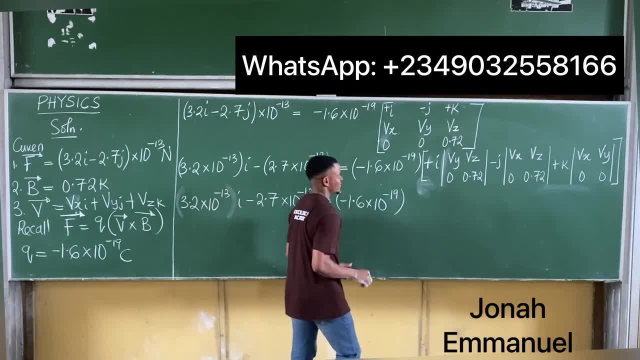 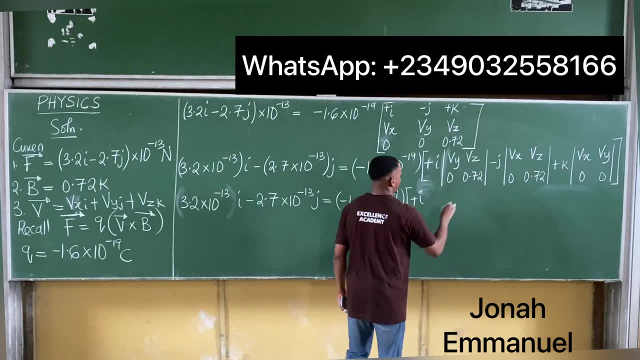 minus 19,. I have this into, for this one here I have. this is giving us plus i. so plus i multiply this, this becomes v y times 0.72, that gives you 0.72 v y. so this times v y. we said it's. 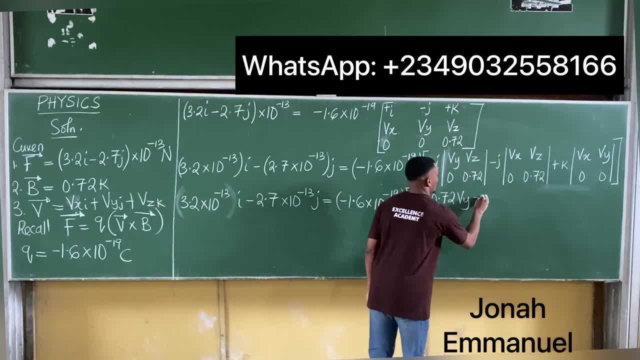 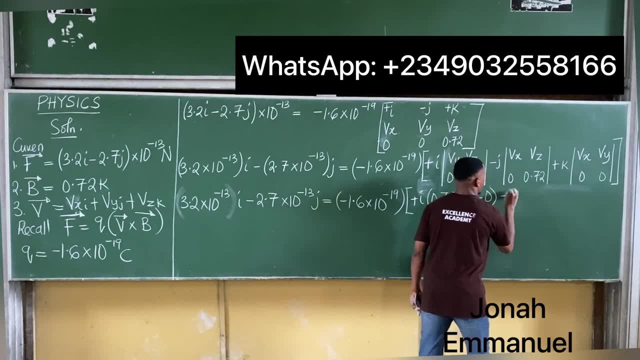 this times this, minus this times this. so minus v z times 0, gives you 0,. so this one here, let's see. so minus j into v x times this gives you 0.72 v x, so 0.72 v x next up. minus this times this. 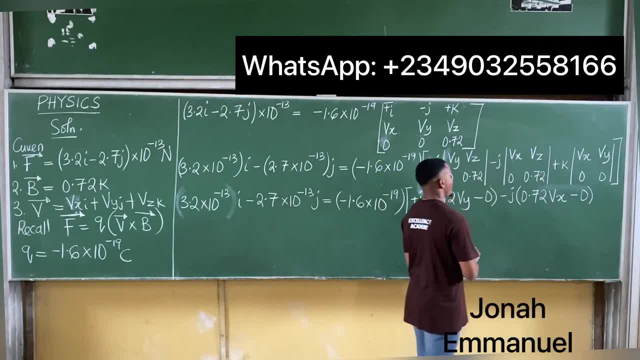 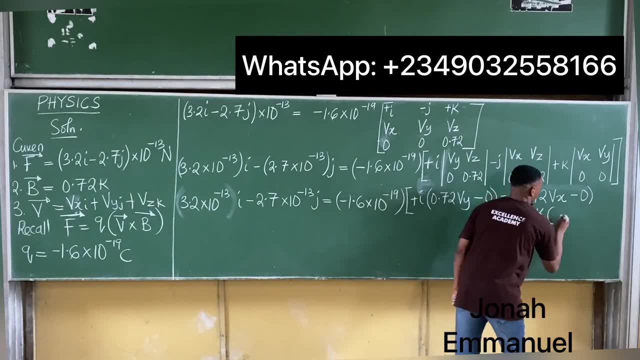 v z times 0, is 0,. so I have this. finally, I now have a plus k. so plus k into v x times 0, 0, minus v y times 0, 0, so I have. 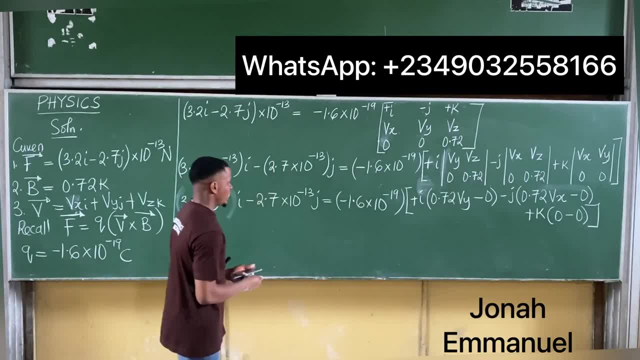 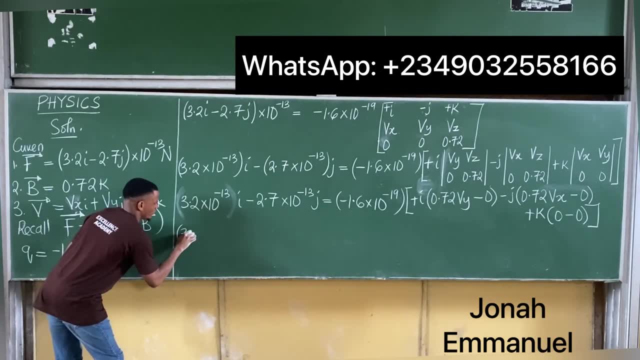 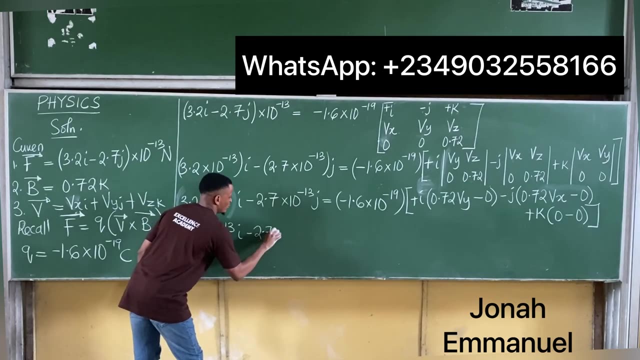 this one here, alright, so I have this case here, expanding further. I see how this is. this is 3.2, times 10 to the power minus 13 i minus 2.7, times 10 to the power minus 13 j. 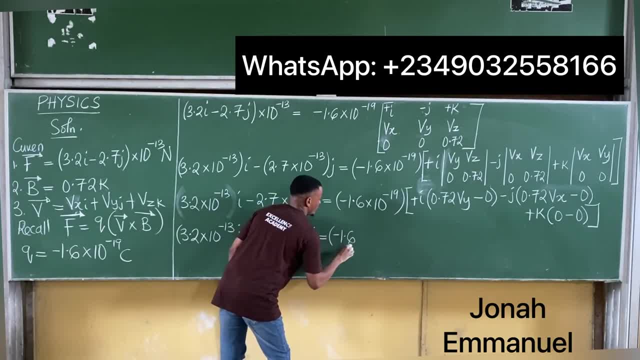 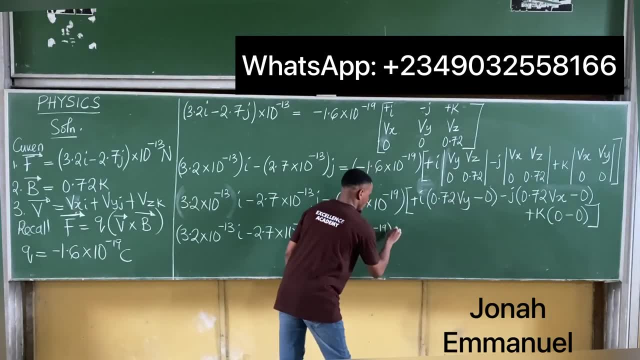 is equal to. I have this as minus 1.6, times 10 to the power, minus 19,. into, let's work this out. that will give us that's equal to plus i. into this minus this. 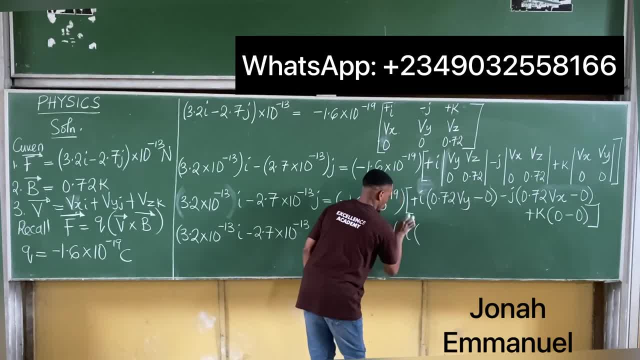 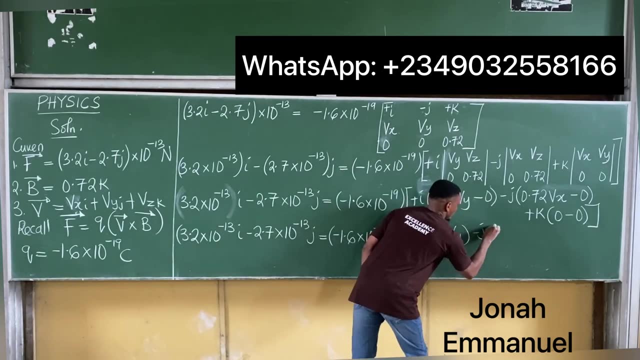 is itself, so this minus 0 is itself into. this gives you this: minus 0 is itself so 0.72 v y I have this one here, so it's off minus j. so minus j into this minus 0, is off. 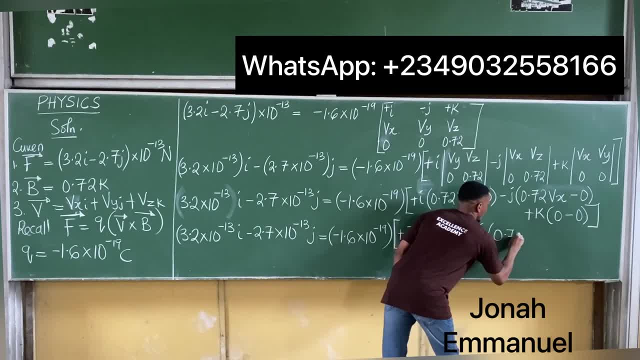 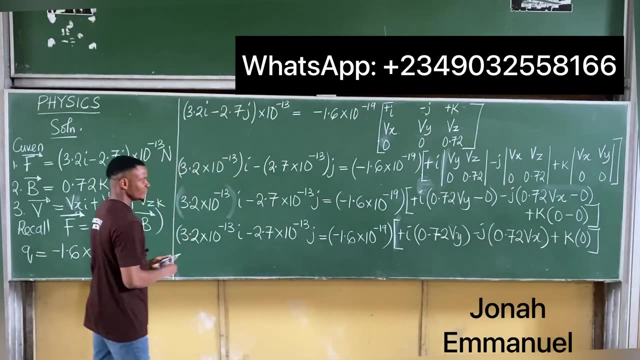 0 is off. I'm saving this: 0.72, v, x, so that's this plus k into 0, minus 0, is 0, so I have this alright. so I'll simplify the terms in the brackets. alright, I'm proceeding again. 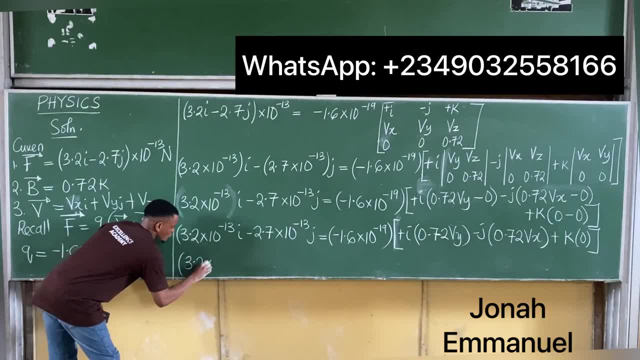 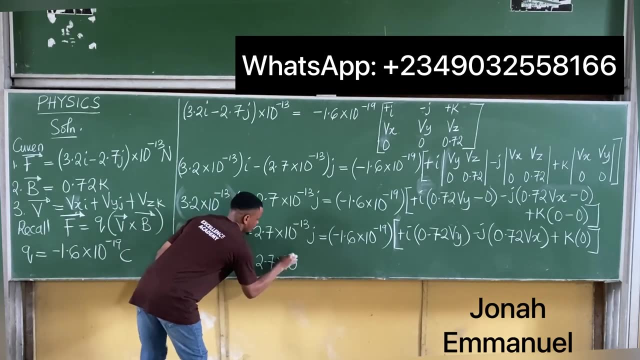 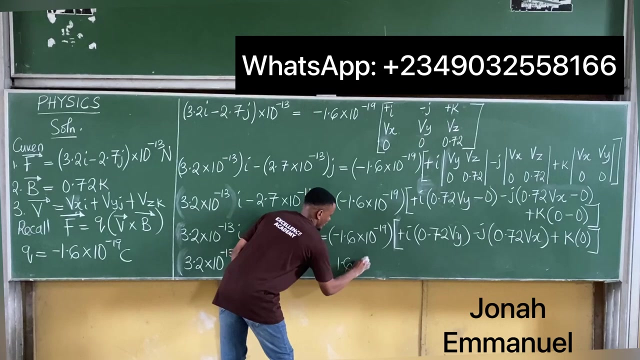 I now have this as 3.2, times 10 to the power minus 13,. i- okay, I have this minus 2.7, times 10 to the power minus 13,. j is equal to 1.6, times 10 to the power minus 19,. into for this, I have this times i. 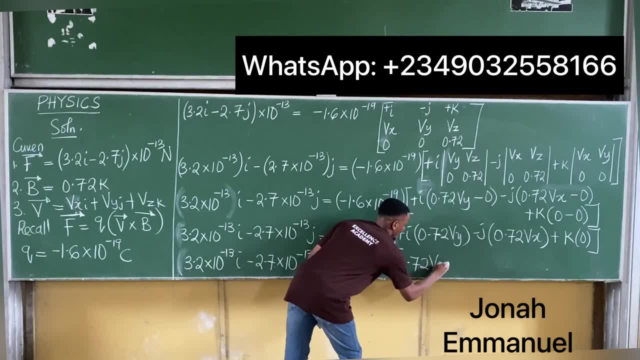 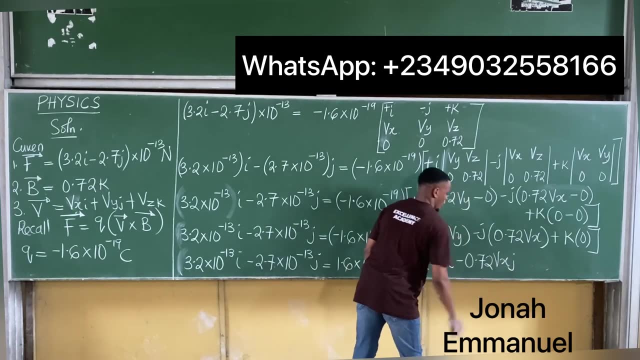 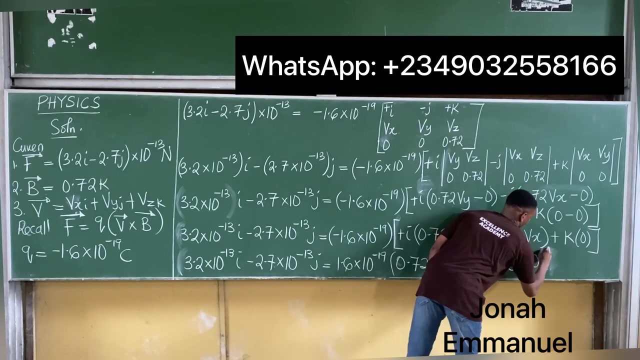 that's 0.72, v, y, i. this times i is this: come to j. this times gives you minus. so minus this and this, 0.72, v, x, j, and then plus k times 0, is 0, so it's off. now I have this okay. 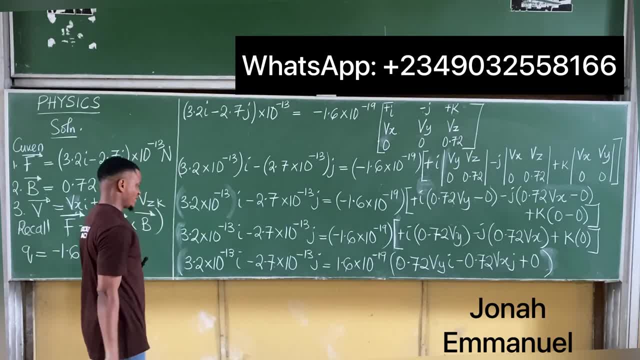 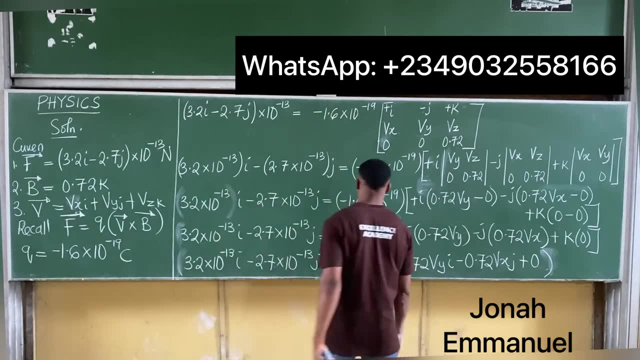 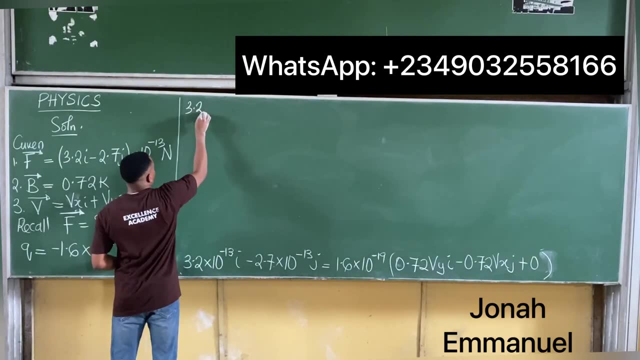 so I have this point here, alright. so what's next there? I'll have to use this to multiply, true? okay, let's take this one off. alright, let's proceed with this. so I'll have this as 3.2, times 10 to the power, minus 13,. i. 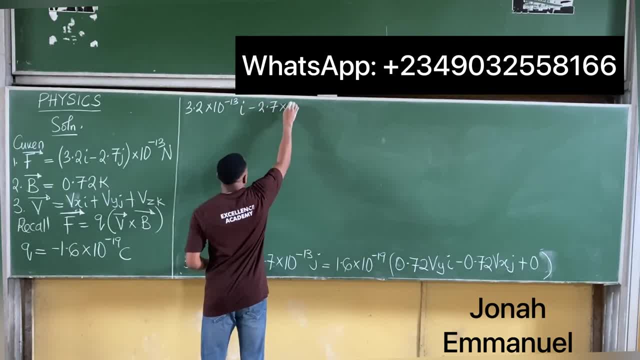 this one here, minus 2.7, times 10 to the power minus 13,. j is equal to: let's multiply these two, so I'm having this should be a minus 1.6,. please, minus 1.6,. 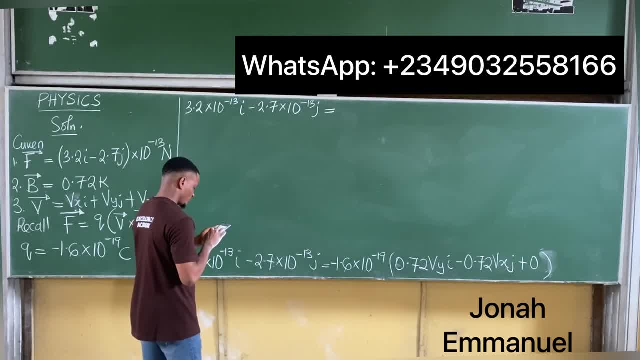 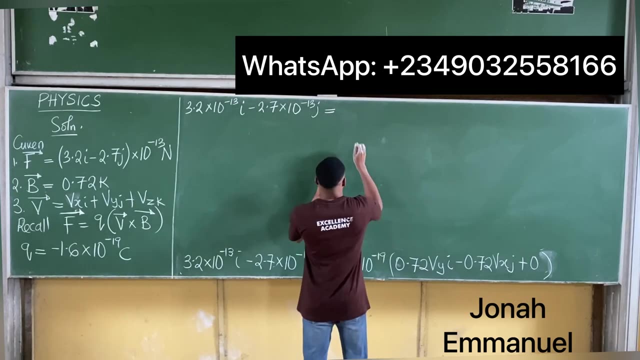 okay, that becomes minus 1.6, times 10 to the power minus 19,. multiplying 0.72, that's about minus 11.52, times 10 to the power minus 20,. bring back the v? y. 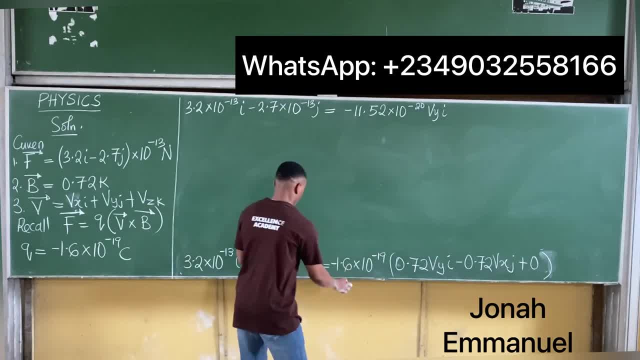 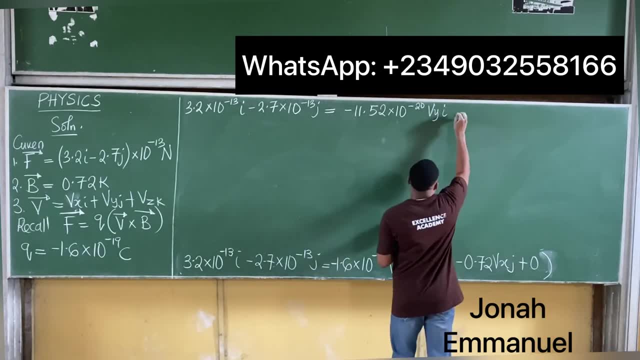 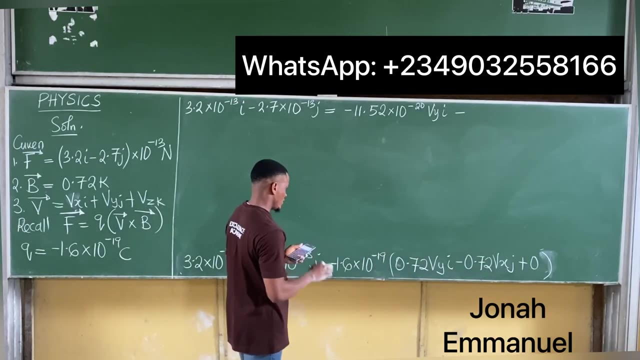 i. I have this, so this times this gives this one here. then bring back the v y i minus. let's take this into this. so that's this times. so this is just the same thing. 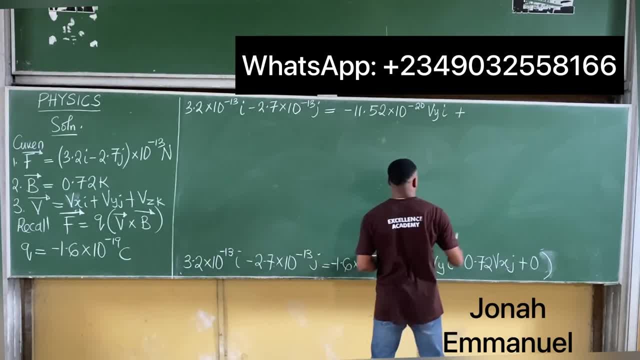 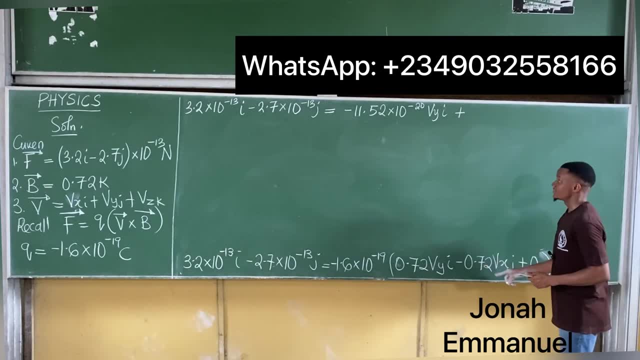 this times minus this. that should be a plus. it becomes plus this one minus 1.6, times 10 to the power minus 19,. multiplying minus 0.72, gives you plus 1.6, times 10 to the power minus 19,. 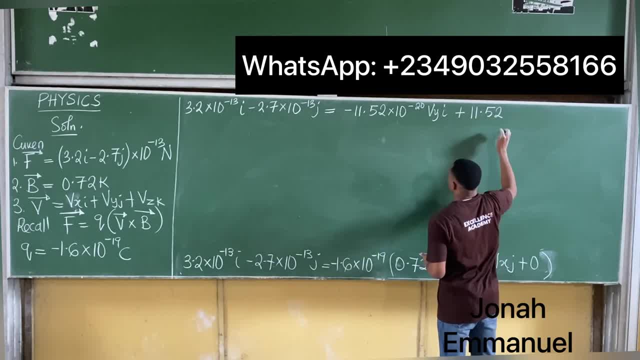 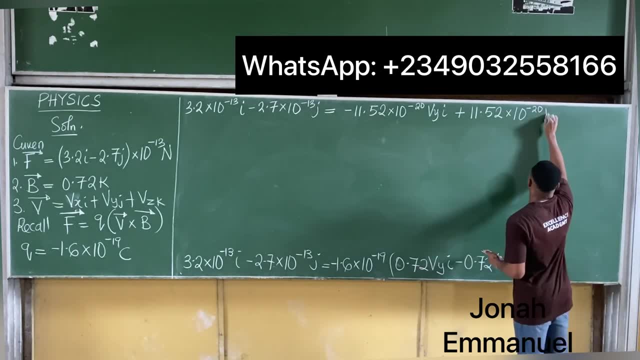 plus 11.52, times 10 to the power minus 20, into v x j, becomes v x j. so I have this, and then you have this. times 0, is 0,, so it's up. no need to include. so I'm now at this point. 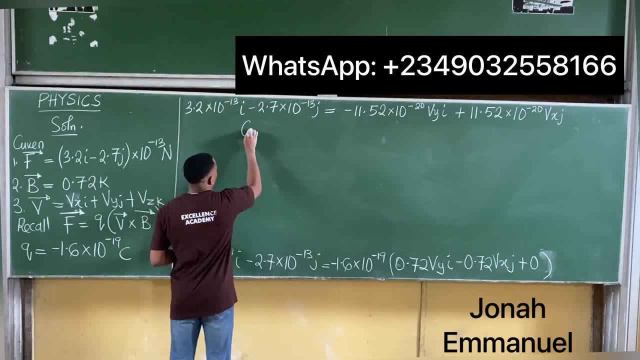 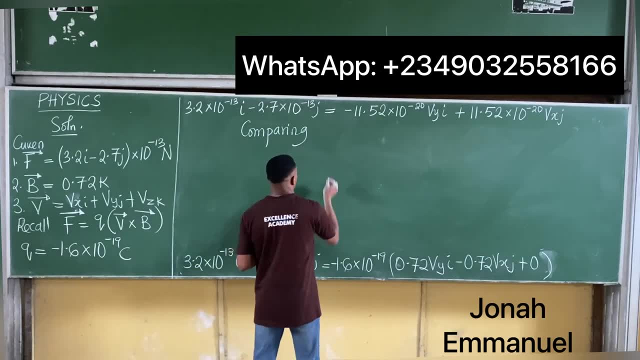 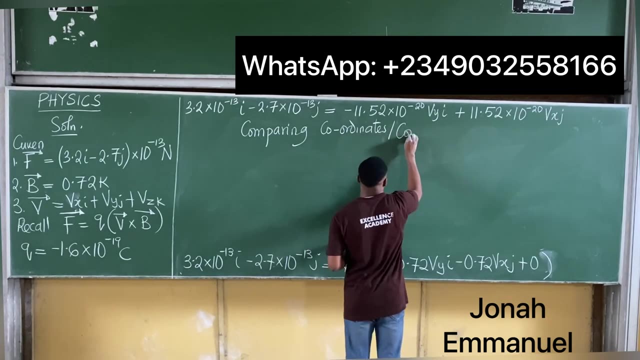 so next task, your next task here is to compare, or you can say comparing, comparing coordinates. I say coordinates or coefficients. if I compare coordinates or coefficients, let's better, as you can see, coefficients. 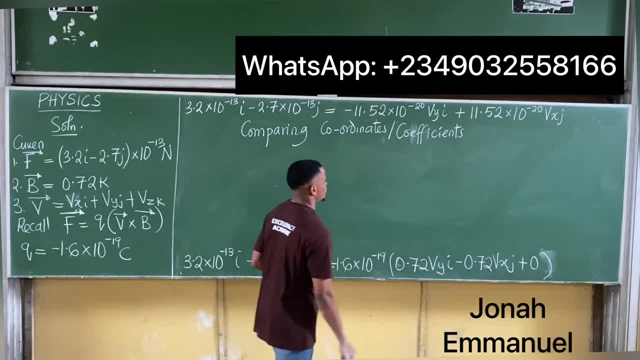 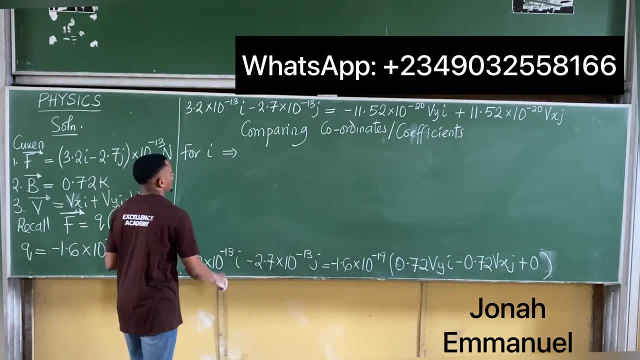 better, as you can see, compare the coordinates, or coefficients. let's start with for i, for i, for i. what do we have on the left-hand side? the i coefficients here is that 3.2, times 10 to the power. 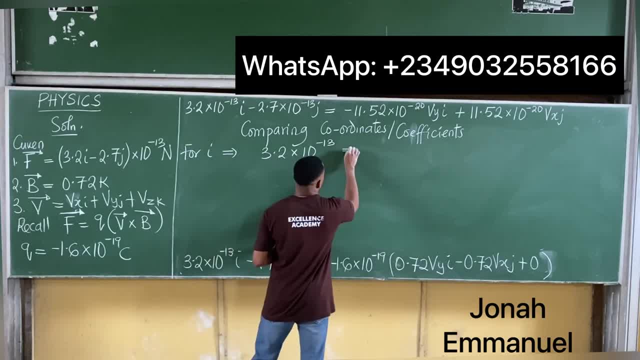 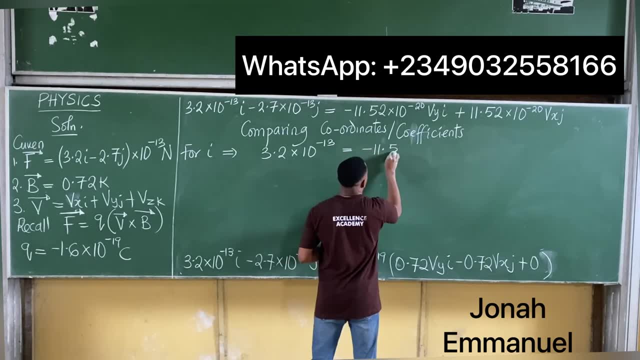 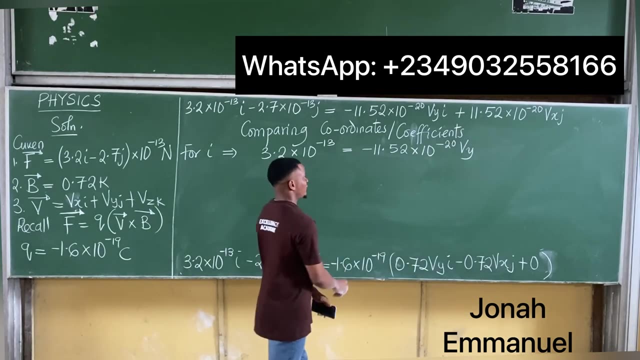 minus 13 is equal to. for the right hand side of the equation here, the I coefficient is minus 11.52 times 10 to the power minus 20 Vy. so I have this right if I compare I to I here. the coefficient here should be equal to the. 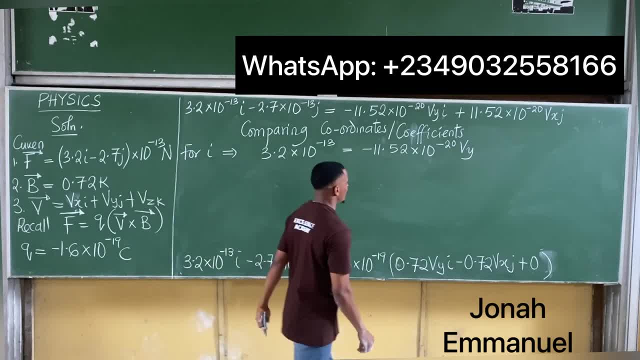 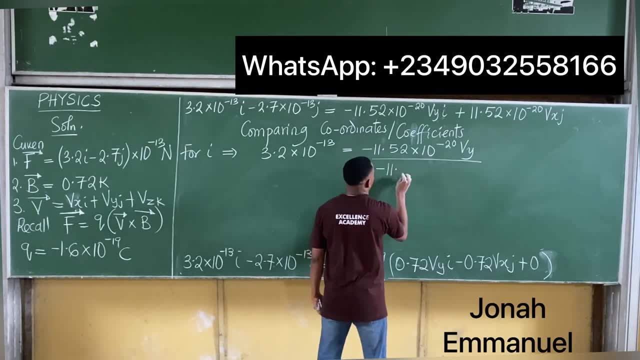 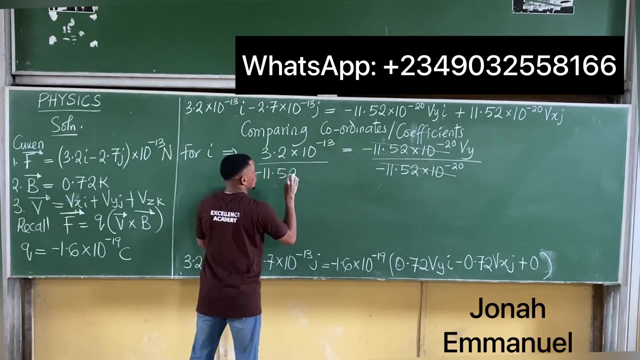 one here. so I have this from here: we can get Vy to get Vy. we simply divide here by what's attached to Vy, which is minus 11.52 times 10 to the power minus 20. so this one here cancels this divide, here too by the same thing, minus 11.52 times. 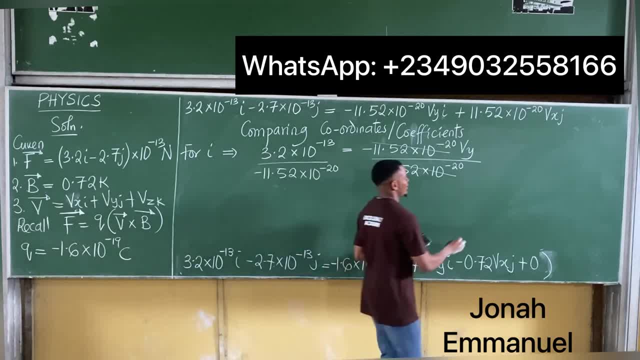 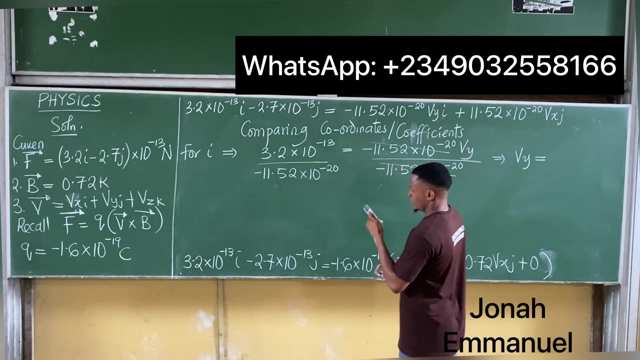 10 to the power minus 20. from here we can now note that Vy is equal to. let me get this division here. from here I have 3.2 times 10 to the power minus 13, all over minus 11.52 times 10 to the power minus 20. 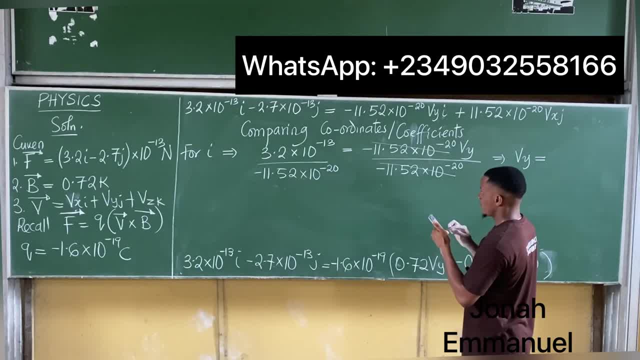 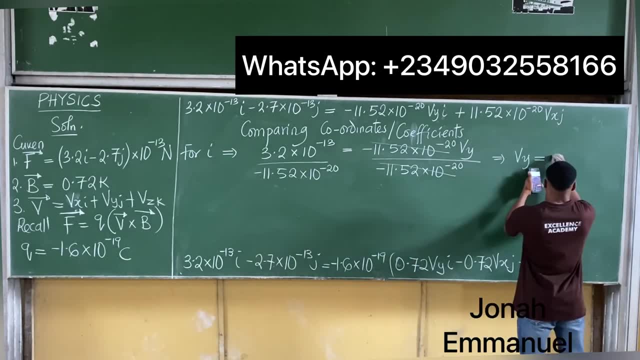 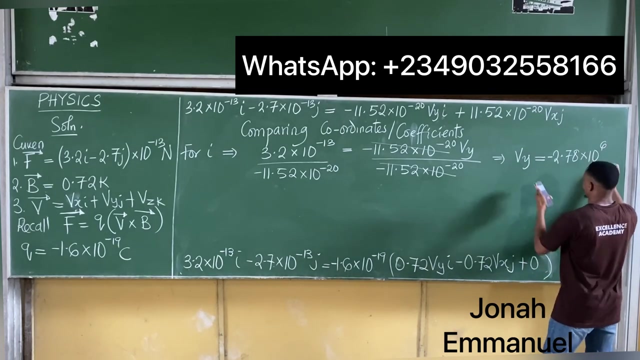 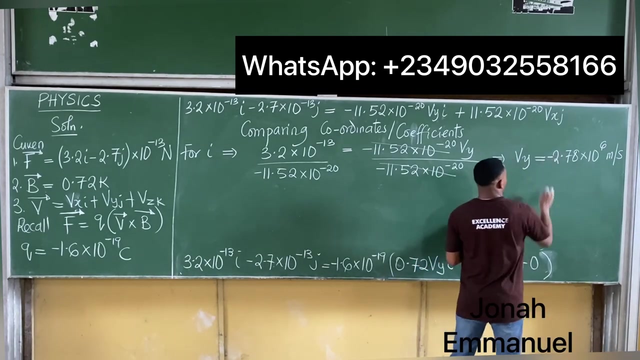 okay, all right. so this is about equal to 2.78 minus 2.78 point seven, eight approximately times ten to power. from here I'm having a one, two, three, four, five, six, think six. this should be velocity meter per second. I have this. that's minus two point seven eight times ten to power six. I'm just 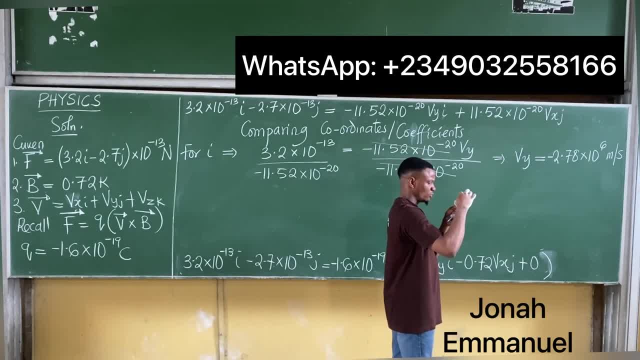 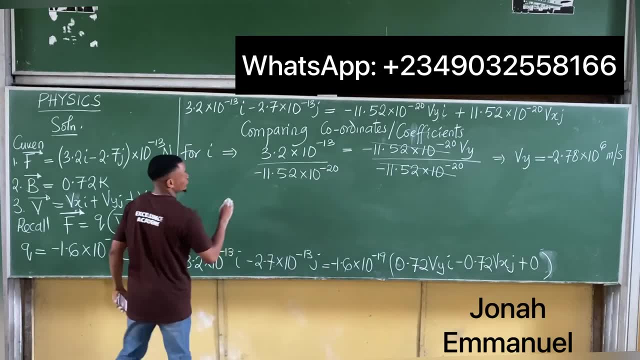 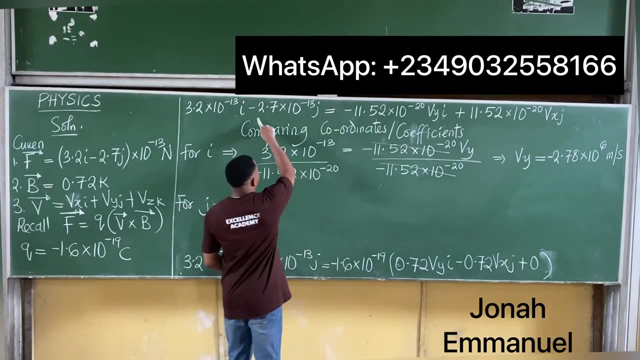 trying to confirm that from here, one, two, three, four, five, six. alright, I think this will do also. let's look up for J. for J, what do you have for the J component I have on my left hand side of the equation. my J component is minus two. 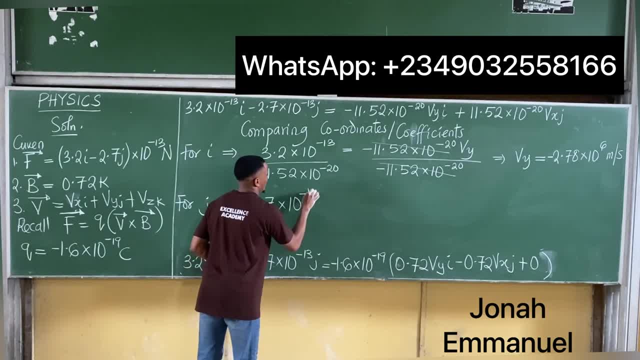 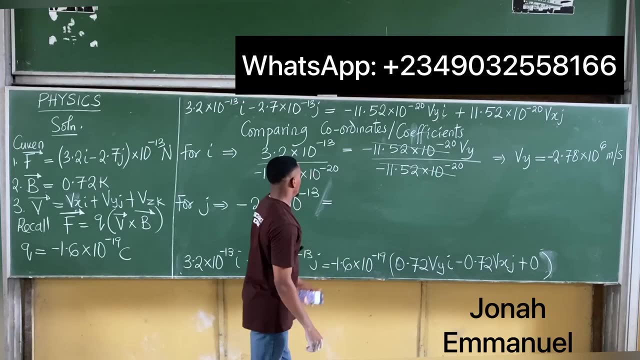 point seven times ten to power minus thirteen J or minus thirteen, that's ignoring the J- is equal to: for my right hand side, the J component here is eleven point five two. that's eleven point five, two. so five two times ten to power minus twenty Vx, so Vx. so I have this one here, alright. so of course, to get Vx I'll 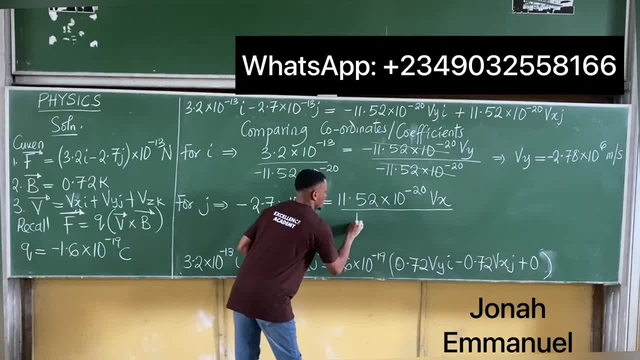 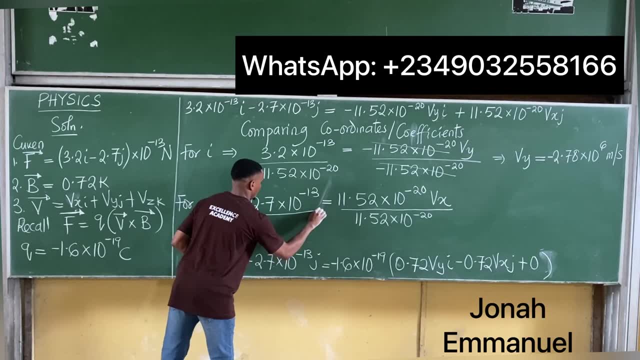 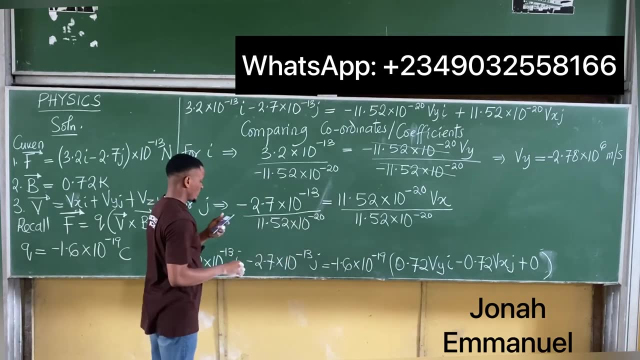 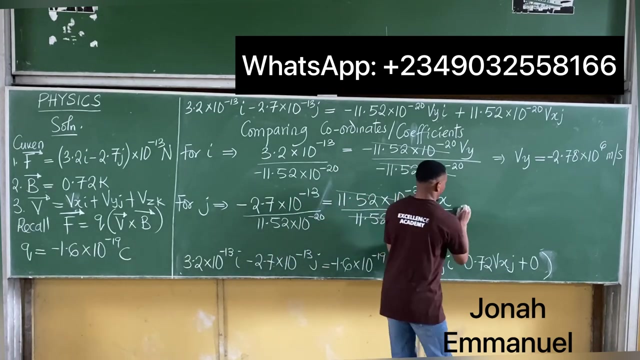 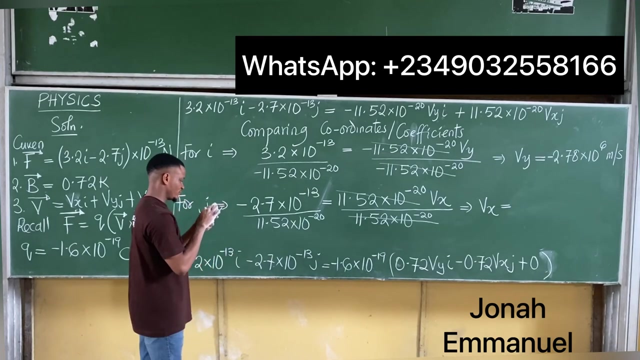 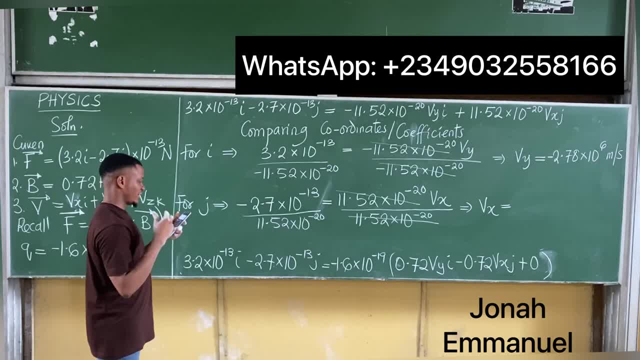 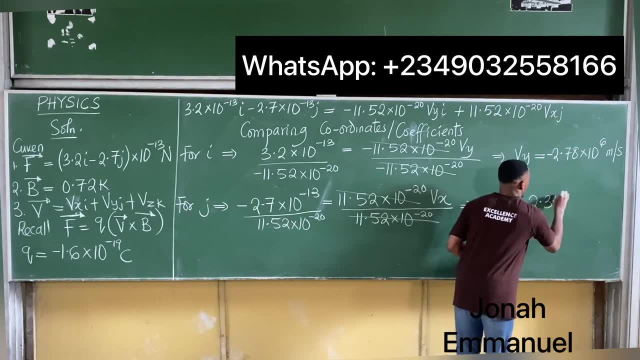 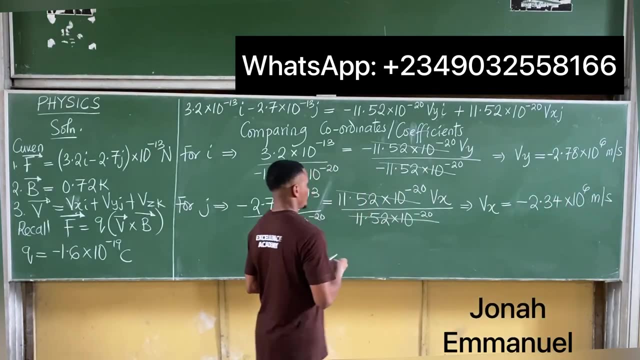 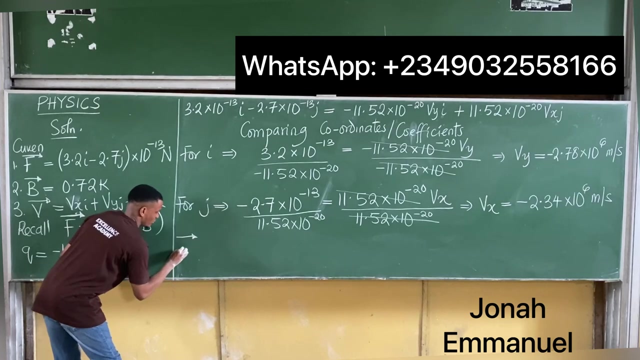 all over eleven point five, two times to the power twenty. so this gives about minus two point three four times ten to power six in meters per second. so I have this alright. so if that's so, therefore, we can now get our V, the velocity we have to look for. so therefore we can now say that V is equal to Vxi. so my Vx is this one. 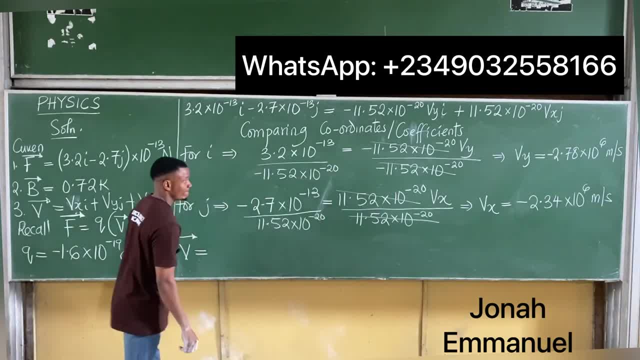 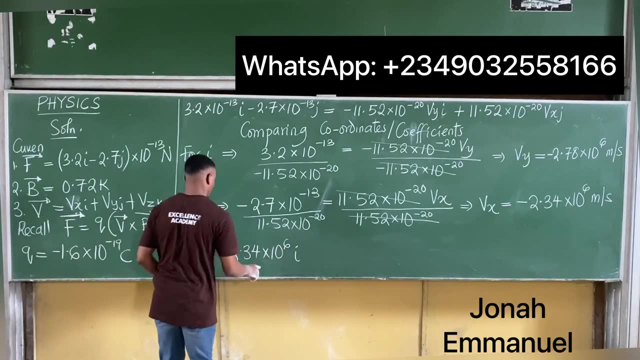 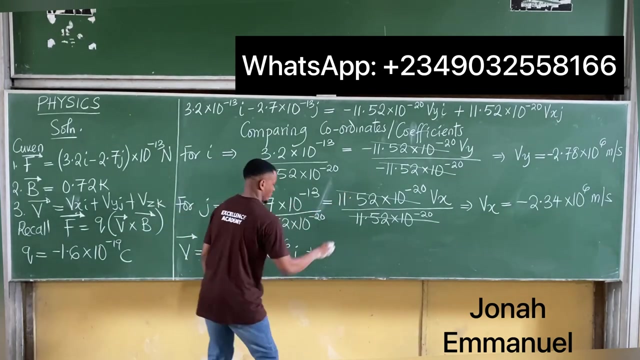 here. that becomes. that becomes, let's say, minus two point three, four times ten to power six. so here is Vx, inside Vx, and I. so this, I, this Vx, and then I plus. next becomes Vy Vy. is that one there? that's becomes Vy Vy. is that one there, that's? 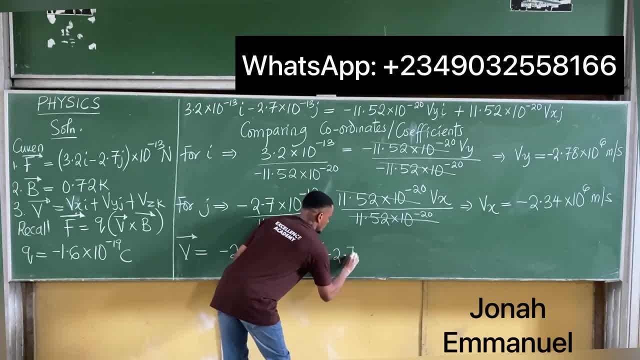 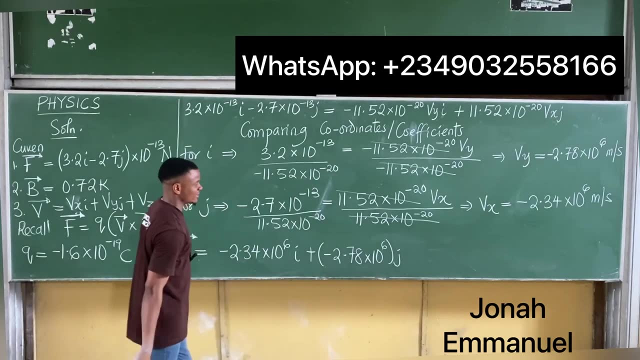 about minus two point seven, eight times about minus two point seven, eight times ten, to power six, so Vy and then J. alright, so Vx, I plus Vy, J. there is no Vz or zero, so it's off alright. so here's my answer. all of this should be in meter per. 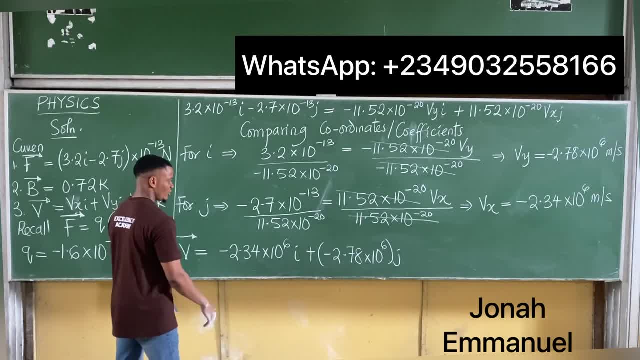 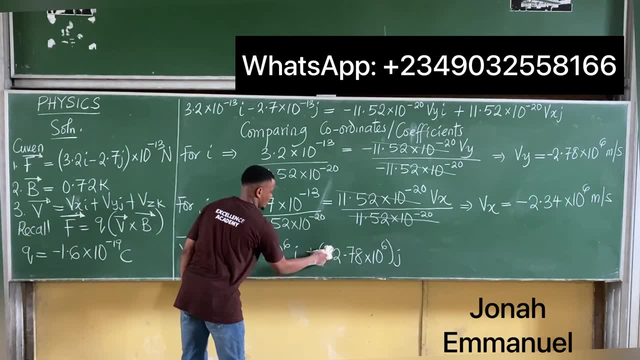 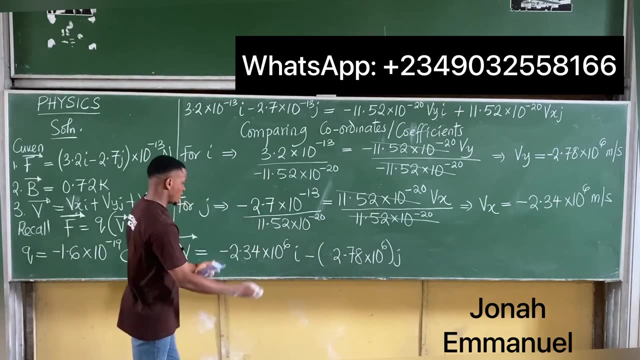 second, but I know I can still factorize this, of course, factorizing. I have plus times minus, which is minus, so this one here is off, so that's a plus, minus is minus, so becomes mine loss all of this. so that's basically simply. let's featureize this by factorizing. I am picking the term. 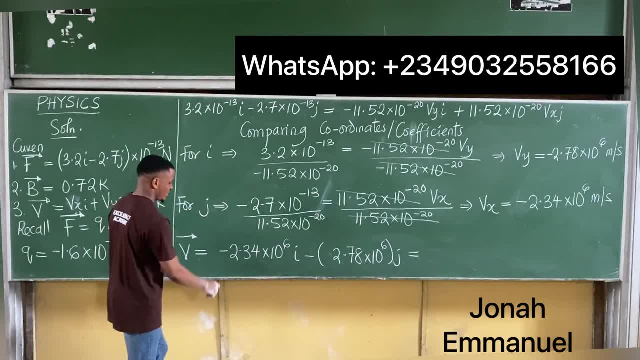 come on on both sides. on both that I can see in miners and it mines they'll bring minus outside, so minus into also. on both both of this I can see 10 to the power 6, 10 to the power 6, I'll take it to the extreme so if I take off, 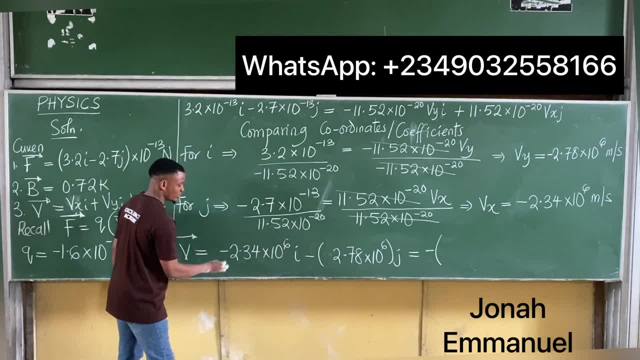 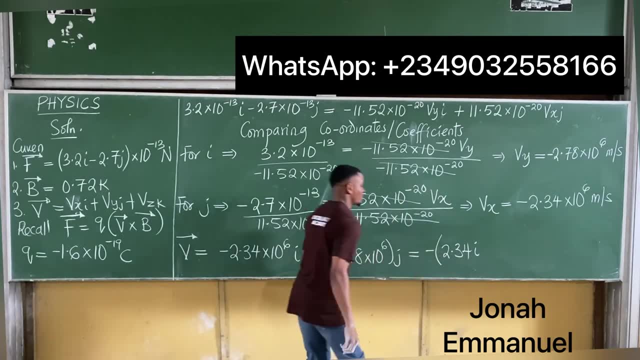 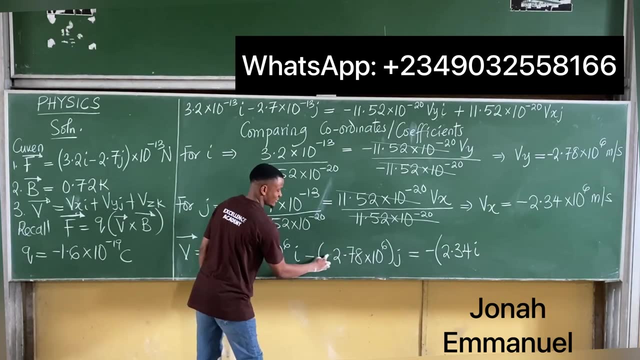 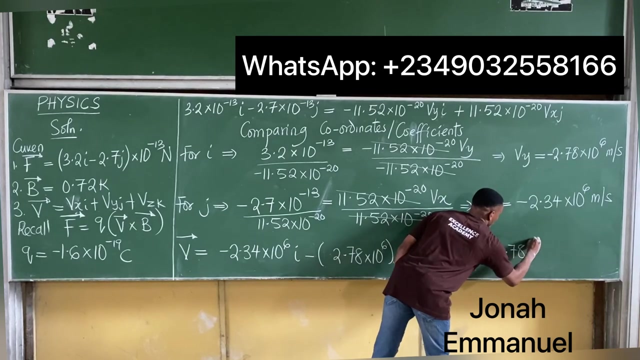 minus and then 10 to the power 6, I'm left with 2.34i. that becomes 2.34i next up. if I take off minus and 10 to the power 6, I'm left with plus 2.78j. so plus 2.78j. so I have this so minus. 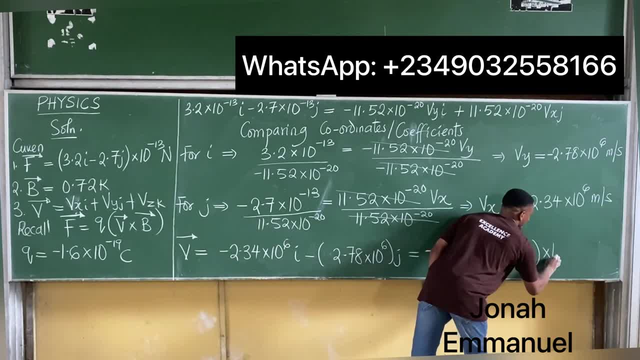 this, and then, of course, times 10 to the power 6, so I have this. all of this should be in meters per second, because I'm calculating velocity. all right, so this is how I solve this equation. so this becomes: 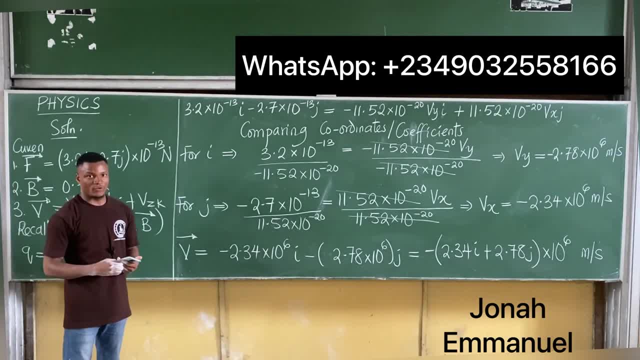 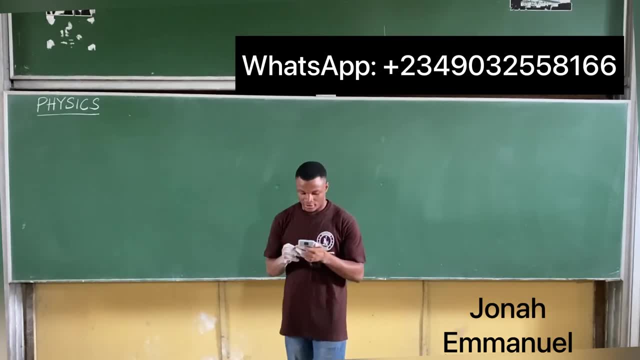 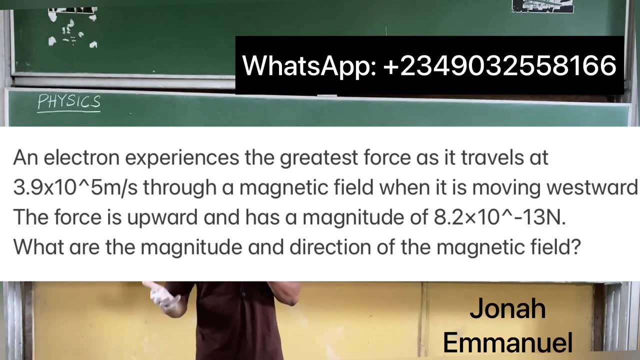 the velocity we are asked to look for. so this is how we solve this particular question. all right, let's try one final question on this. all right? so this question says an electron experiences the greatest force as it travels at 3.9 times 10 to the power 5. 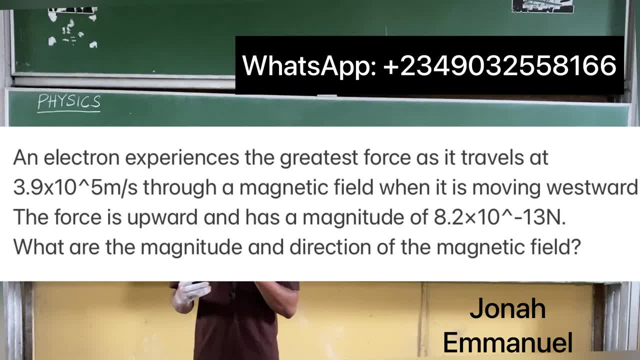 meters per second through a magnetic field when it is moving westward full stop. the force is upward and has a magnitude of 8.2 times 10 to the power minus 13 newton full stop. what are the magnitude and direction of the magnetic field? all right, let's get this done. 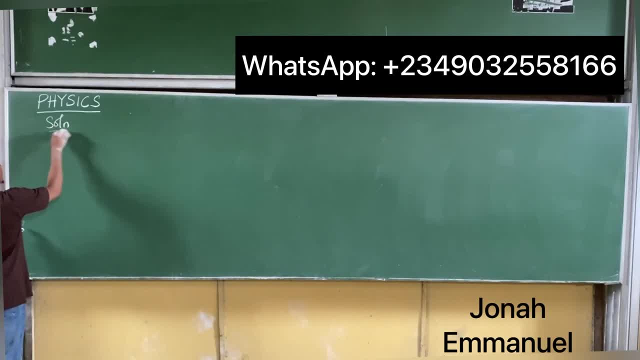 please. so solution um solution, quest tax, as usual, list out given parameter, so given number one um what I have. they said it travels at 3.9 times 10 to the power, 5 meters per second. 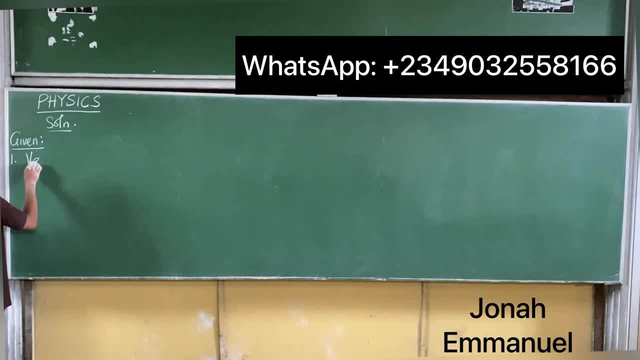 that's velocity. so velocity that's v is equal to 3.9 times 10, to the power 5 meters per second, they said, through a magnetic field. when it is moving westward the force is upward and has a magnitude. so next up is force um, force f. the magnitude is about, let's. 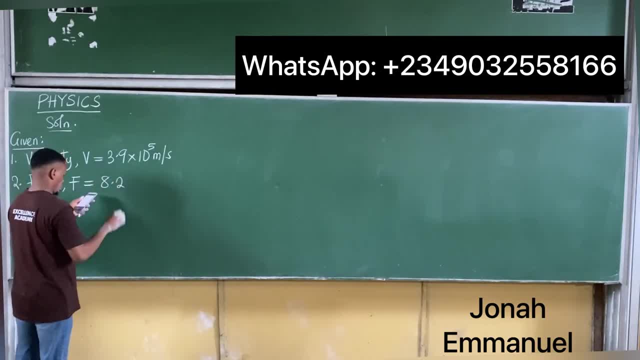 say about 8.2 times 10 to the power minus 13 newton. okay, what are the magnitude and direction of the magnetic force? all right, so these are the things I'm giving there. um, let's recall formula. we said f is equal to 4, for an electron or a charge in a magnetic field, f is equal to qvb. 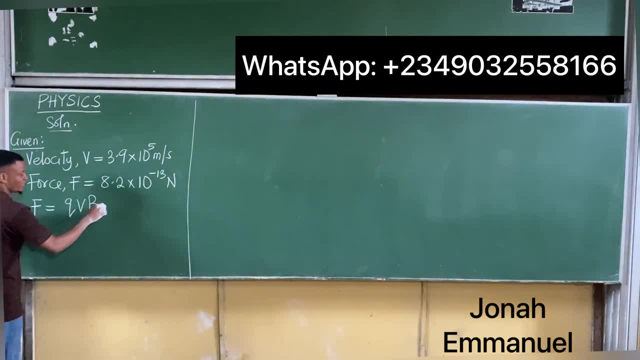 but they said the maximum force. so for maximum force, this should be sine theta. we said for maximum force, theta is 90 degrees. for this one here, that means um, if they tell you that the maximum or the greatest force experienced. so for the greatest force to be experienced, that means: 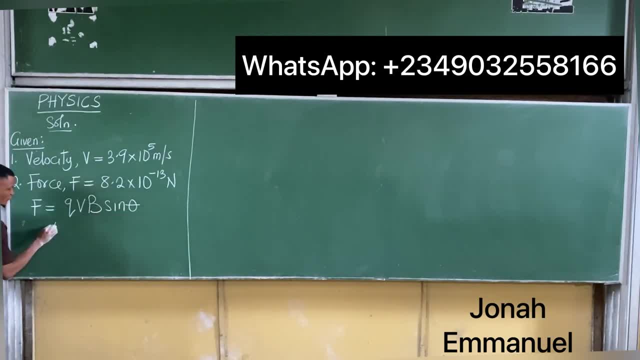 theta has to be 90 degrees, as I explained earlier. so for here theta is equal to 90 degrees, or you can choose to just keep it if you want to. so I have this. um, so we have to find. b, so we have to find. 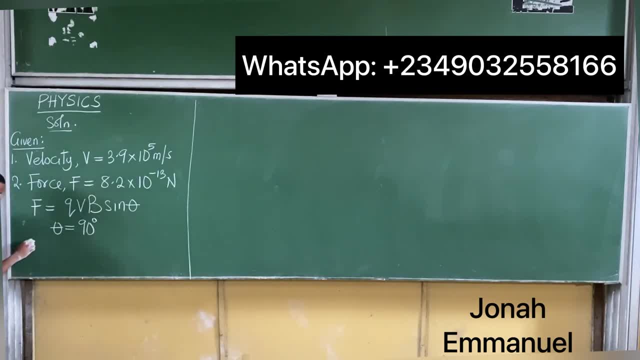 what is the magnitude and direction of the magnetic field? so b is equal to unknown. we know that q on its own is equal to minus 1.6, that's equal to um minus 1.6 times 10 to the. 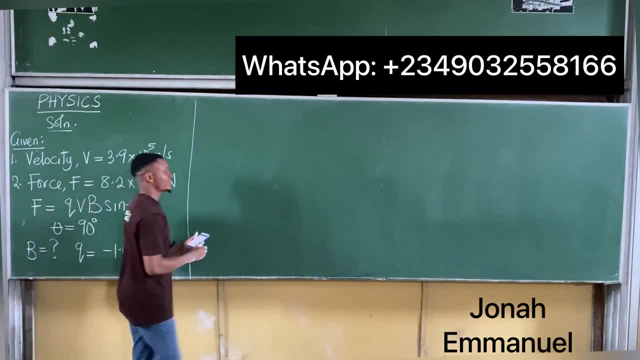 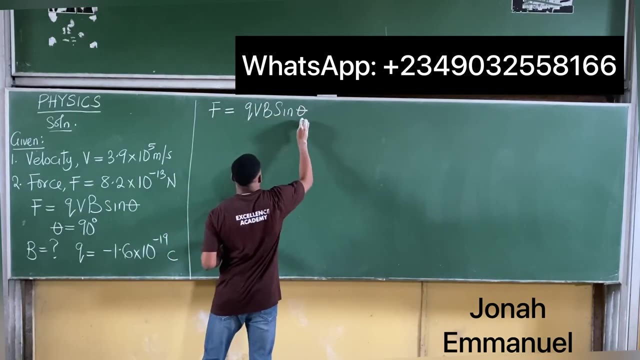 power minus 19 coulomb. so we have this all right. let us substitute values. so what do we have there? all right. so from here, if you have that f is equal to q v, b sine theta or sine 90, to get b here, divide by q v sine theta. 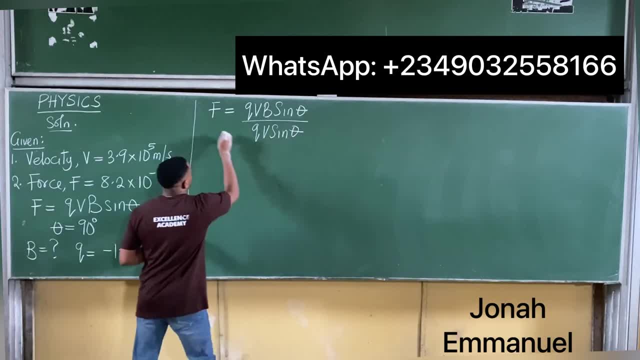 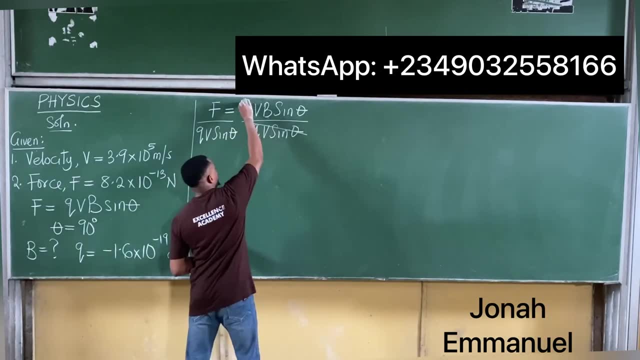 divide by q v sine theta. divide here by q v sine theta. q v sine theta will cancel q v and then sine theta. so it means that b is now equal to f all over q v sine. 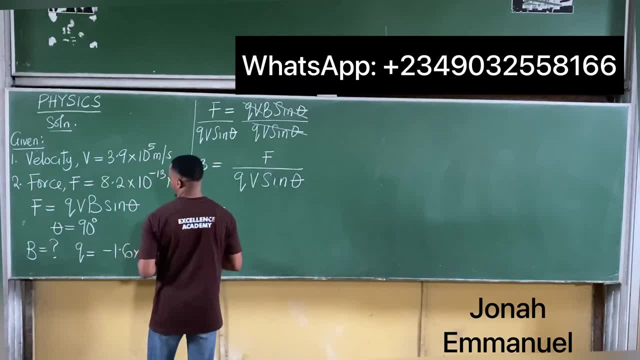 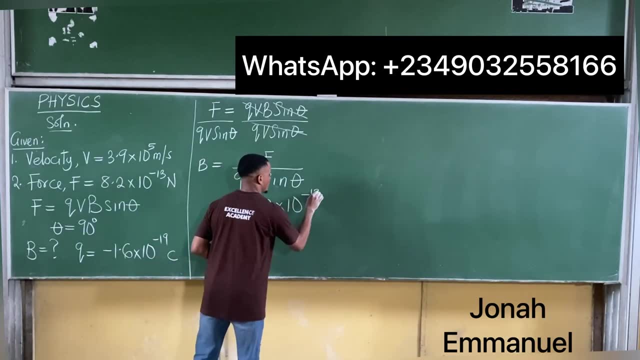 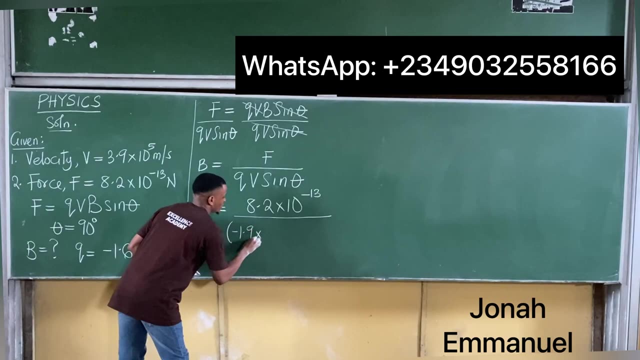 of theta, and that's equal to f, is about 8.2 times 10 to the power minus 13,. all over q, this one here, minus 1.9 times 10 to the power, 1.6 times 10 to the power minus 19, times v, v is. 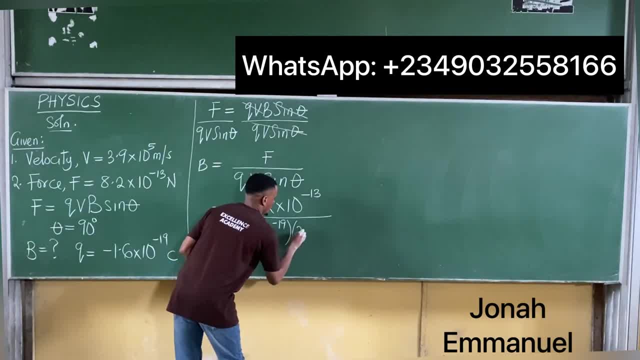 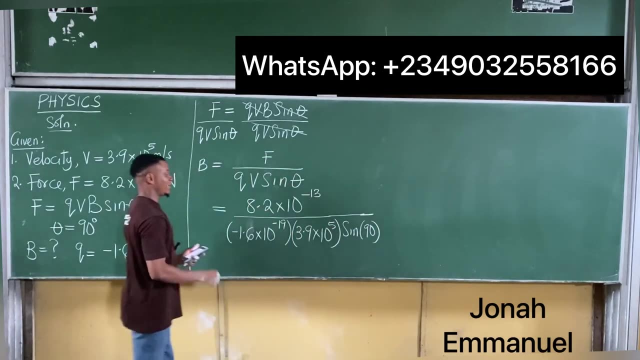 this one here, 3.9 times 10 to the power 5, then sine theta that becomes sine theta will be 90, why is theta 90, we said because they said the greatest force. so we said for greatest force or for maximum force. 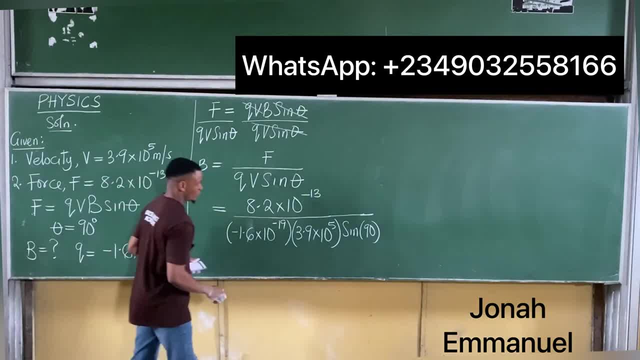 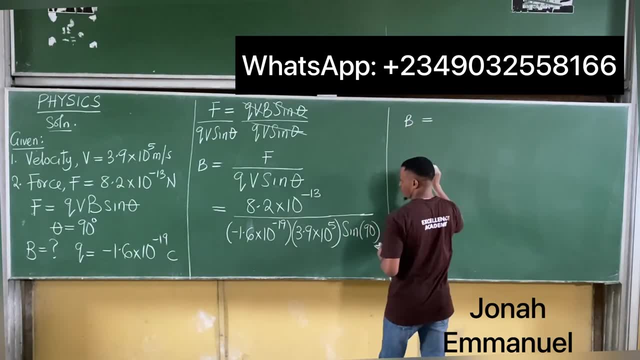 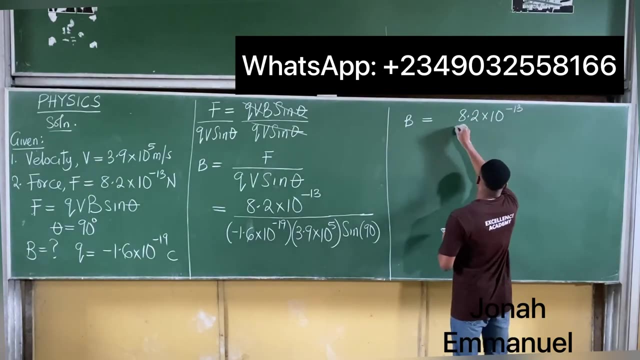 theta has to be 90, so that's the idea here. so from this it means that it means that from here b, v is equal to. I'm having 8.2 times 10 to the power minus 13, all over if I punch denominator. 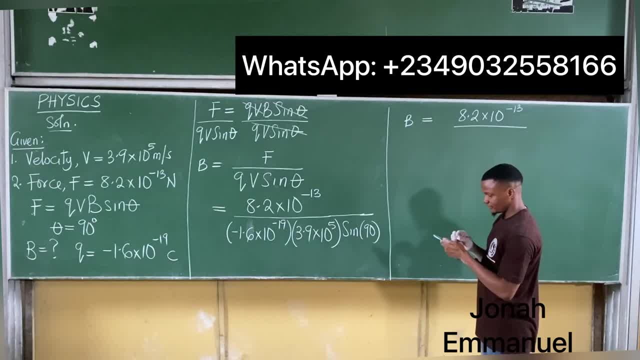 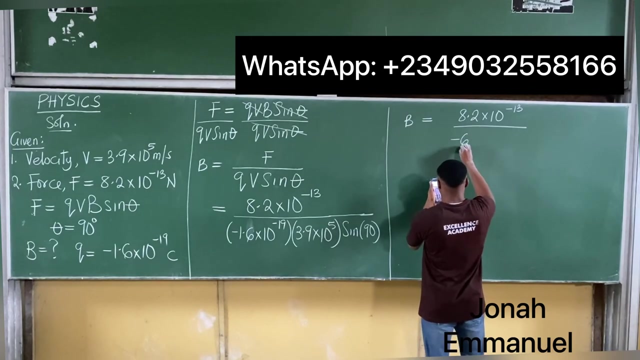 for denominator. I have minus 1.6 times 10 to the power minus 19, times 3.9, times 10 to the power 5, so I'm getting and that's about, that's about minus 6.4 times 10 to the power, minus 16,. 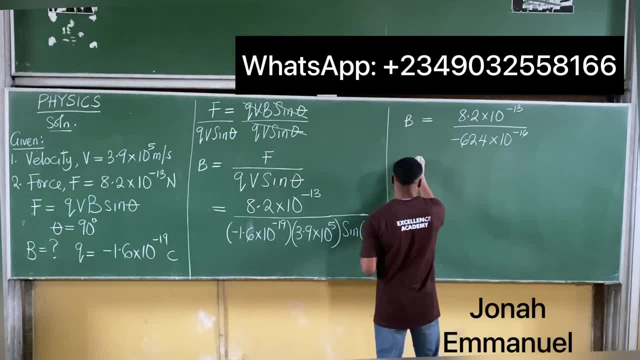 sine 9, so I have minus 16そう. I have this. that means v is equal. to divide this, I'm having 8.2 times 10 to the power minus 13, all over minus 6.4 times 10 to the power minus 19.. 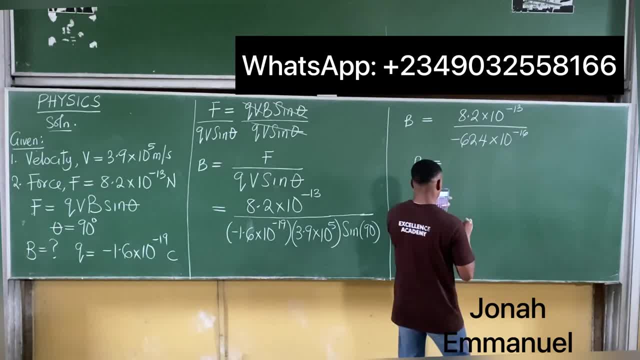 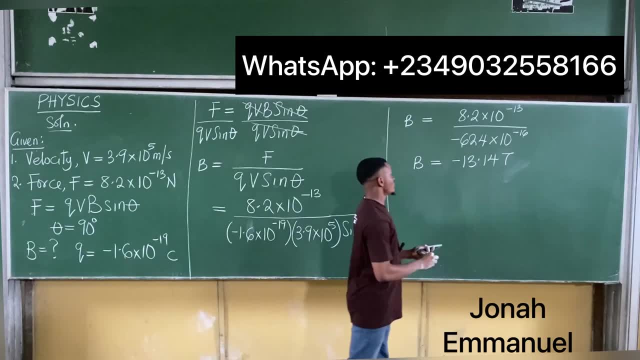 minus 16, that's about equal to minus 13.14 approximately in tesla. so b is equal to minus 13.14 tesla. now the thing is this, um, when you have a negative magnitude, usually when we get magnitude, we're expecting a positive answer. so this might be negative. now what you do is to this: 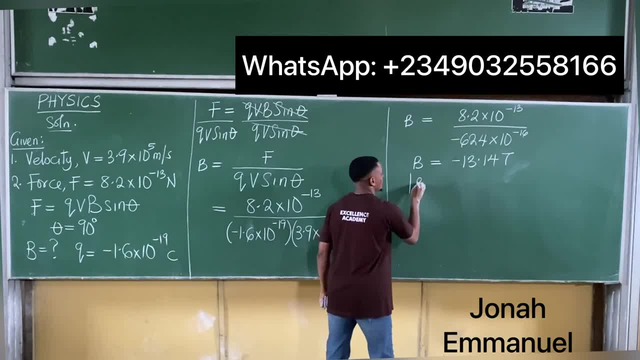 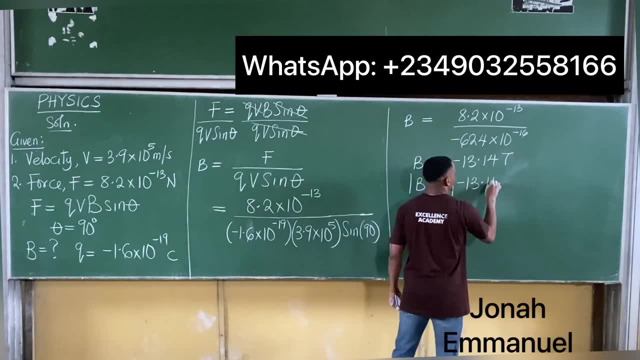 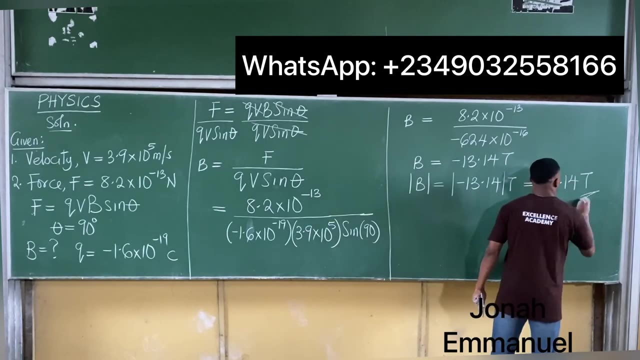 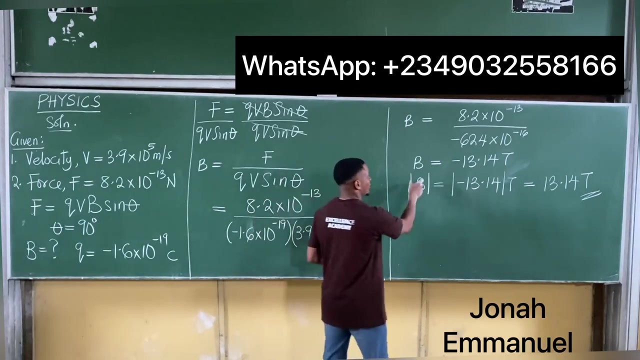 what you do is to take the absolute value, so the absolute value of the magnetic field will be equal. to take absolute value of 13.14 tesla, and that'll be equal to 13.14 tesla. so the same thing there, but we expect a positive result. that's the idea. so please, uh, when you're calculating for 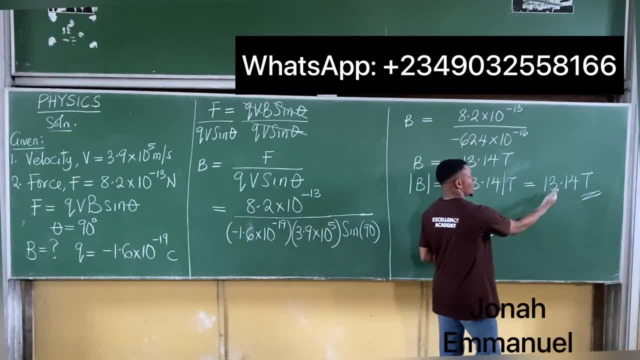 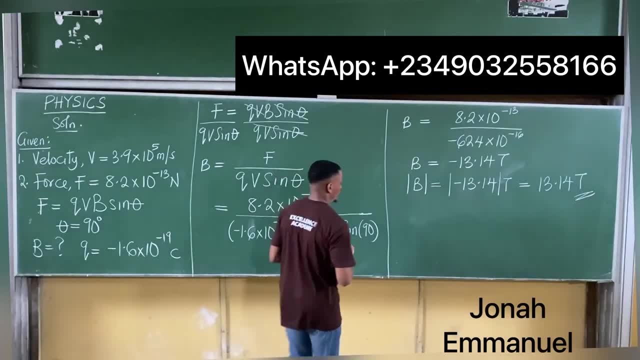 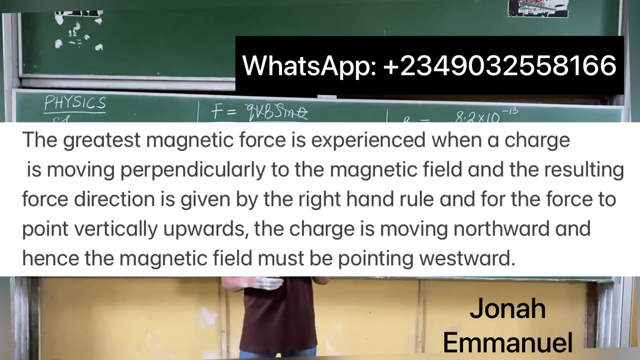 magnitude. you do this please. your magic value has to be a positive answer, so have this one here. so this is the magnitude of the magnetic field for the direction. for the direction, the answer would be westward, and the idea is this: the greatest magnetic force is experienced when a charge is moving. 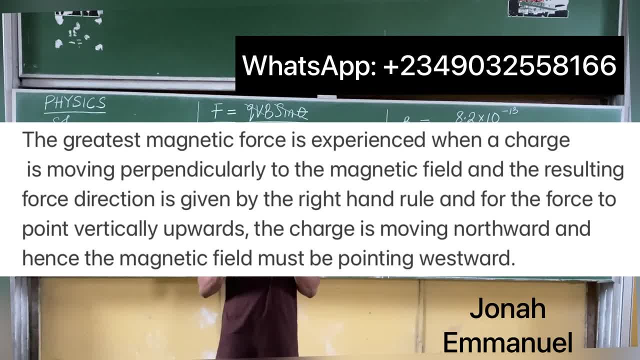 perpendicularly to the magnetic field and the resulting force. direction is given by the right-hand rule which we stated earlier, and for the force to point vertically upwards, the charge is moving northward. hence the magnetic field must be pointing westward. all right, so what we are saying is this: we are saying: 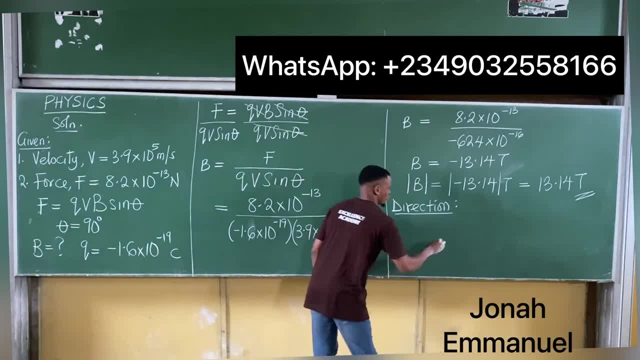 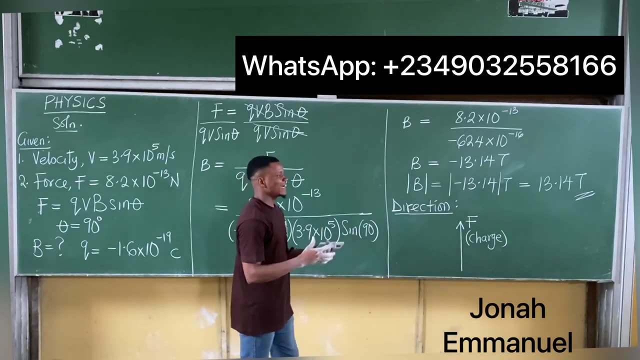 that if I have a force, if the force is going upwards or northwards, as you see in the equation, if the force is going upwards, that means the electric charge is also moving in the same direction. so that means the charge is moving northwards. and we said: for the maximum or the greatest force it must be. 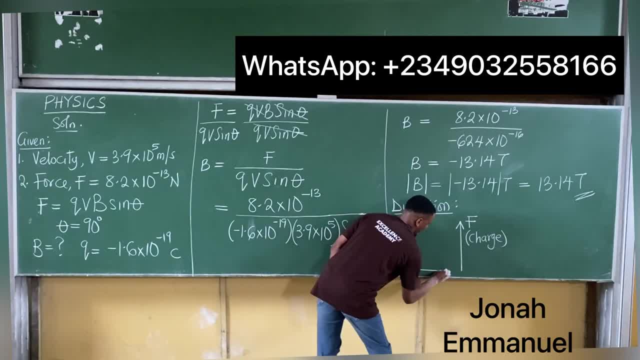 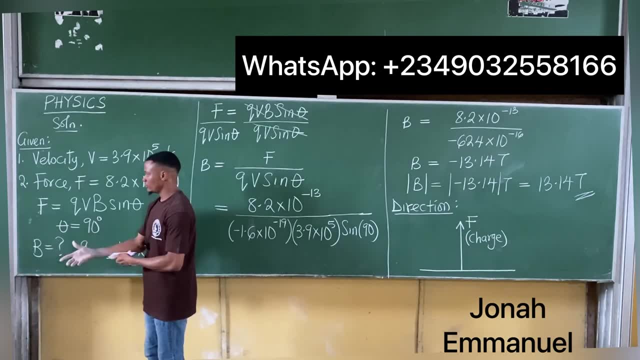 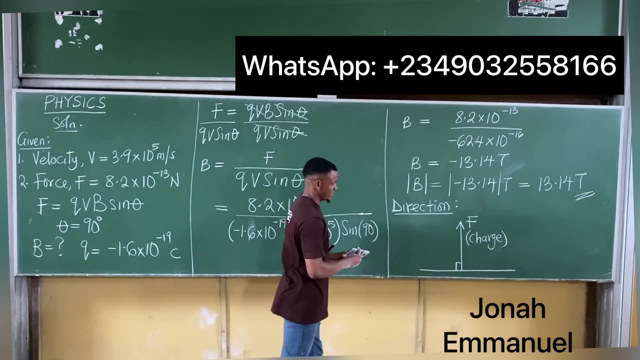 perpendicular, so I'll simply draw a perpendicular line to this. of course, the maximum force is experienced when the charge is perpendicular to the field. that's 90 degrees. that means I'll be having this way as my this. all right, so I have 90 degrees, so the, the magnetic field is now moving.